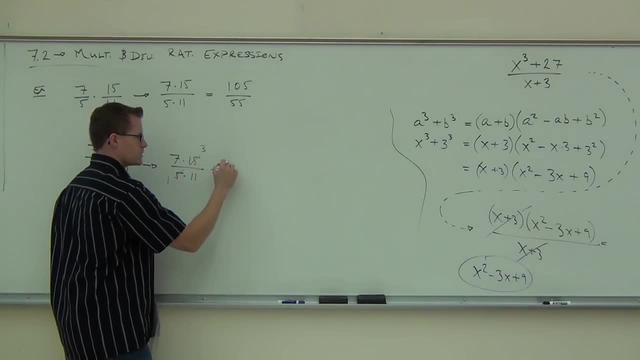 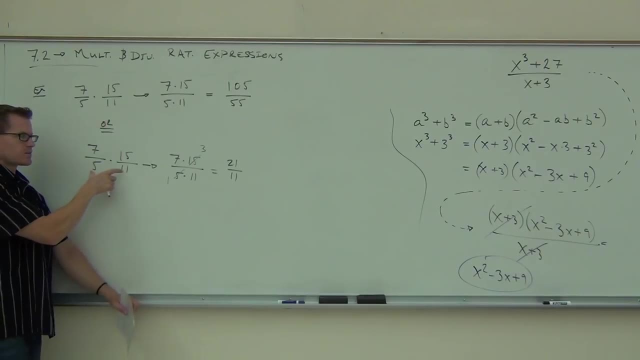 This is what you're used to, right? I hope Yes, And you do the 21 over 11,, which is a lot easier than doing that. But notice that the process here is, when you write two fractions being multiplied together as one fraction, you change it from a multiplication problem to a simplification problem. 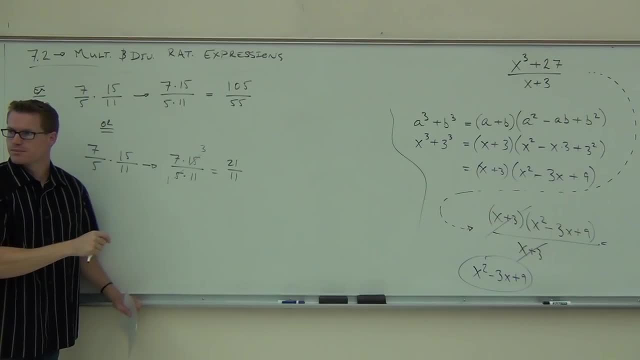 and then we're back to the 7.1 step there. So there's a whole bunch of stuff that we just finished doing. That's it. That's really it. We'll try a few kind of basic basic problems here, just to get our feet wet with this stuff. 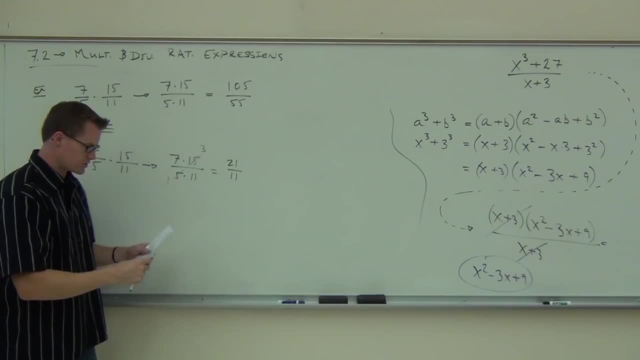 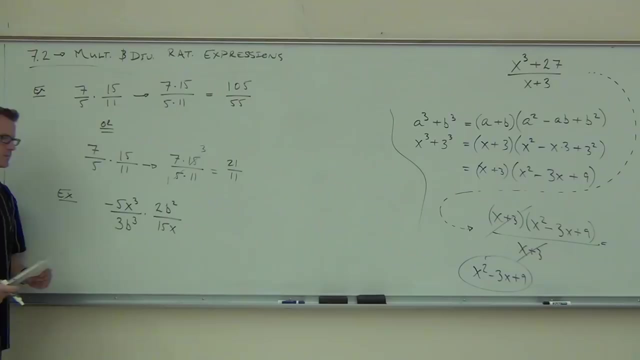 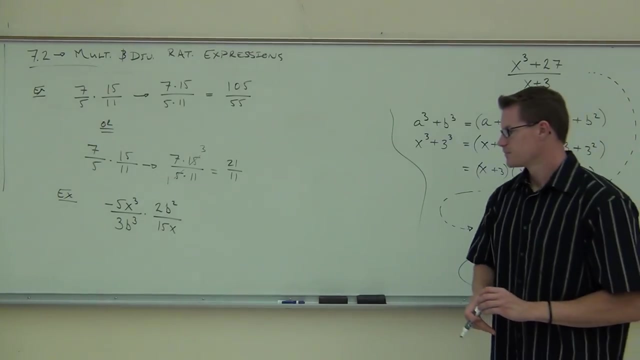 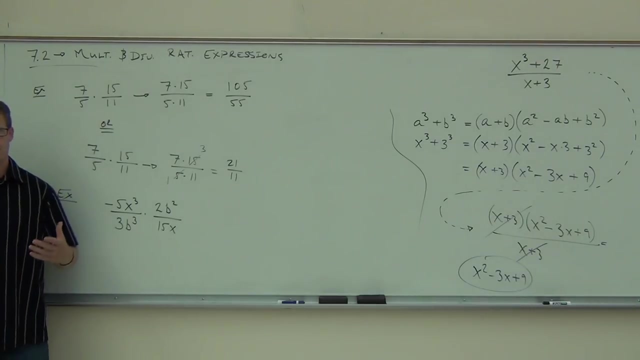 and then we'll deal with some some honest to goodness rational expressions and see how the problem shows. So just to kind of confirm what we're doing, can we do something like I want this one? Okay, first thing, notice we do have multiplication. they're fractions, they're rational expressions. 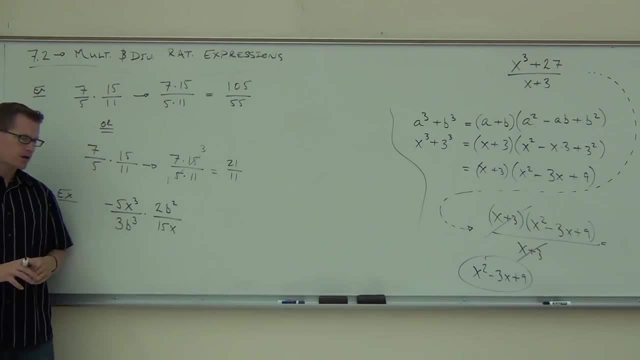 We only have one term on each numerator and denominator. though that's fine, We can still go about and multiply these together and simplify them. So here's what we're going to do. Here's a step I do need to see from you. 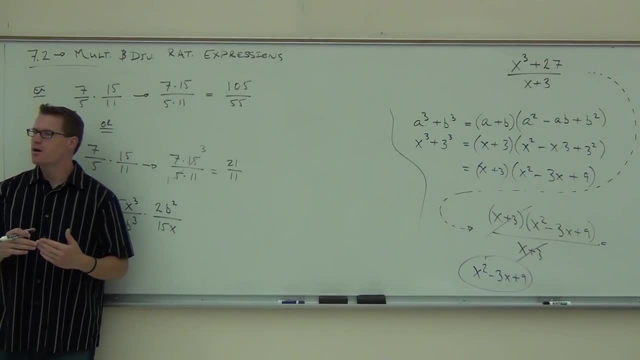 Are you listening back there? Step, I do need to see from you, I need to see somehow that you're making this into one fraction before you start simplifying them. This is for a couple reasons. First, I need to see that you know we multiply straight across. 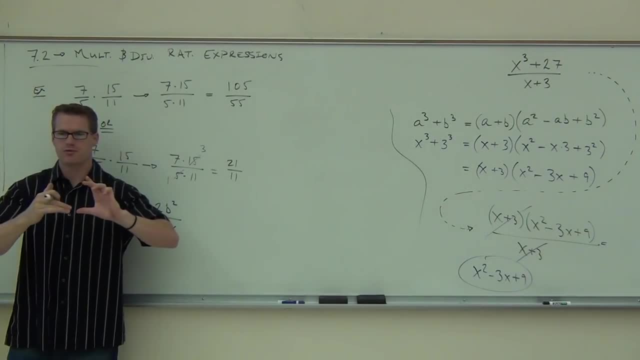 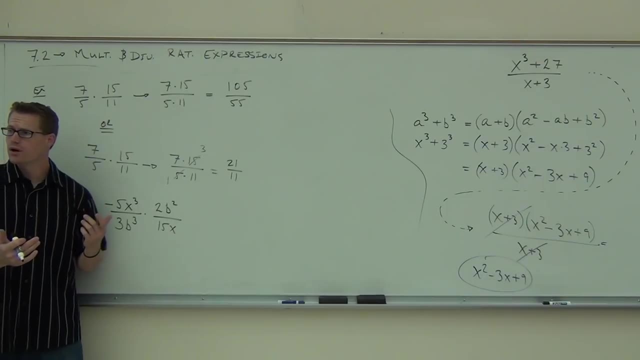 and we get one fraction on the top and the bottom numerator and denominator before we simplify. Second, I can't allow you to do this across like addition Or subtraction, because it just flat out doesn't work, And so if you can make this into one fraction, write this as one fraction. 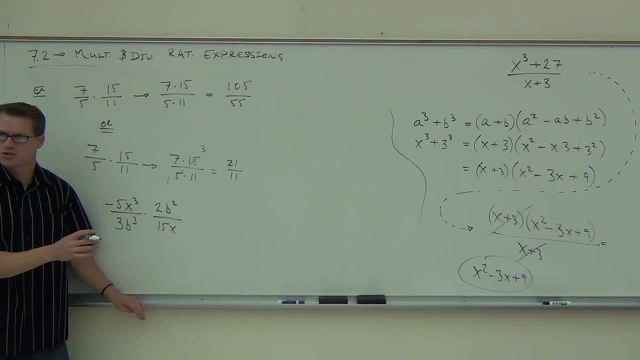 then I know you understand that I'm not going to be able to do this. on addition and subtraction: We can't simplify across addition and subtraction. Are you with me on this? So there's two ways you can do this. You can rewrite the problem like I'll be doing or, if you want, if you just don't feel like rewriting it. 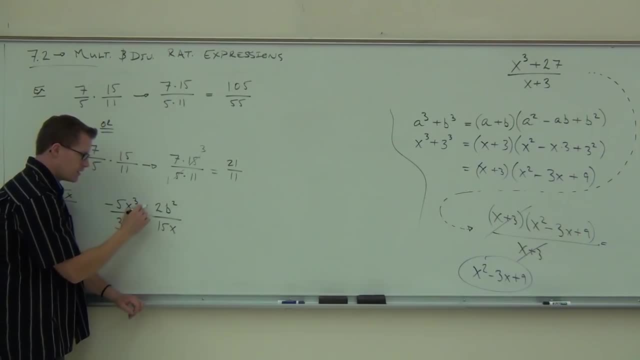 if you ever have multiplication, we can just extend that line and put the dot and the dot That makes this into one fraction. Just do this, Do this little piece before you actually simplify it. You okay with that? Just do that for me. 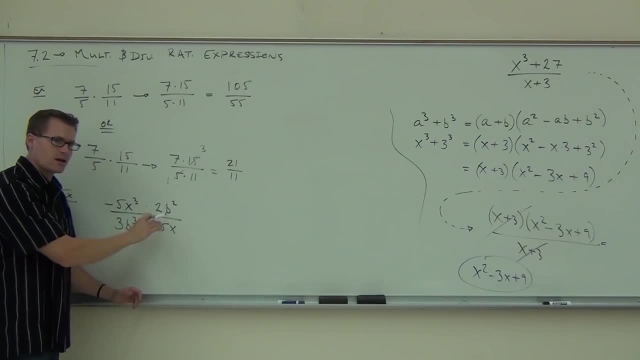 Make sure you have one fraction before you simplify it, because if you can't do that with addition or subtraction, you've got a problem. You can't simplify like we're about to, So I'll go back to what we were. You can just do the line, put the dot and the dot, if you'd like, on your paper. 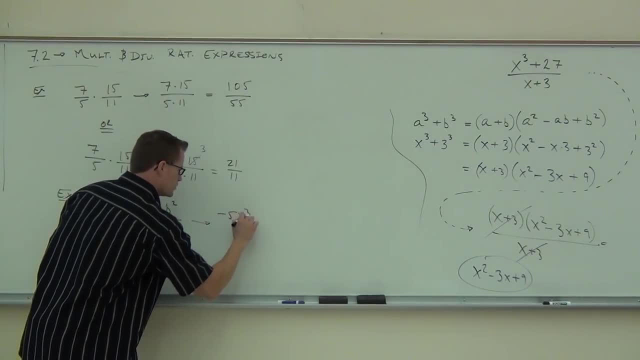 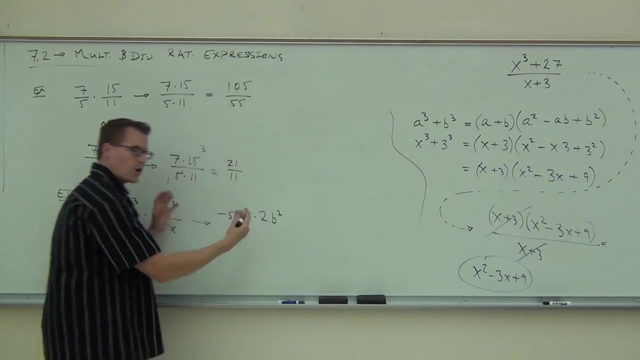 Me. I'm going to rewrite it: Negative 5x cubed. We know, with multiplication we multiply straight across, So this becomes negative 5x cubed times 2b squared. We're actually not going to multiply them together. We're not going to get negative 10x cubed, b squared. 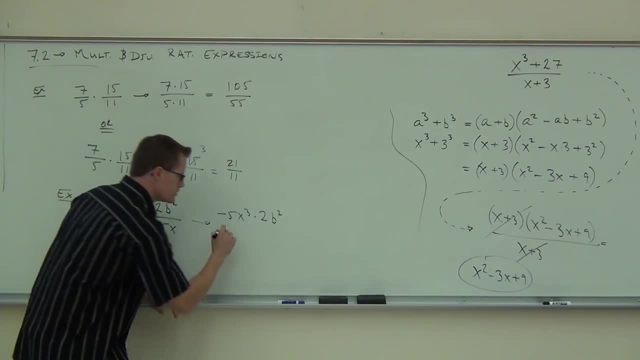 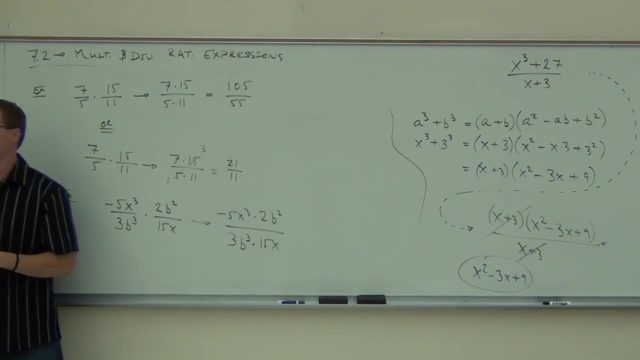 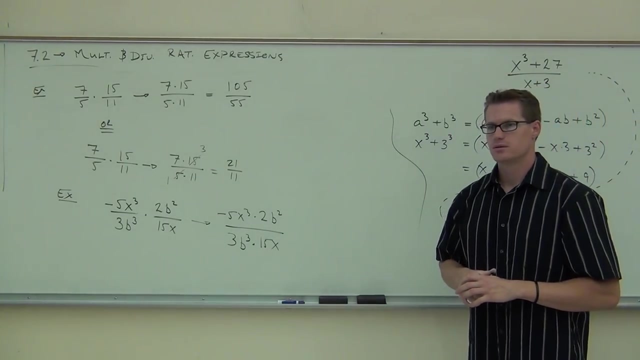 That's too much work. We want to simplify before we do that. So let's look at this problem. What I'd like to know from you is: do I have any common factors on the numerator and the denominator? Yes, Firstly, are you okay getting to this point? 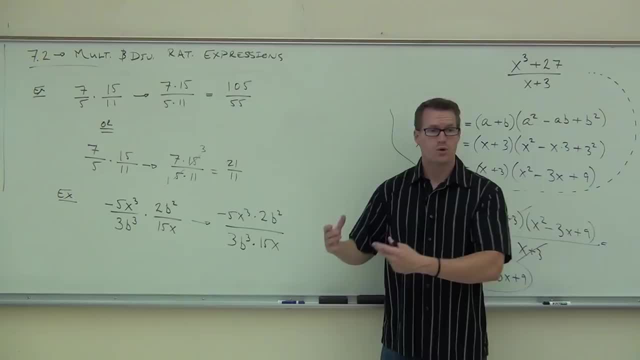 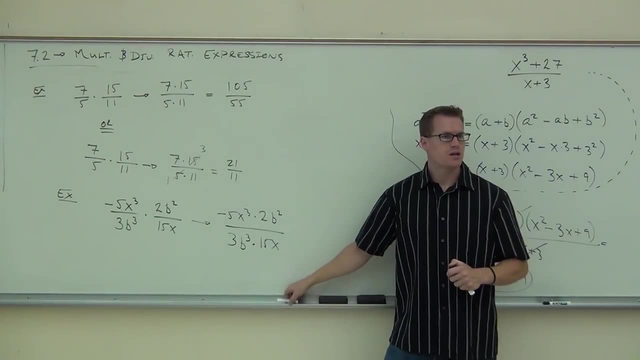 Multiplying fractions is straight across. We're right here right now. We haven't multiplied the numerator and the denominator. We haven't multiplied the numbers yet. We're right here right now. We're going to simplify now. What was the numbers you said? 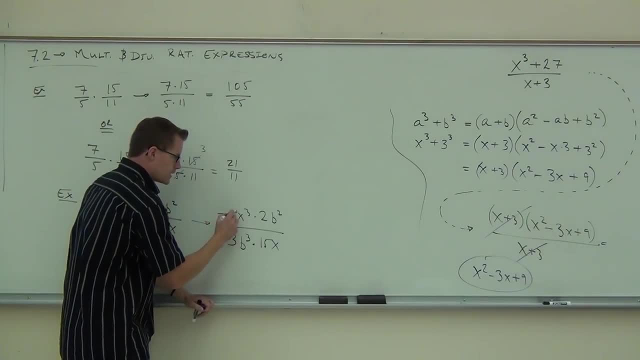 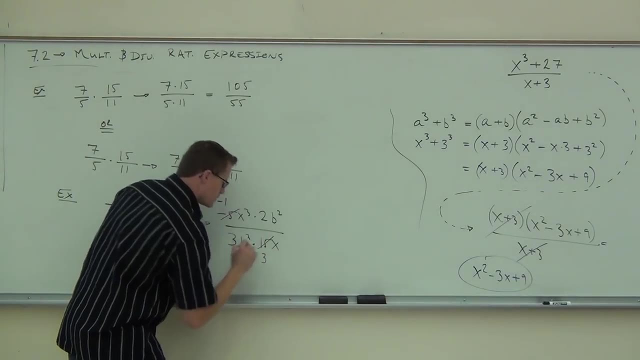 5.. So we're going to simplify like you would up here. The negative 5 becomes a what now? 1. Don't forget about the negative. And this 15 becomes 5.. And we're dividing by 5, remember. 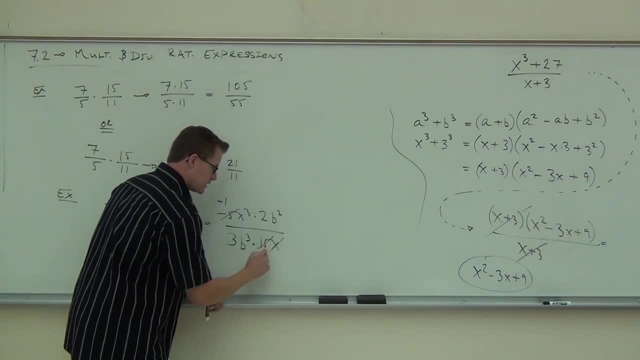 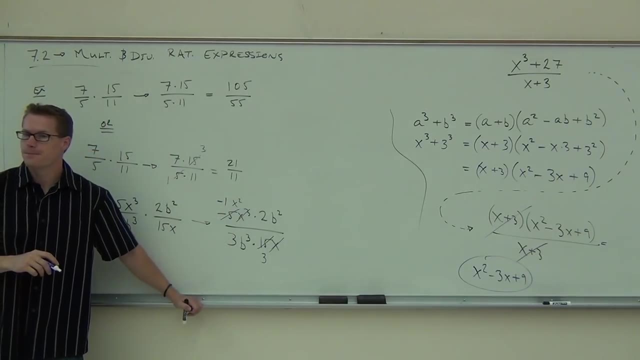 What else gets simplified? Oh, x is great. This x is completely gone. I'll write that up top, so I don't forget about it. Anything else. The b squared, So the b squared and the b cubed. What happens here? 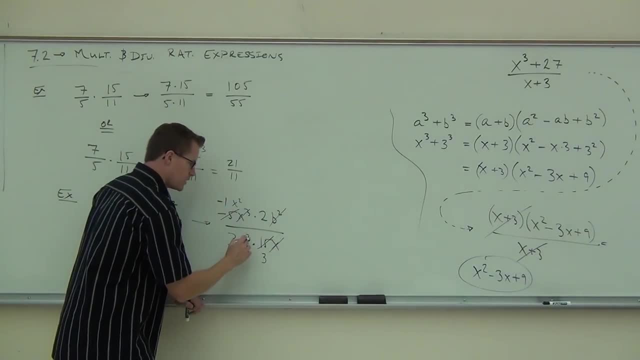 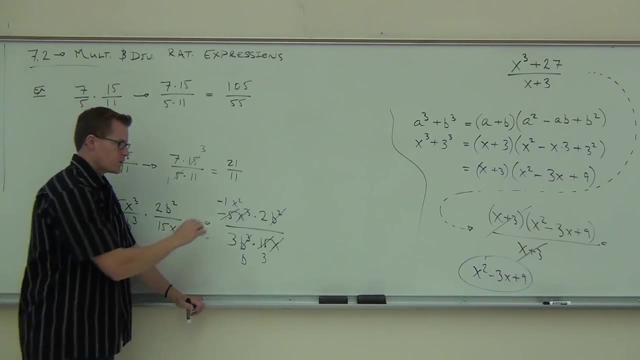 Gone And this becomes a what, Maybe? So I'll rewrite that. We just have to be careful not to lose anything in translation here. So we notice we have a negative, We've got an x squared And we have a 2.. 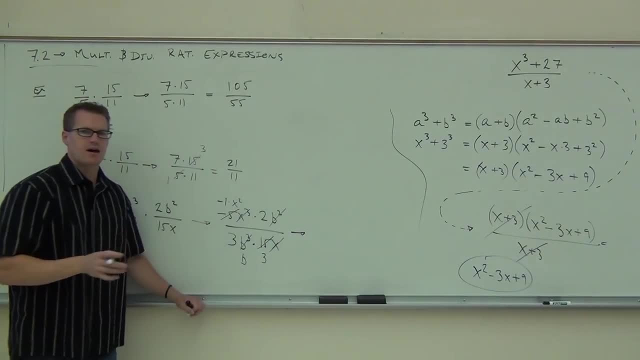 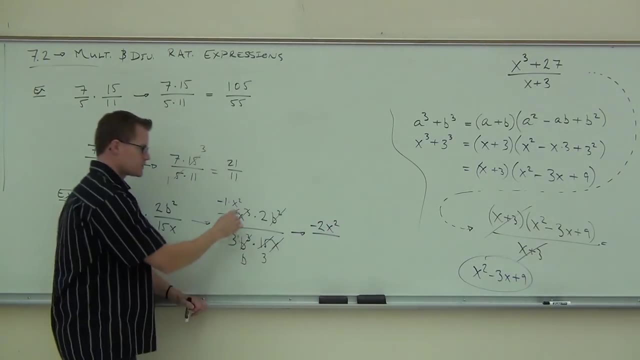 Don't forget about that. 2.. Can you tell me how much I'm going to have on the numerator? Negative 2.. Great, Perfect, That's exactly right. Negative 2, negative 2, x squared, It's all being multiplied. 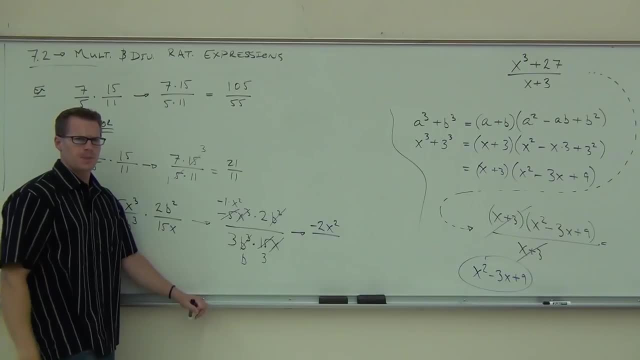 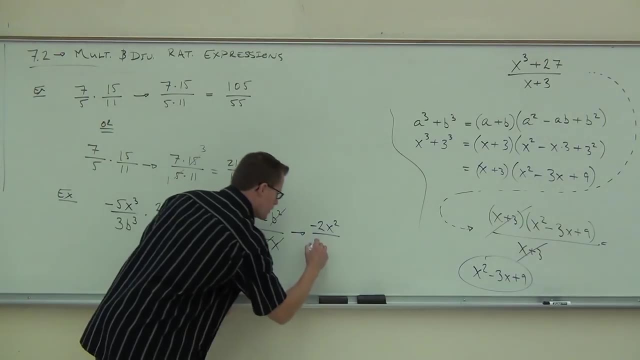 And on the denominator: how much did you get 9.. How did you get the 9?? Because 3 times 3.. So we don't forget about that 3.. We didn't cross that out, It's still there. 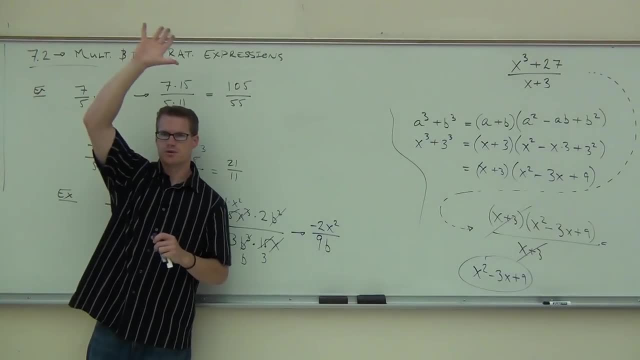 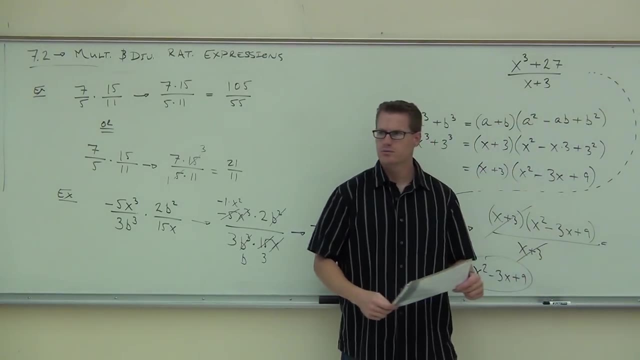 3 times 3 and then the b. You're exactly right. Would you raise your hand? if you're okay with this one, I feel alright with it. Would you like to try one of your own? Sure, We'll try two. 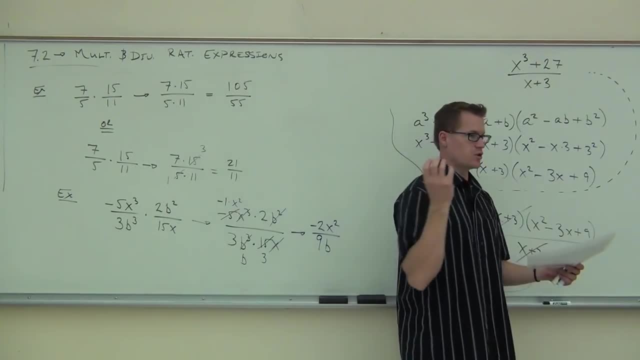 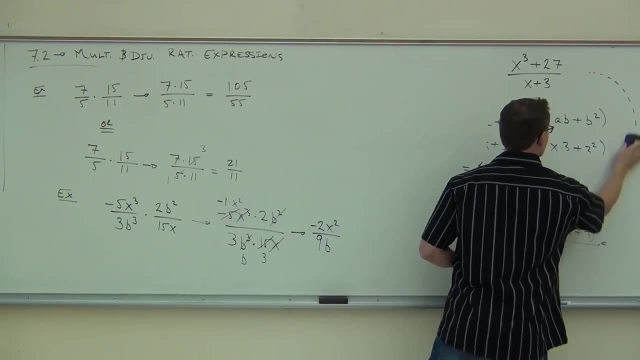 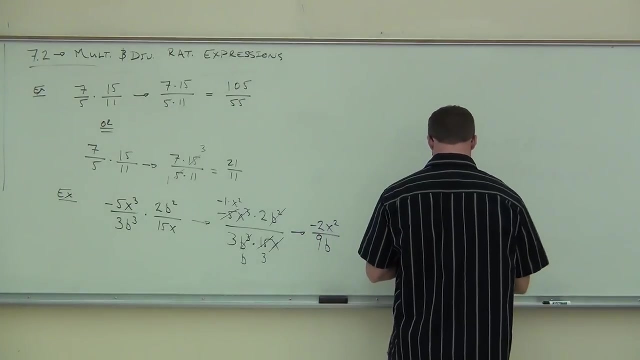 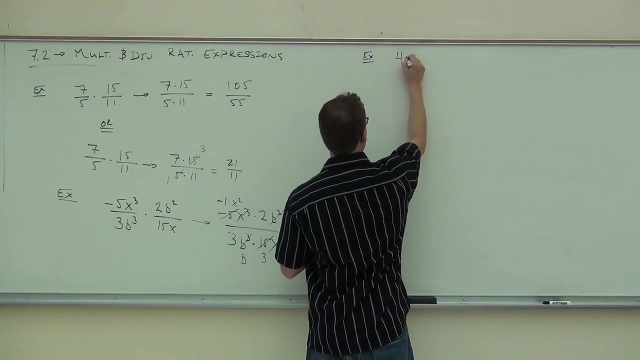 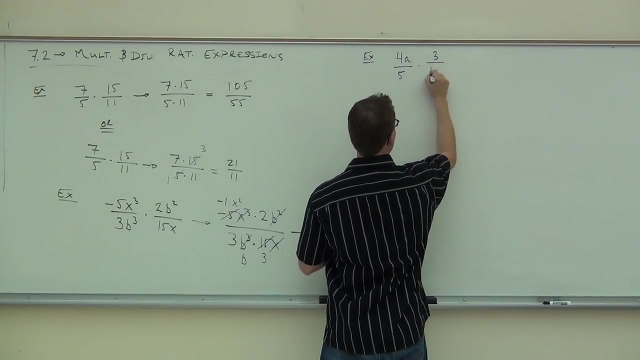 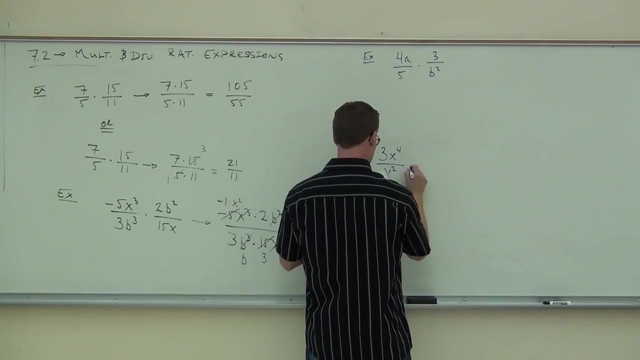 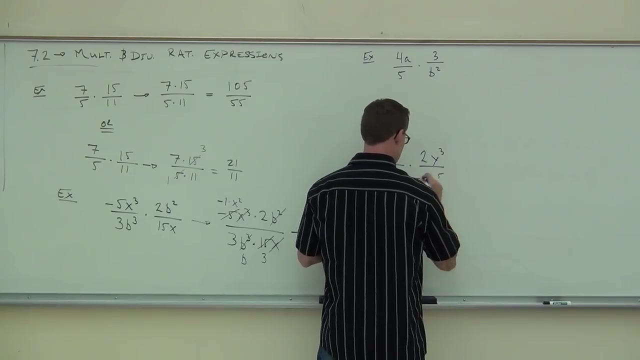 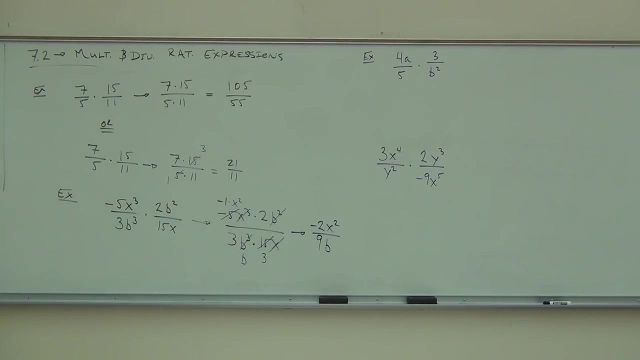 One you might not be able to simplify. I just want to make sure that you can do this. The second one you'll be able to simplify: There we are. There we are. So let's do this one on your own, Remember, what I'd like you to see from me is: 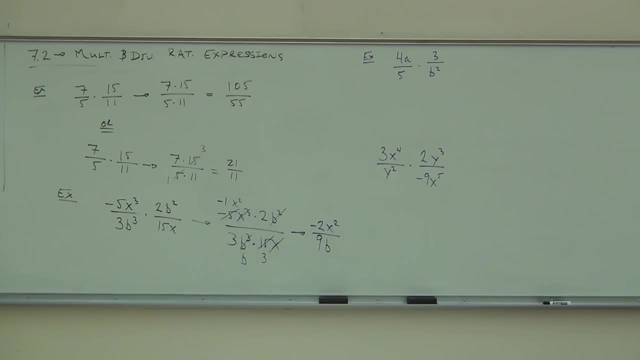 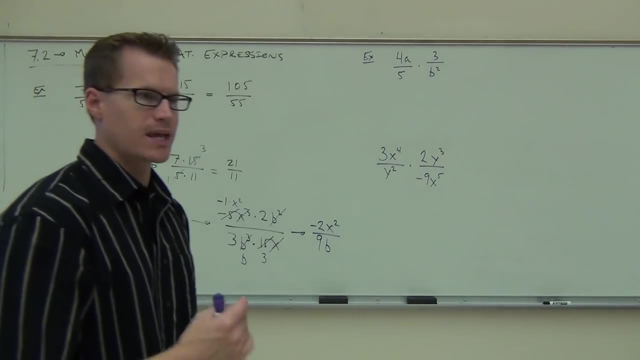 before you try to simplify or even multiply these things together, I want to see you write this as one fraction. So if you want to just extend that line, that's okay. That's fine with me, As long as we know that we can't simplify. 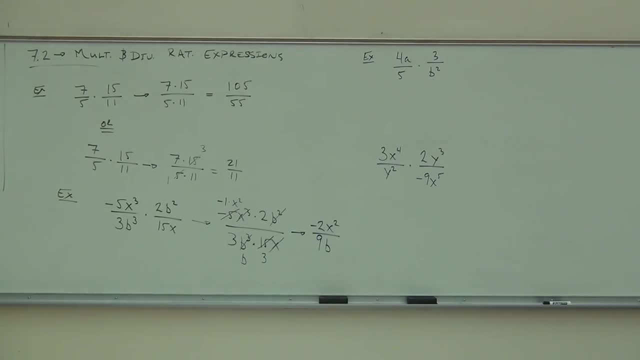 until we get this to be one fraction. That saves us a lot of headaches later. You can write down the number of times you've finished. You can kind of just add some more time to make this as one fraction. So I'm going to give you. 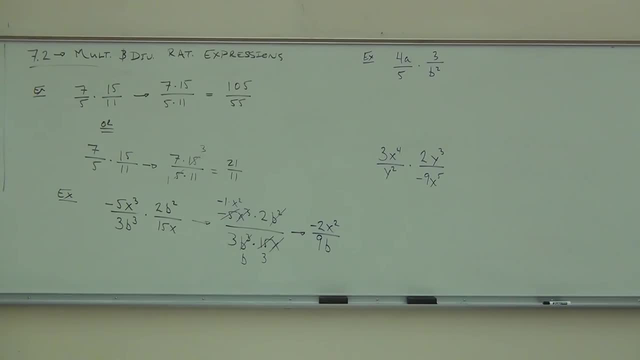 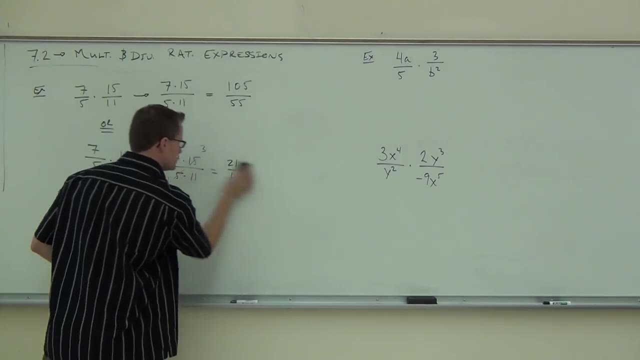 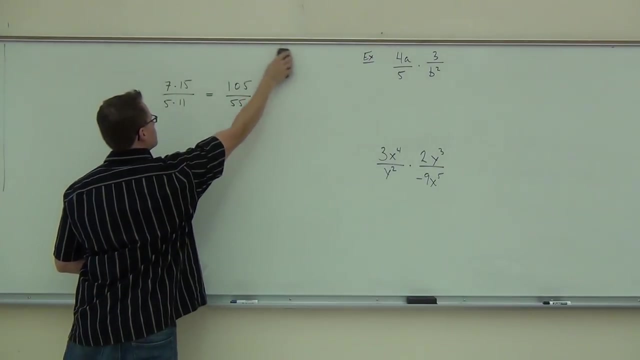 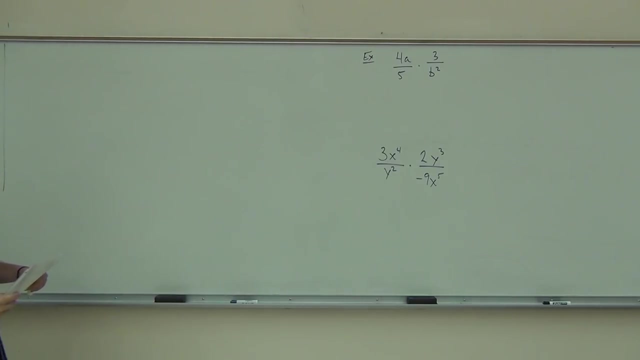 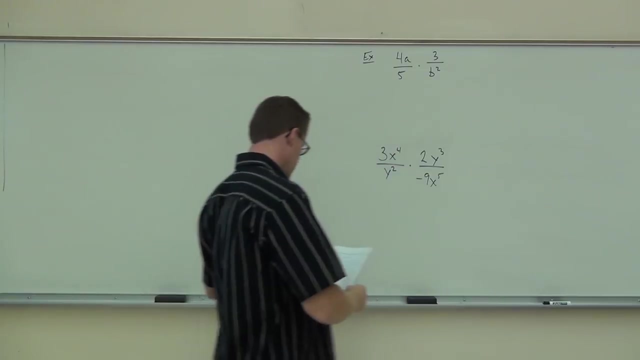 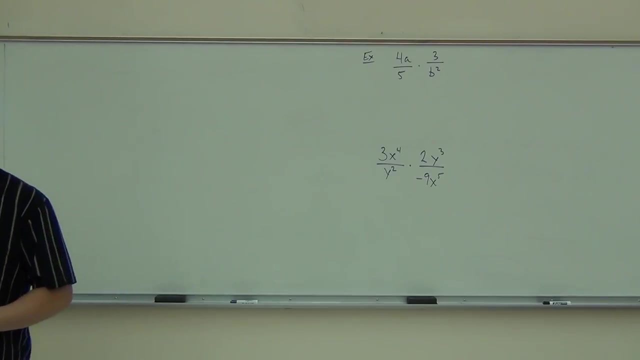 a couple of minutes to write down what you want to do, And then I want you to take your time, So I'll show you all of these you can do. Now Give me a little bit more time, give it 20 more seconds, so we can see if we can knock. 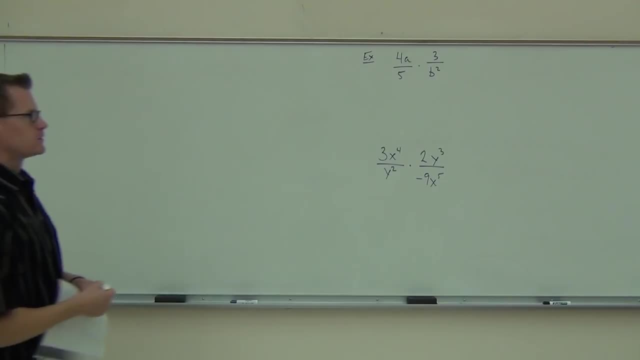 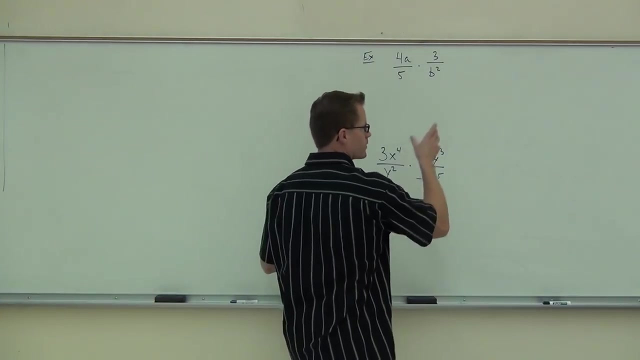 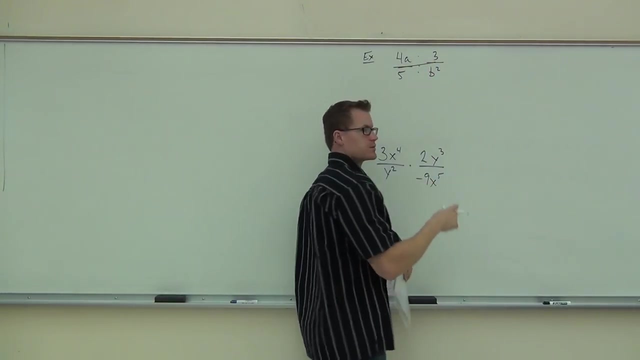 that out. Okay, here's what I'm talking about, about showing me the work. If you really want to do this, if you don't want to rewrite it, write this as one fraction, because we can do that with multiplication with a dot and a dot signifying that multiplication. 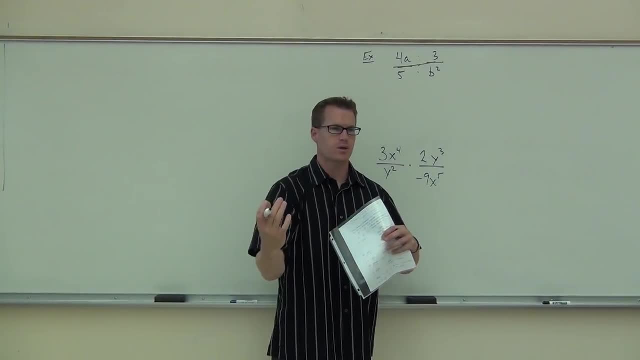 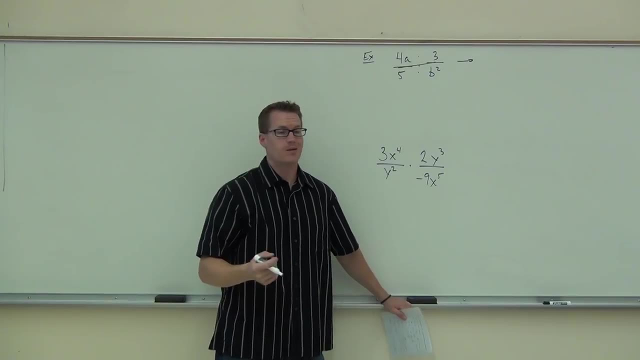 of two fractions is multiplication of numerators and denominators. That's fine with me. okay, you can do that. Then check for anything you can simplify. Is there anything to simplify in this problem? No, No, there's really not. 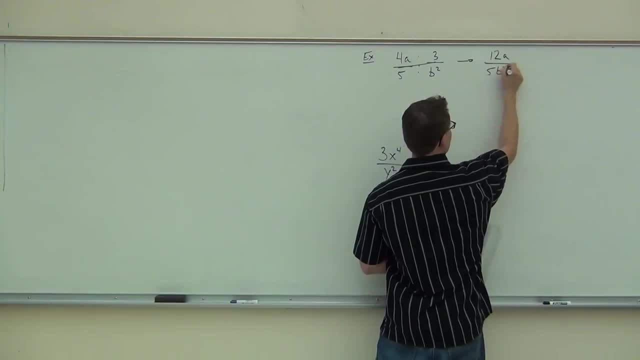 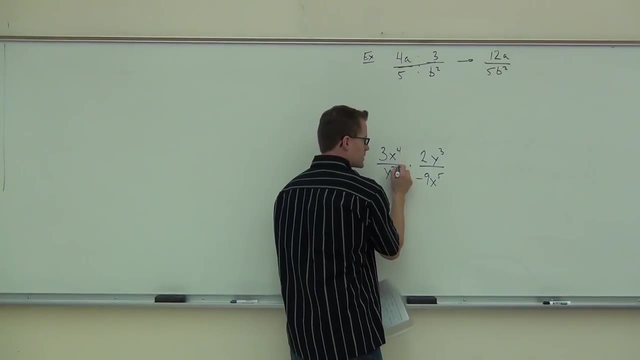 You can keep on going and say: this is 12a, this is 5b squared, and that's it. Sometimes you can't simplify anything. If there's no common factors, you're good, that's it. The next one same idea: we'll extend our fraction. 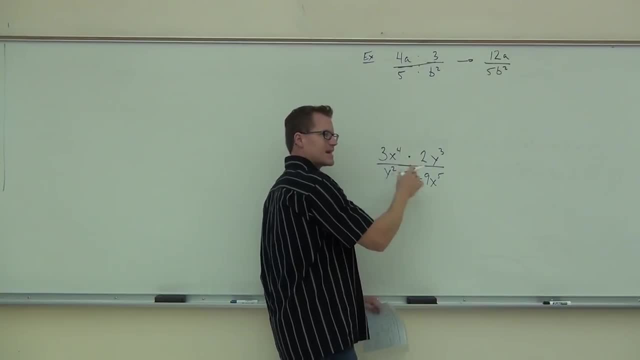 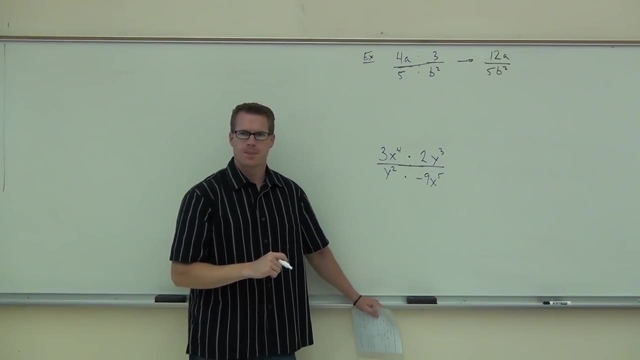 Did you do that? Yes, Put the dot and the dot. I want to see that because this shows me I understand. it has to be one fraction before I start crossing stuff out. Anything simplified here: The y squared- Okay, the y squared's gone. y cubed becomes a. 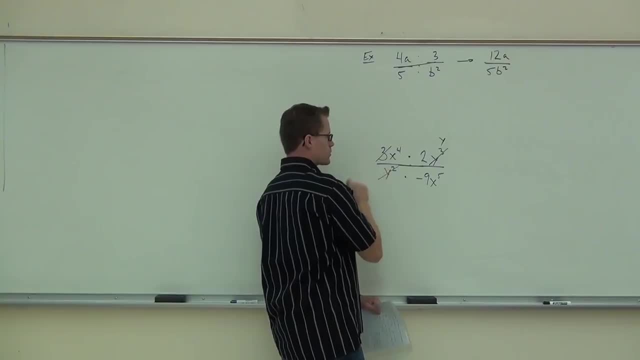 Y, Perfect, Anything else. The three and the x. The three is gone. that becomes a one, actually, and the negative nine becomes Negative three. Good, don't forget about the negative And the x. Ah right, we have x to the fourth and we have an x to the fifth. 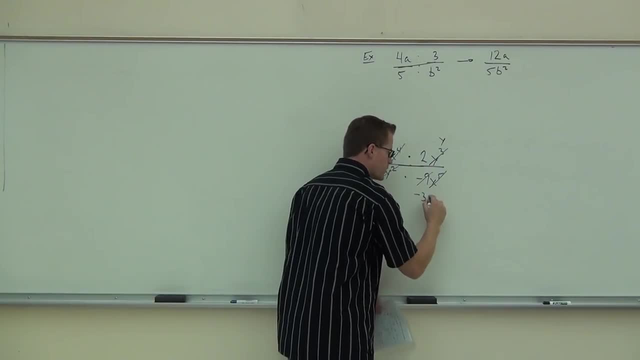 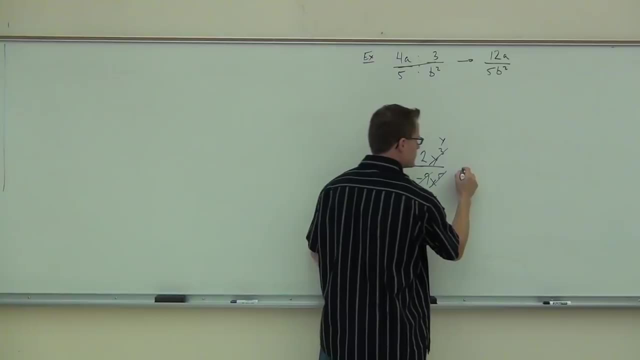 X to the fourth is completely gone, it becomes a one X to the fifth. we have one remaining x after we simplify that out. How many of you made it that far? Good, We write what's left over, write it nice and neat, like. 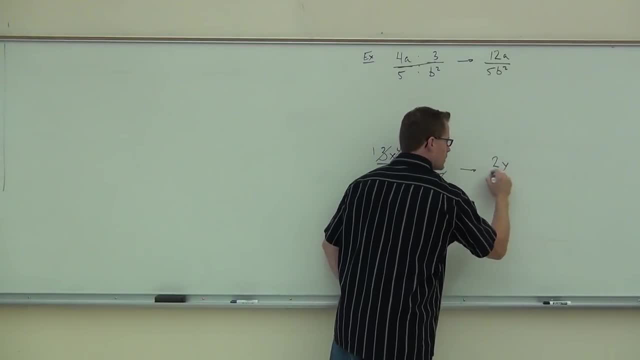 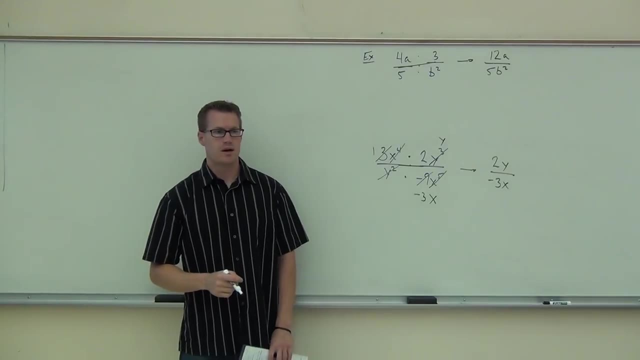 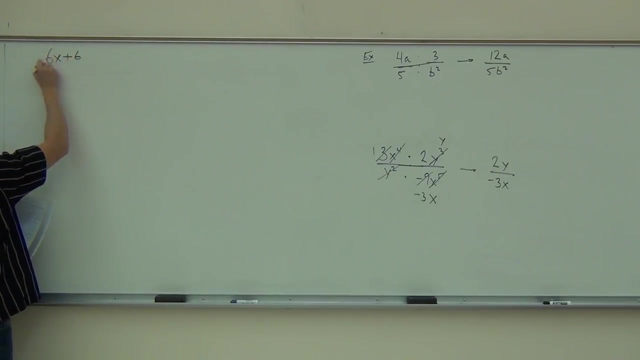 We've got one times two times y, so that's going to give us two y. We've got negative three times x. that's just negative three x. I believe that's our final answer, as good as we can do it. Now. there is one more that we can cover today that we're going to talk about. 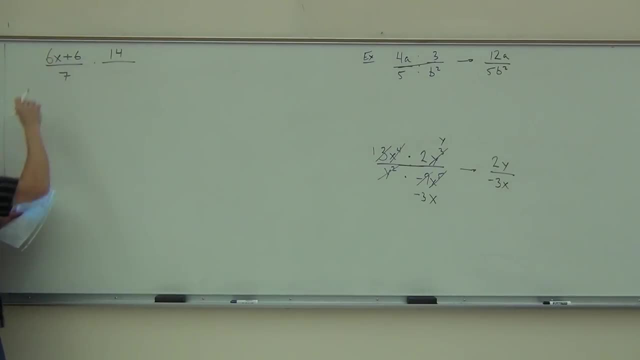 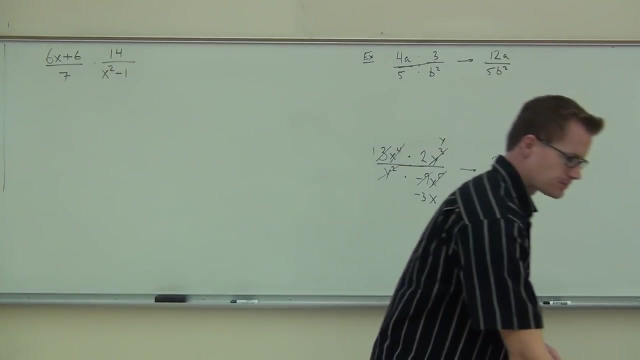 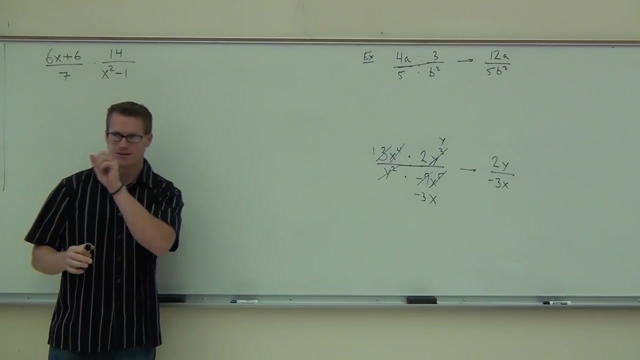 What happens when I start doing things like this? a rational expression times a rational expression Simplify. Well, guess what this is going to be? so similar simplification. it's not even funny. it's going to be almost the same thing. There's only one little extra step that we need to do. 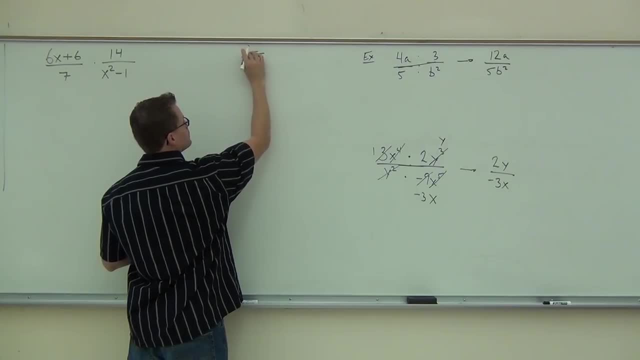 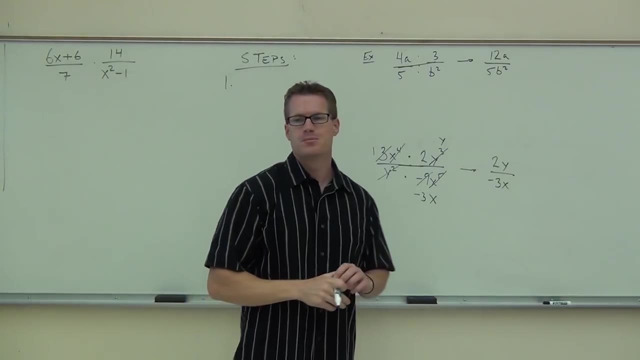 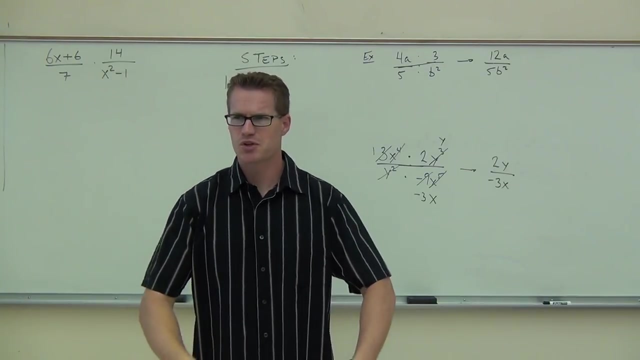 So here's our steps. for this First step, we're going to do pretty much. this happens almost almost every time you get rational expressions. What's the first thing you think we're going to do? What shoes are you wearing today? Factoring shoes. 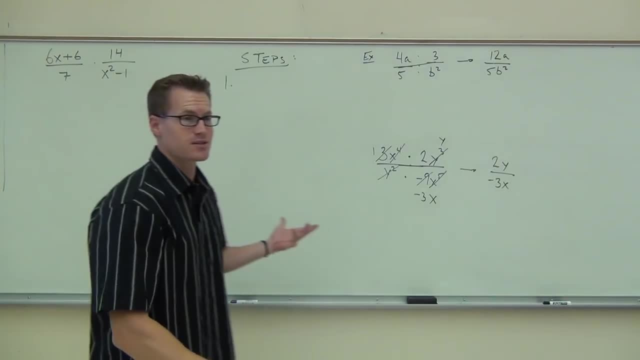 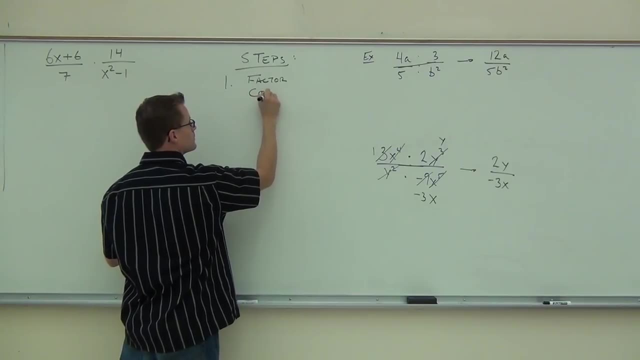 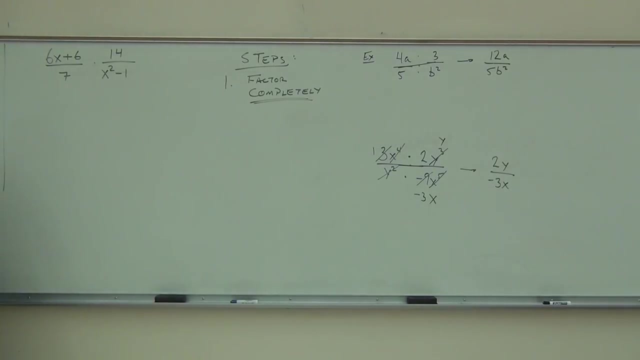 Factoring shoes. What are we going to do? Factor, You're going to factor, Yeah, you're going to factor this, Just like you did with simplification: Factor completely, Factor completely. Let's see if we can do that. just kind of do this quickly. we have a minute and ten. 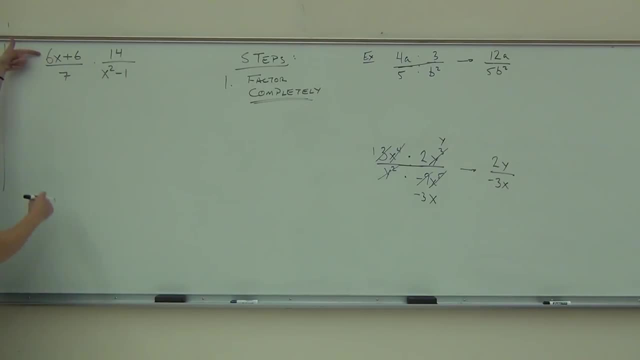 seconds to see if we can get this thing done. Does this factor, Yeah, What factors out of that Six And then x plus one, Perfect? Does the seven factor, No, No. Does the fourteen factor, No? Hey, are you starting to recognize what the x plus one is? 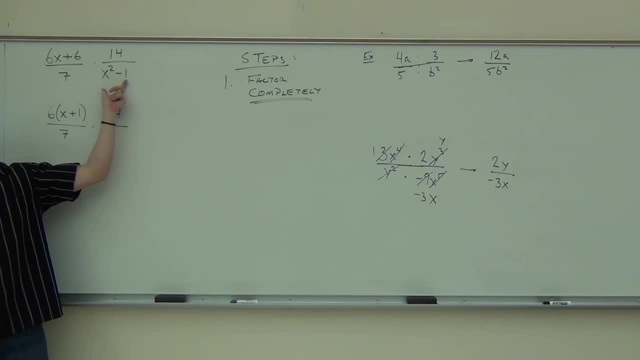 No, What is that? X plus one, x minus one. Good, Difference of squares. someone said over here: x minus one, x plus one. Are you starting to see the x minus one, x plus one pop up like that? Good, We factored this in fact. notice six. 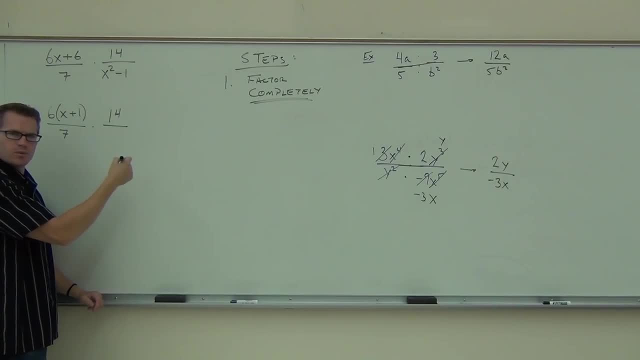 Seven and fourteen, we're good. X squared minus one. we've got to factor that difference of squares. remember this is x minus one squared. we can do x minus one, x plus one. we already did this today actually in this class. 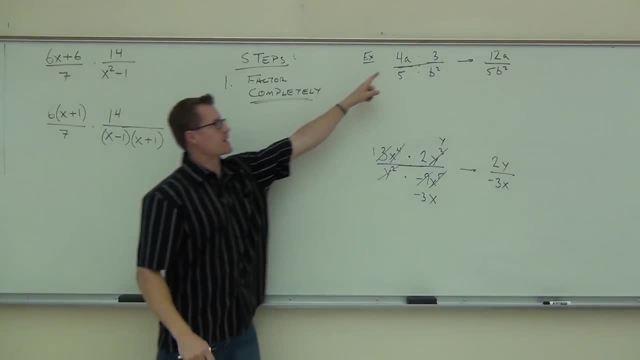 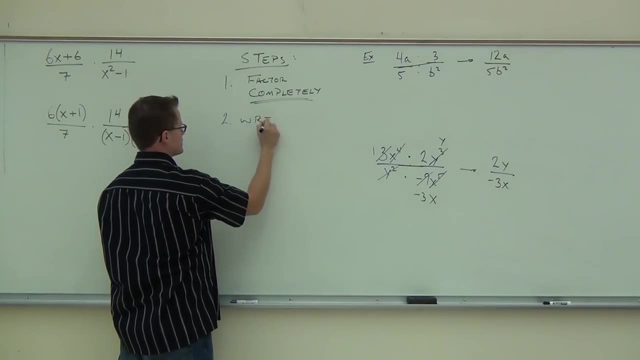 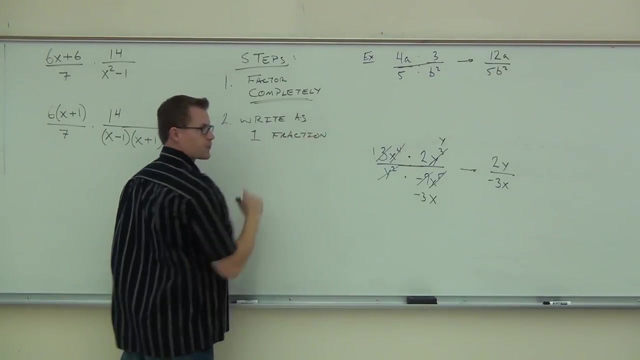 The next step is exactly what we did right here and right here, we're going to write this as one fraction. That's the easy. that's easy For us. that just means this: right here, folks, we're going to take this, we're going to extend. 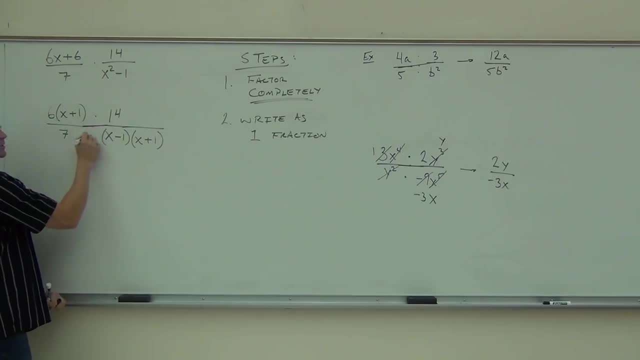 the line that makes it one fraction. put the dot dot and guess what? look at the board. Does this not look exactly like what we had in simplification? Yes, Because it is exactly what we had in simplification. The third step is simplify. 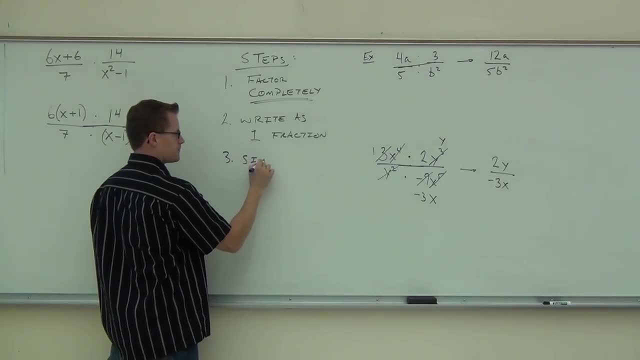 If we simplify, can you tell me some things that simplify here? X plus one Gone Seven and fourteen. Seven becomes a one, fourteen is a two. so on our numerator we have six times two, that's a two, That's a two. 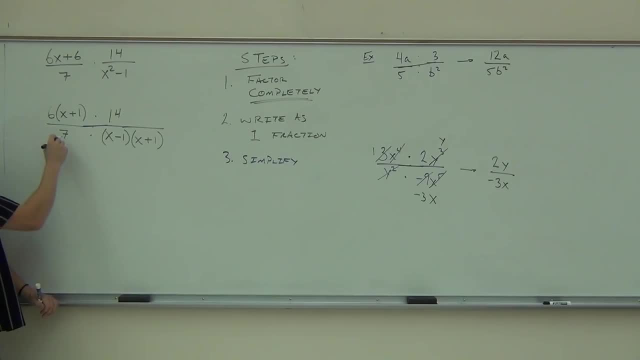 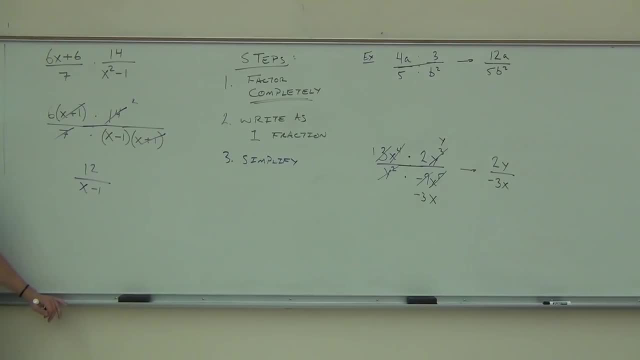 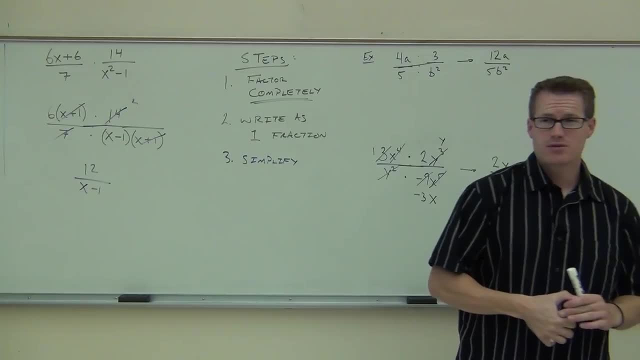 as well. I believe I gave you your homework for 7.1, didn't I? It's up on the internet. It's up on the internet. Okay, Have you made it to the internet yet to find that? Yes. 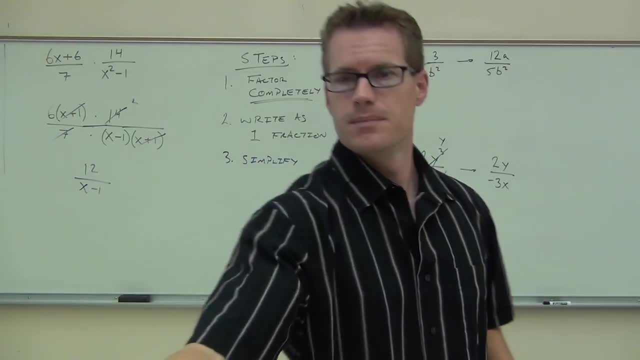 Alright, so we're continuing learning how to multiply and then we'll get to dividing some rational expressions. Today we'll continue with a couple more multiplications. We're going to do a little bit of multiplication. We're going to do a little bit of multiplication. 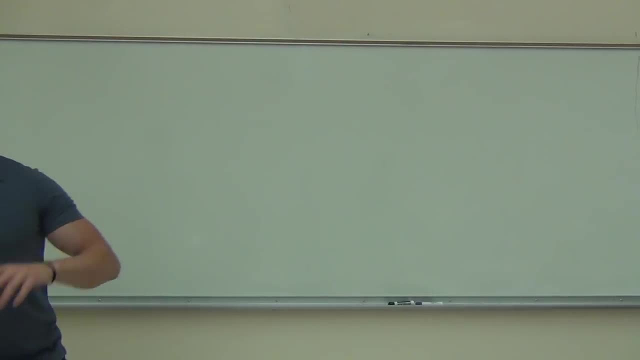 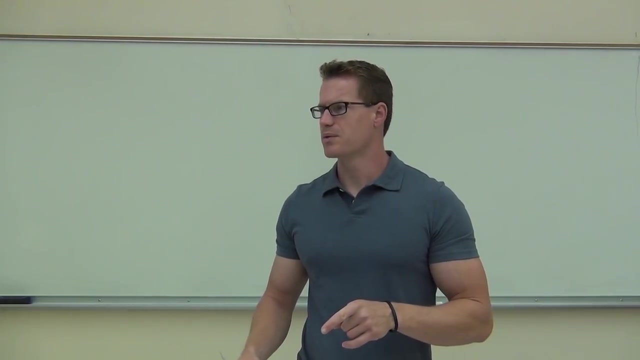 Alright, so we're continuing learning how to multiply and then we'll get to dividing some rational expressions. Today we'll continue with a couple more multiplying. The last one I gave you was the one with some steps on that right, I gave you the steps as well. 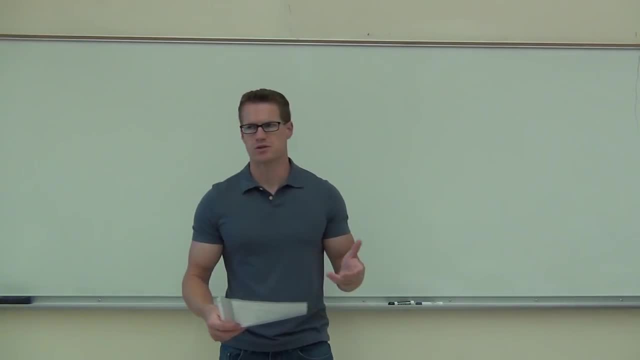 The first thing I want you to do when we're multiplying some rational expressions is we need to factor these things completely out. The reason why is because we're going to be simplifying using common factors, so we can't do that unless we actually factor it. 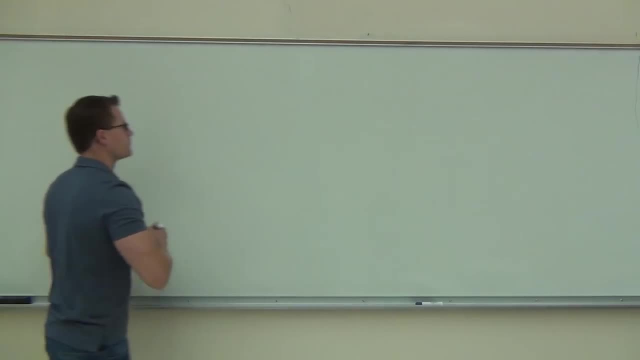 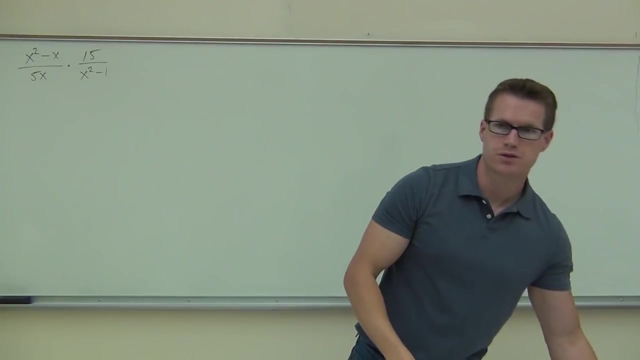 So let's go ahead and try this on this one, this next example. Now we'll see what to do about this Now. I gave you a few steps Last time. we're going to follow those pretty much to the letter every time we do a multiplication of rational expressions. That's the best way to do it. 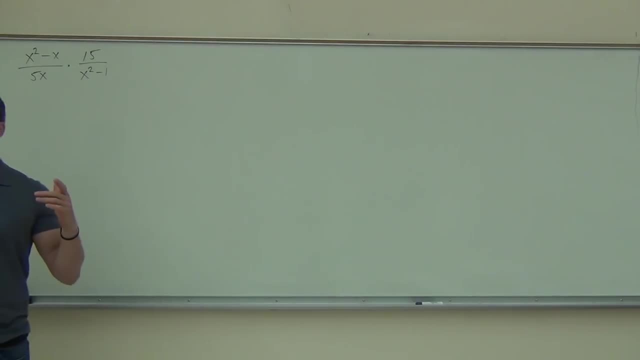 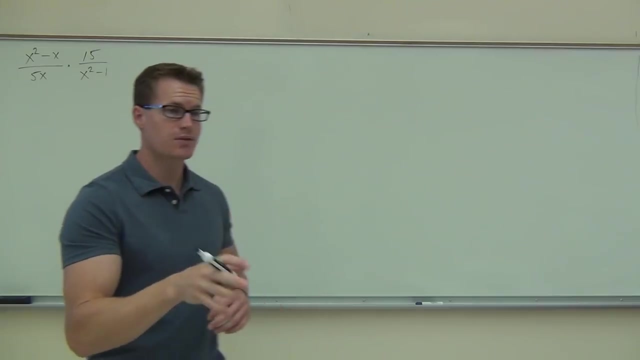 So the very first thing we get to do is we look at this thing and we are going to: what was that? again, Yeah, we've got to factor completely, Because, again, we're going to be looking for common factors eventually. So let's look at this thing together. 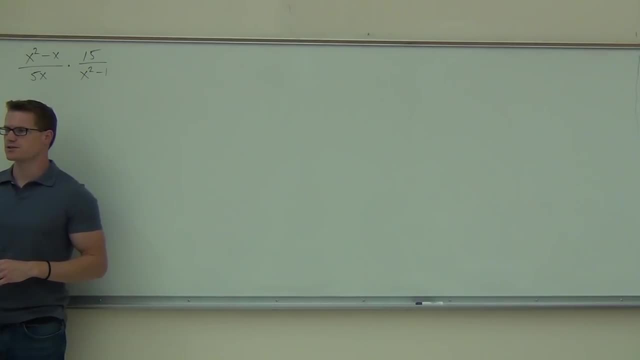 Can you tell me something up here that you're going to be able to factor? Okay, factor out first before we start simplifying. Factor out, so Okay. so x squared minus one, we can factor that thing. What's that called? people on the left-hand side of the room. this particular term. X squared minus one, we can factor that thing. What's that called? people on the left-hand side of the room, this particular term? Okay, so what's that called? people on the left-hand side of the room, this particular term? 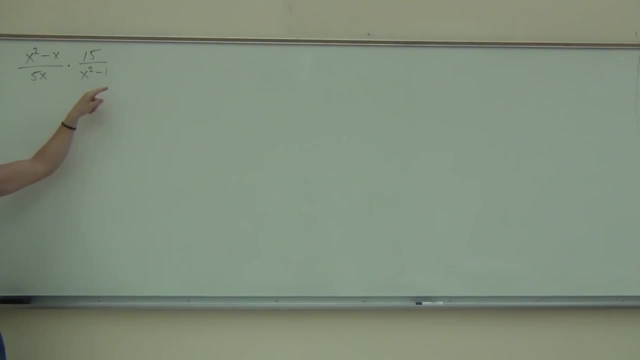 What type of expression is What term Different? on the square? We'll have a square, something We have a difference of a square. Are you guys awake today? That's a legend. All right, let's wake it up, Come on. 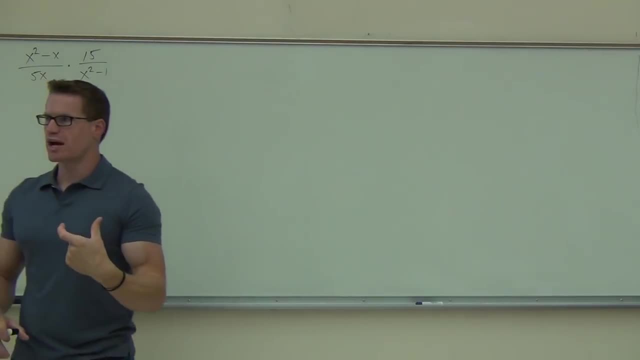 Yeah, that's a difference of squares. You need to be seeing that. Yeah, that's a difference of squares. You need to be seeing that It's a difference because it has a subtraction. It's two squares there. We've actually factored that one at least twice in this class already. 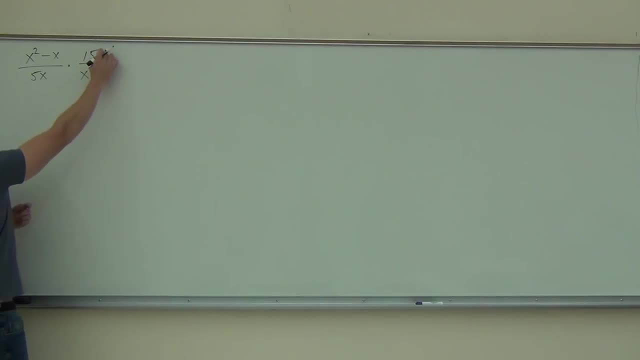 We need to be very good at seeing this We're going to: how about the 15,? can I factor the 15?? No, How about the 5x? can I factor the 5x? No, Those are there. those are just single terms. 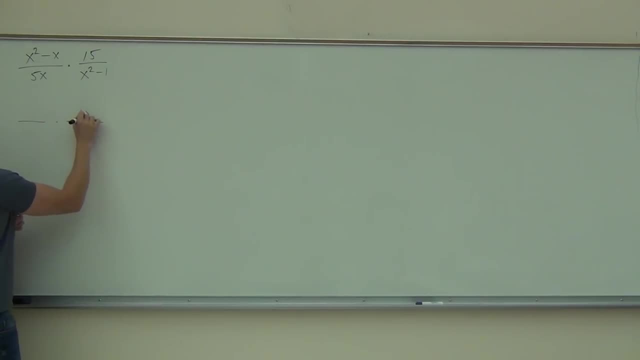 you can't factor single terms- X squared minus one- though that is something we can factor. Someone in the middle of the classroom tell me how I factor x squared minus one, please. X minus one, x plus one, Very good. 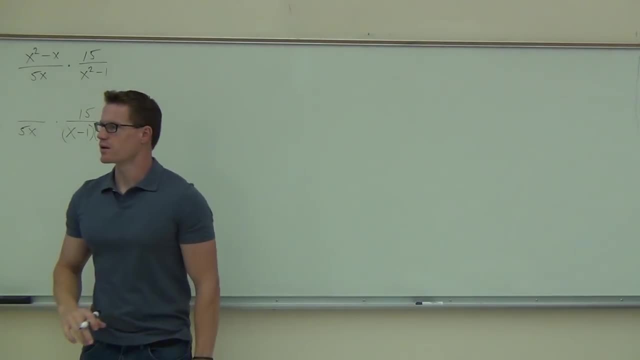 That's the difference of squares. gotta be bam, just getting those right all the time. Are you okay on getting x minus one? x plus one? See where that's coming from. Good, all right, we've covered that a few times in here now. 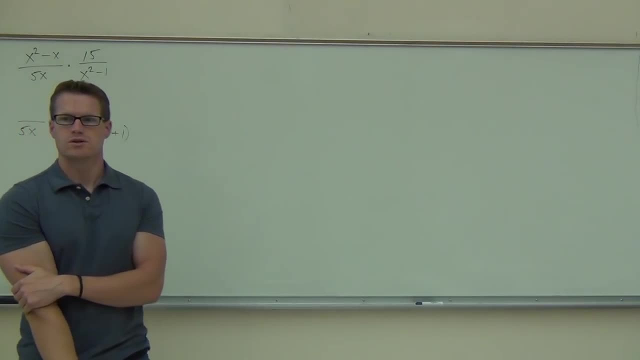 Now, how about anything else up here? what else factors Great x, squared minus x, what factors out of that? So remember, even though it looks like two terms, like that's not a difference of squares- how much does it factor that? 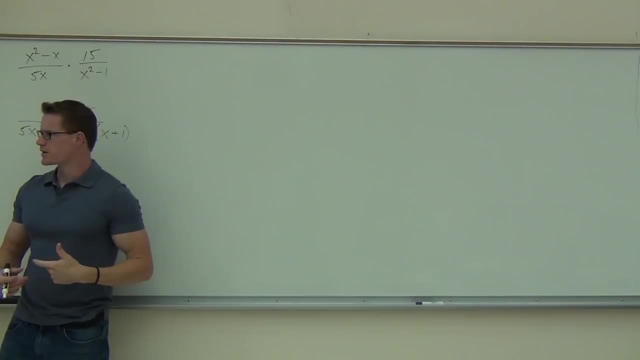 We always start factoring with GCF, that greatest common factor, and when you look at x squared, x squared minus x, well, they share an x in common, so we're gonna factor that out. So factor out an x. what are we left with? 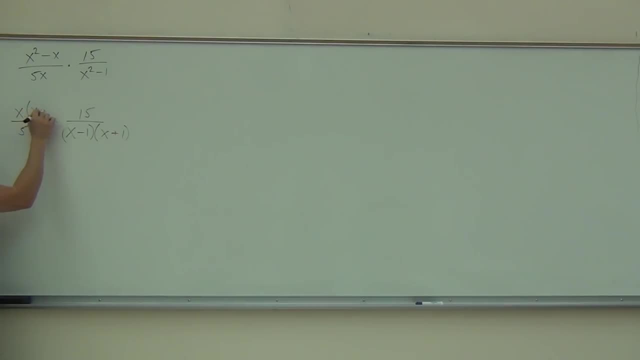 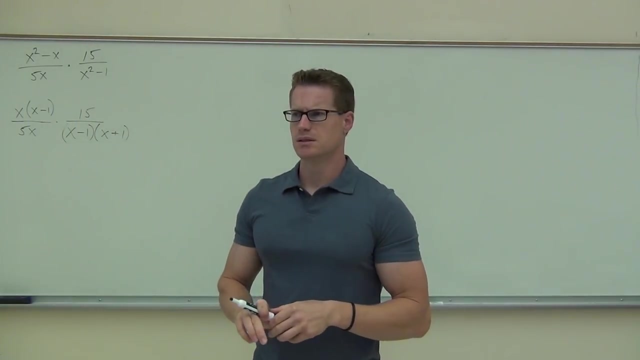 if we factor out the x, X minus one- Okay, You all can't factor in things like that- Good, so no diamond problems here. that's really not a big deal. The next thing we do is after we factor: what am I making you do before we do anything else? 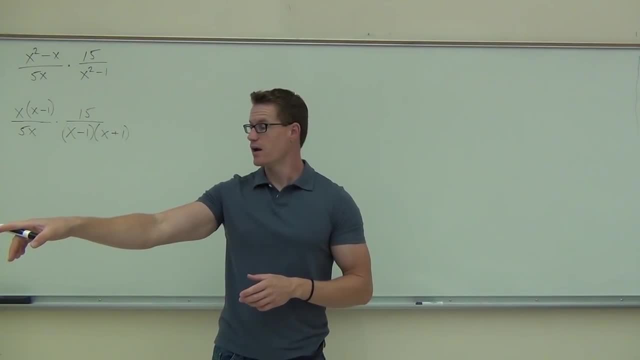 Say that louder: Right as one fraction? Yeah, we have to, because what we're doing here is we're changing after we factor, we're changing a multiplication problem into a simplification problem, and the only thing that we have to do to show that. 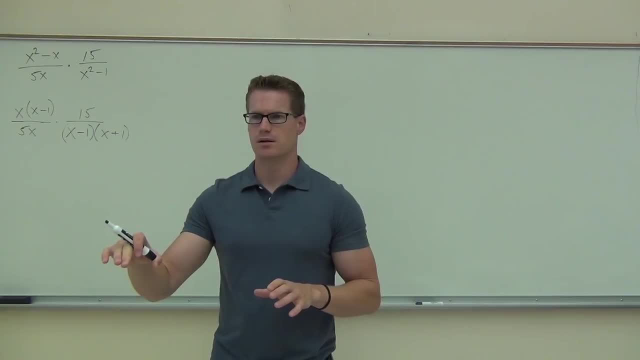 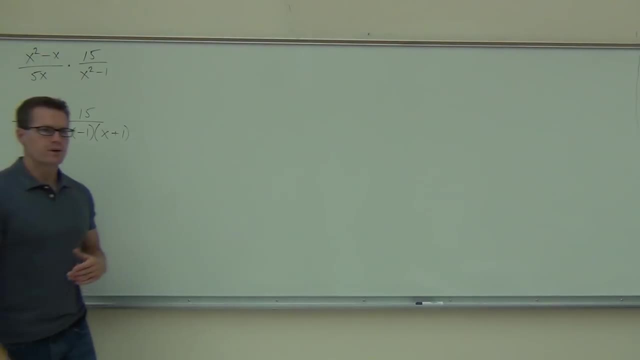 is. I let you, instead of rewrite the whole thing, just extend that line. that's all you gotta do, Because as soon as we extend this line, put the multiplication there and there we now have a simplification instead of a multiplication problem. that's kinda nice. 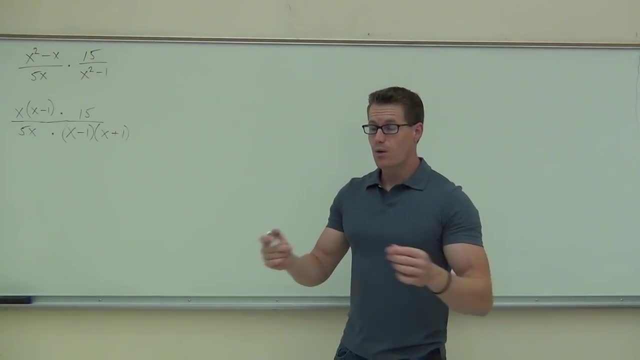 So now we're on to simplification and then we're gonna do this is the best part we get- to cross stuff out. What can we cross out on this problem? The five. Yeah, now we're ready to cross out the five. 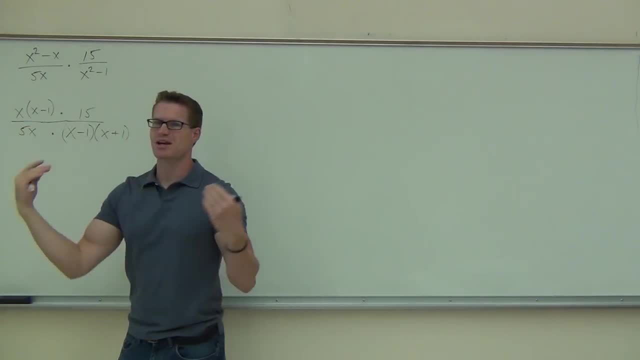 We couldn't do it before because notice, they're not together yet. We wanna factor first. make sure we have this one fraction, then we can do it. The five with the what 15.. 15 becomes a what everybody. 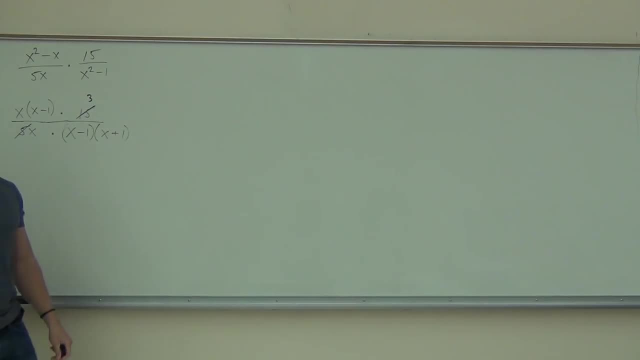 Three. Okay, somebody else, give me another thing I can cross out. Say that louder: The x. let's look at the x. can I cross out the x? They're being multiplied right, That means it's a factor. So this x and this x are gone. that's great. 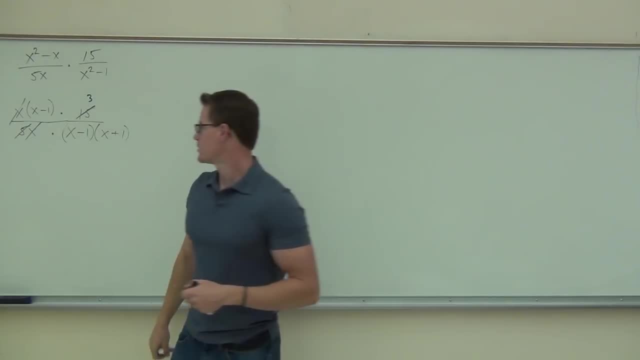 Right hand side of the room. something else I can simplify: X minus one- Perfect. Those are entire factors. we can simplify those out. We're gonna write what's remaining. we gotta be careful not to write anything we've crossed out. 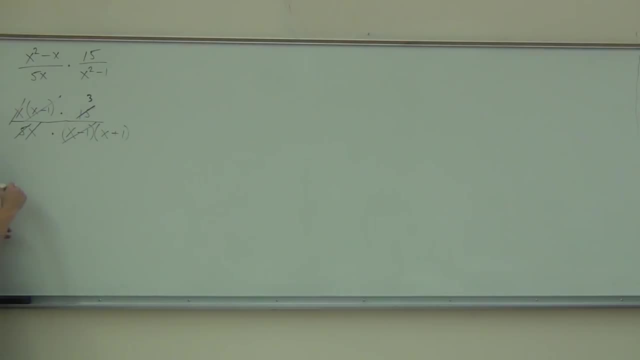 but we can't miss anything either. So, on our numerator, what's left? Three? Well, that's great. How about the denominator X minus one? So all this stuff. when you all simplify it, it's just equal to three. 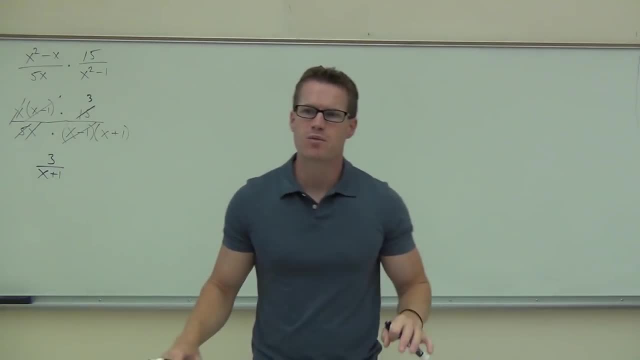 Three over x plus one. That's it. that's as far as we can go. You can't simplify anymore because you wouldn't have been able to do it in the previous step. right there, How many people feel okay about this particular problem? 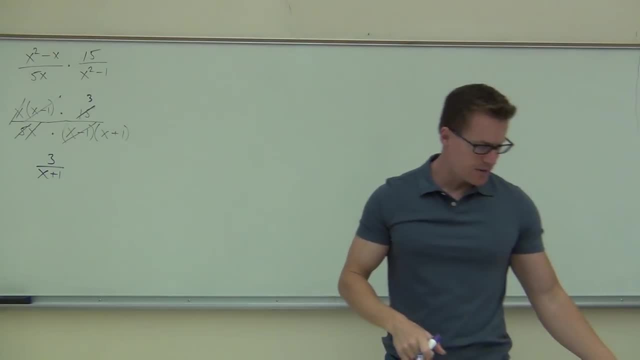 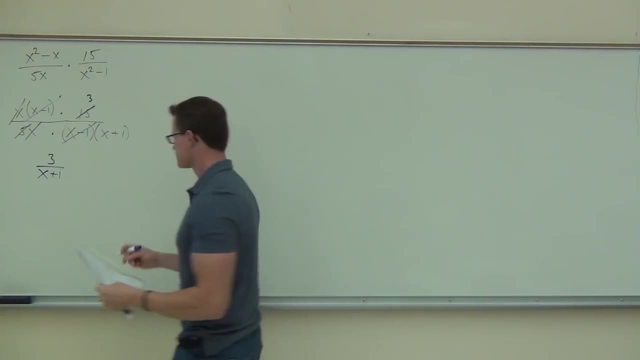 Good, all right, Let's continue on this stuff. We'll do one more together, then we'll start talking about some division and you're gonna find the division is very, very similar to multiplication. There's just one little extra step. 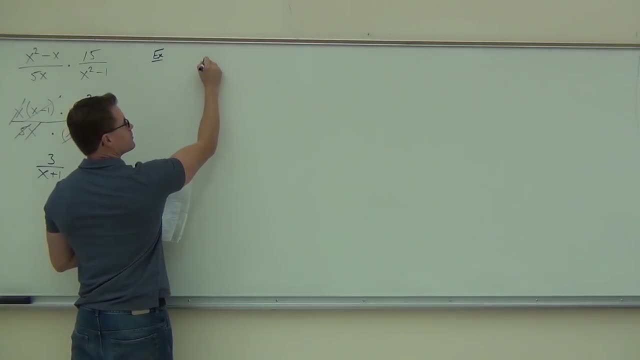 I am gonna have you do some of this stuff on your own on this problem. It's just all about thinking about I don't know what to expect here. You clean this house up, start going to class. nine stories: you're gonna have lunch at 11 o'clock. 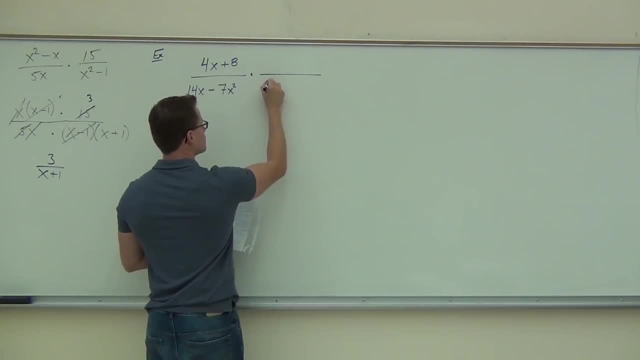 two children come in. you watch this school so much You're gonna have college right next door. I'm just gonna be sitting here like a joke, all turning two stories water together: not appointed. How'd you do You follow them? how'd you do? 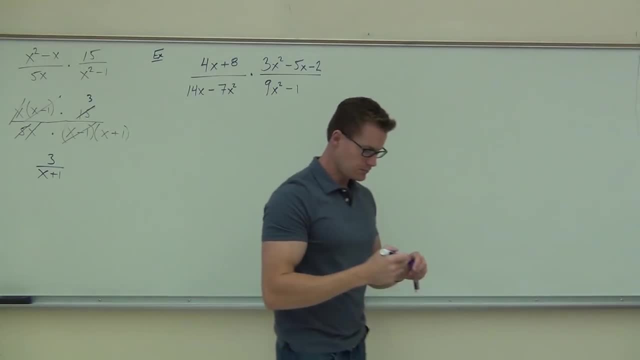 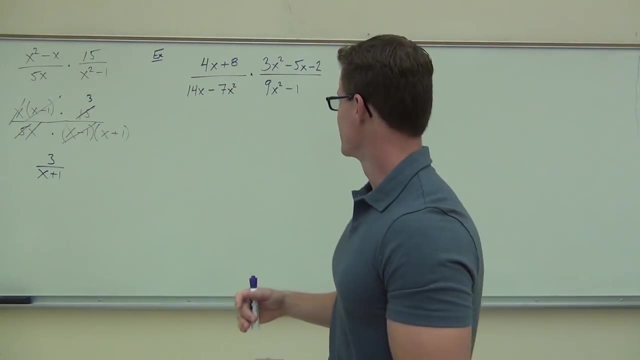 Not me, not you. Neither You're kidding. Okay, we are going to do this somewhat together, somewhat on your own. This is a great problem for us to do. This actually covers pretty much every type of factoring we've done here so far. 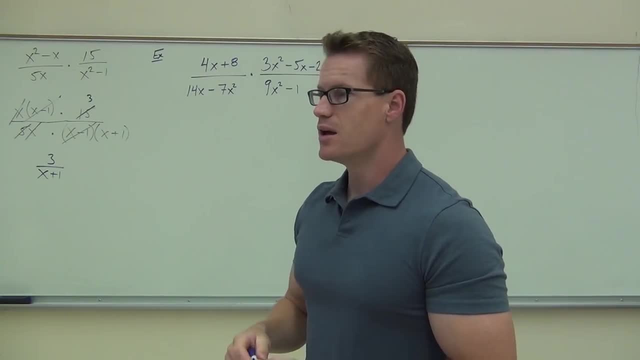 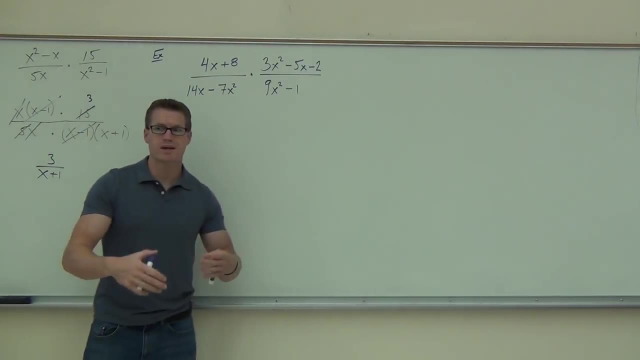 So if you can do this problem, you should feel pretty good about your factoring alright. So let's go ahead, and I'm going to do this piece by piece with you. We'll start with the easy parts of this. So right now, on your paper, the first thing we know we need to do is factor. 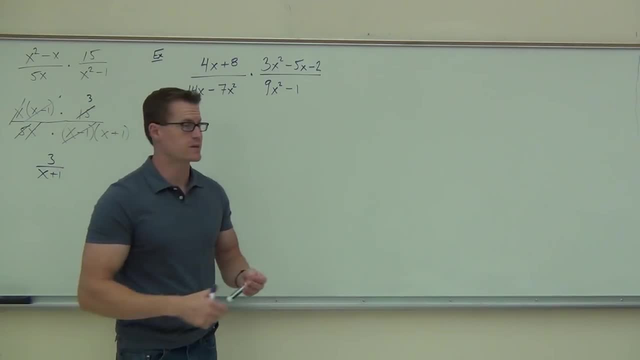 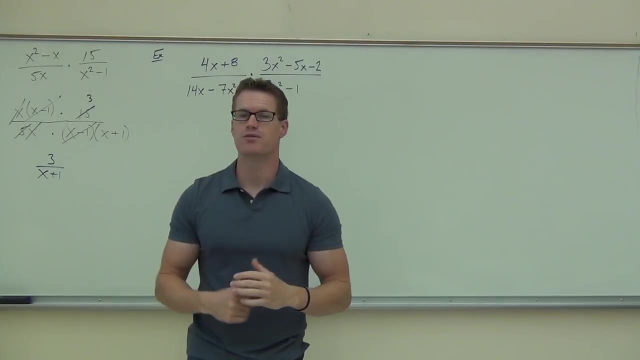 You guys are all with me on that right. We can't really do anything with this unless we factor it. We can't start simplifying three and nine. That doesn't work. You've got to factor first, because you have to do this as one fraction and then start. 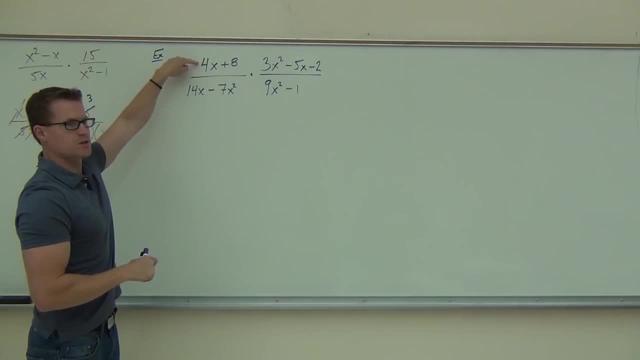 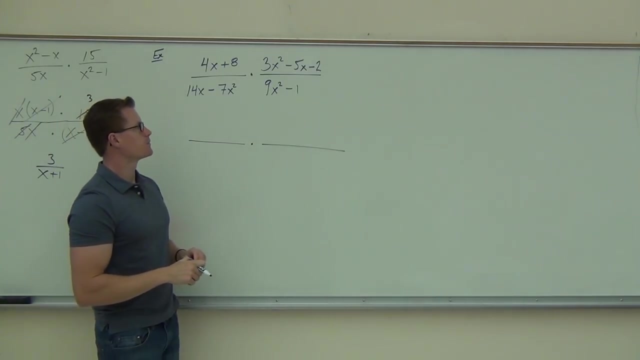 simplifying. So what I'd like you to do, start with your problem. factor this one first. I'll give you about. this is an easy one. let's factor this one about five seconds to factor that. Okay. so the four x plus eight are giving you some time. 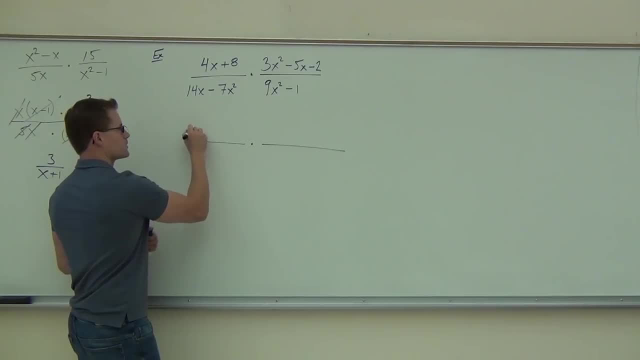 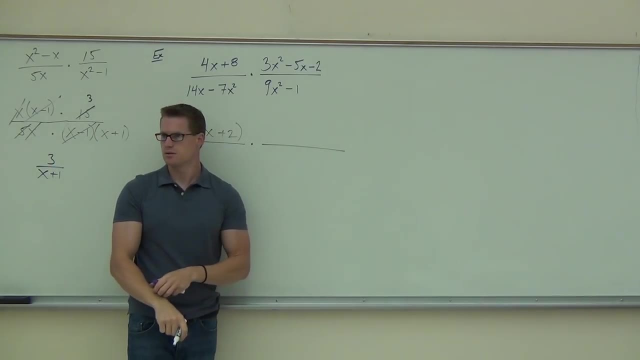 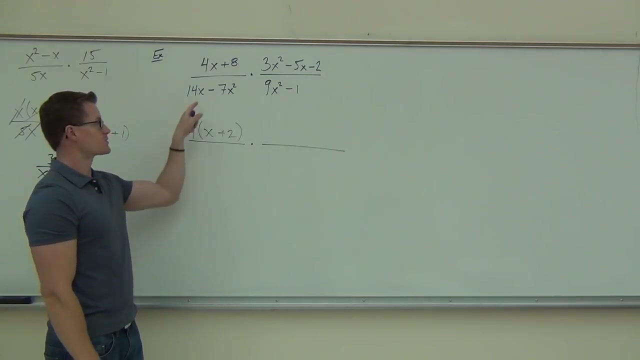 What factors out of four? x plus eight? Good, And you're left with Six. Now, did you have you factored that out and got x plus two? Good, okay, Now let's go down to. let's see which one do you want to do next? 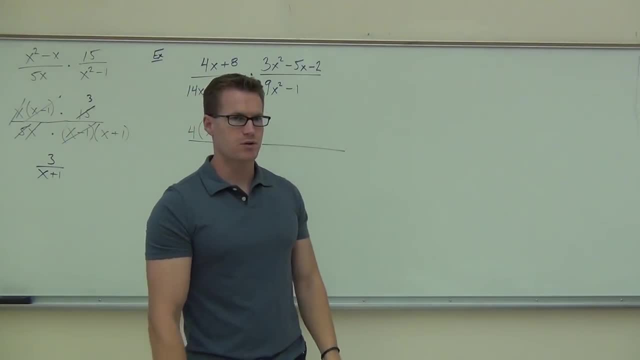 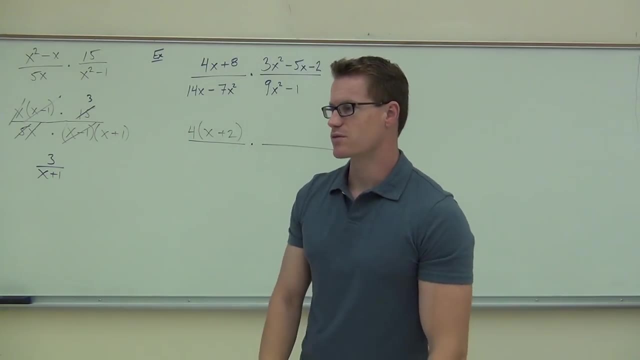 This one. Okay, let's factor that one. Now, there was one thing I told you about that one, Let's see if you can see it. Told you about this, I think last time or something. before that, Factor on your own, see what you can factor out. 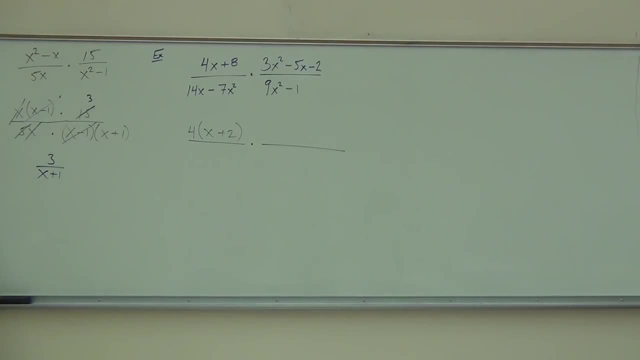 Okay. Okay, so 14x minus 7x squared. You have a couple options here. all right, You have options. Now one of them is going to be a better option for you. I told you this a while back. 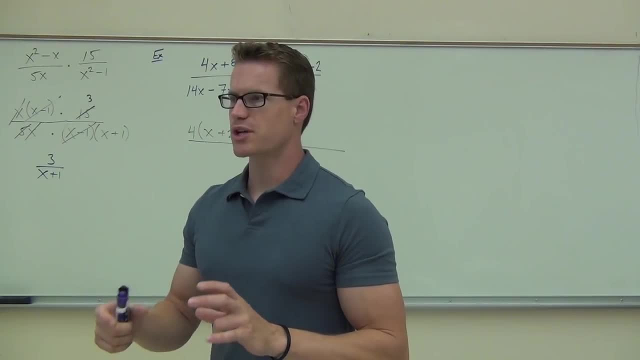 I said you're supposed to factor in order to get the term with the largest exponent positive, because otherwise you're going to have to factor out a negative anyway. Are you with me on this? So in this problem, really you shouldn't be looking at factoring out 7x. 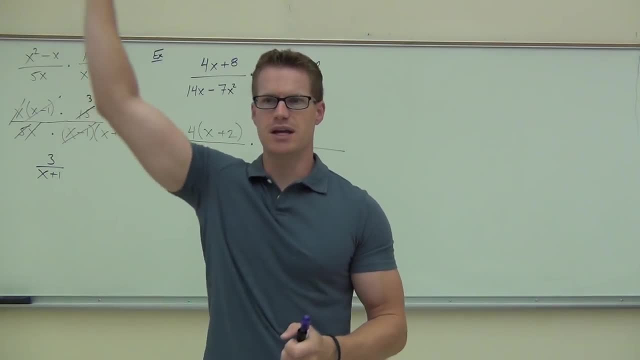 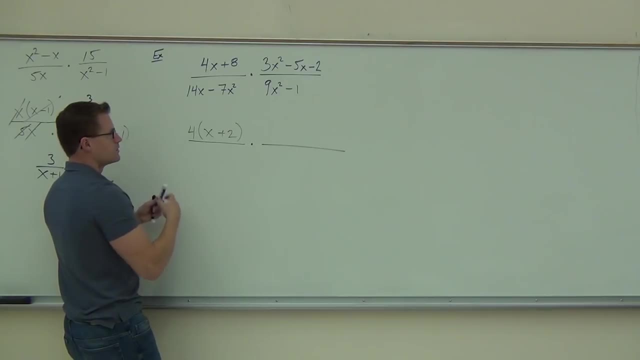 You should be factoring out negative 7x. How many people saw the negative 7x there? Good for you If you didn't now fix the problem. So we're going to factor out. We're going to factor out negative 7 and the x. 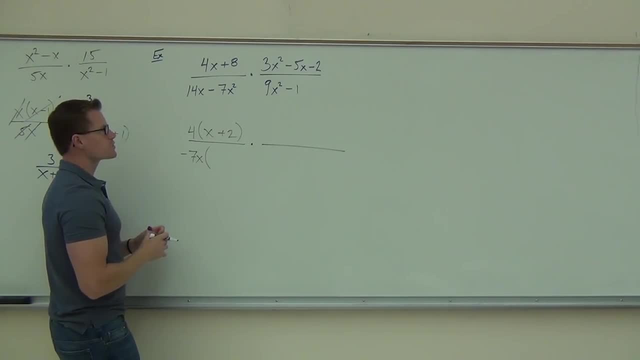 If you do that, factor out negative 7x, what you're going to be left with is negative 2 plus x. Do you see how, by factoring out the negative, we change to both sides? Are you clear on that or no? 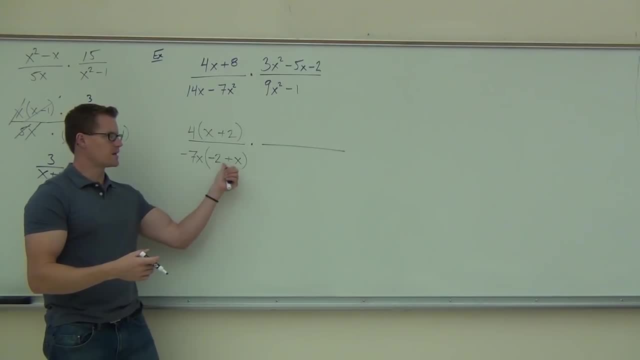 Are you sure? Okay, I just want to make sure that you know why that's a negative and why that's now a plus. Do you see it? So we're factoring the negative out? If you distributed it, We get exactly that thing back again. 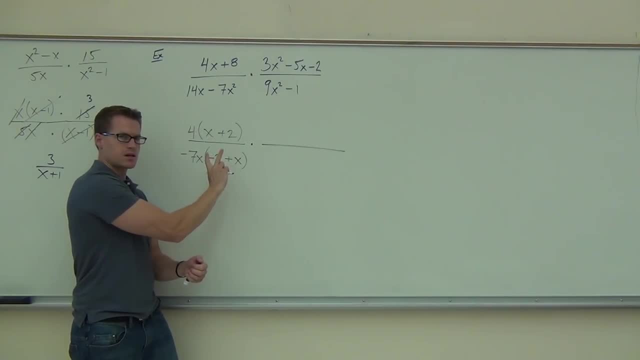 Now the next step I'm going to do on this little part is: I'm just going to take these and flip them around. It's going to be x minus 2. And I'm just going to be okay on that part. Okay, That's going to make things a lot easier to see in the future in the next thing we're going to do. 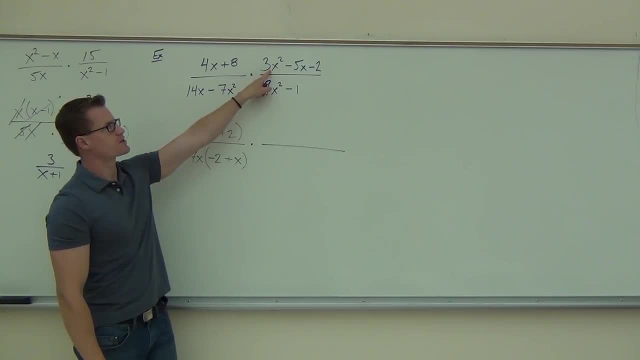 Okay, Let's go down to: oh, let's do this one, Let's do the 3x squared minus 5x minus 2.. You all should know how to factor that one real well at this point. This is what type of problem. 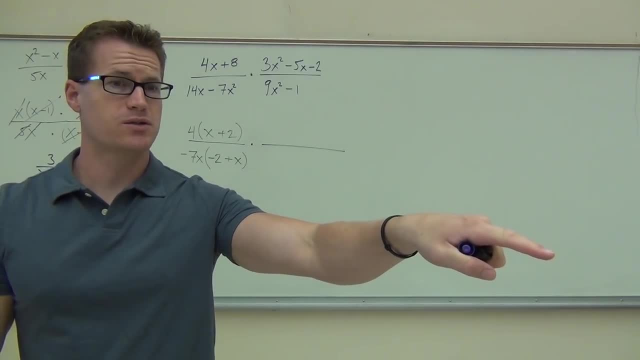 Good And, ladies and gentlemen, I want to thank you for watching this video. If you're on the left-hand side of the room, is this going to be the extra step where we have to factor by grouping, or not? Okay, Do that now. 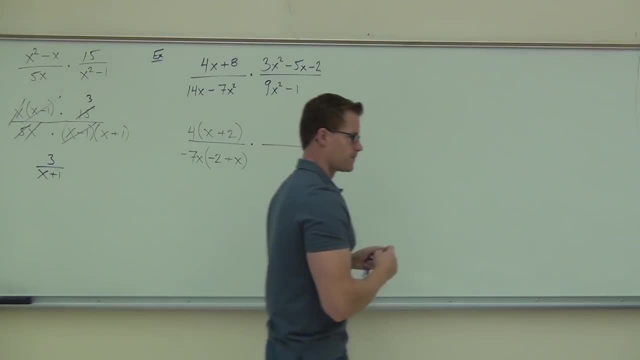 I'll give you about a minute. You should be pretty good at this stuff right now. Also, guys, try to go through that homework kind of quickly, because I have a lot to. I have four assignments to get back to you. If we don't do it now, it's going to get backed up. 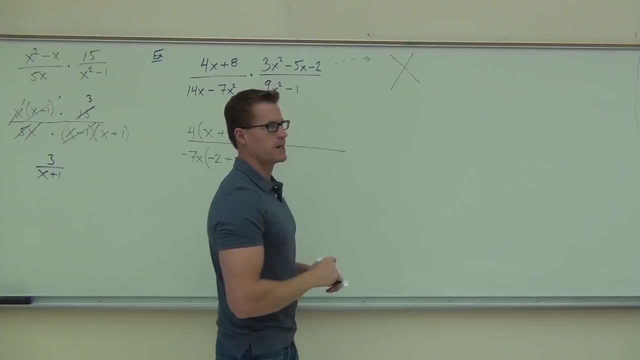 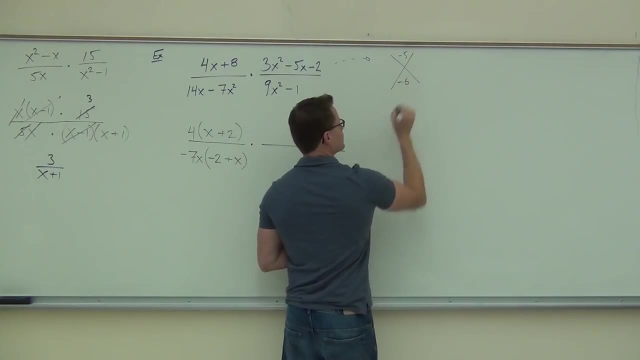 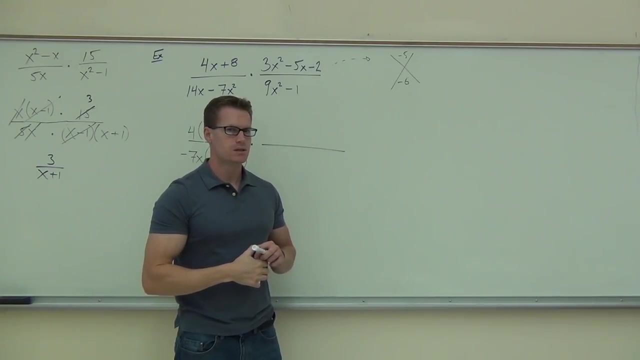 Okay, everybody, what number goes up top? What number goes on the bottom? Just add negative 5. You're supposed to multiply the negative 6.. Yeah, a lot of people try twos and threes here. Twos and threes aren't going to work. 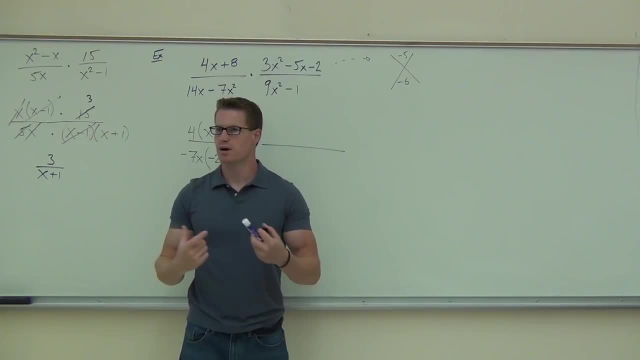 You're going to have to multiply the negative 6.. That means you're going to have one positive, one negative and they're going to have to add a negative 5.. Threes and twos won't cut it for you, So you're going to have to add a negative 5.. 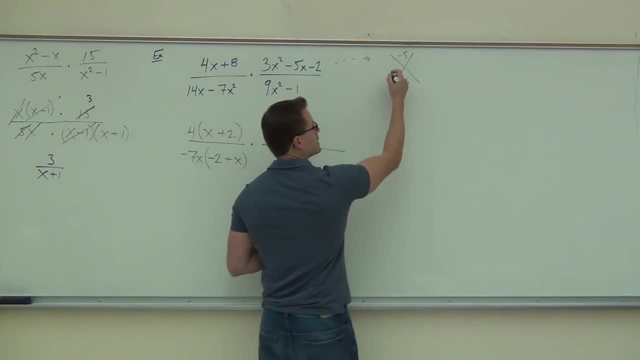 You're going to have to add a 6 and a 1 somehow. In our case, we're going to have a negative 6 and a positive 1.. Negative 6 and positive 1 is only two numbers you're going to get. 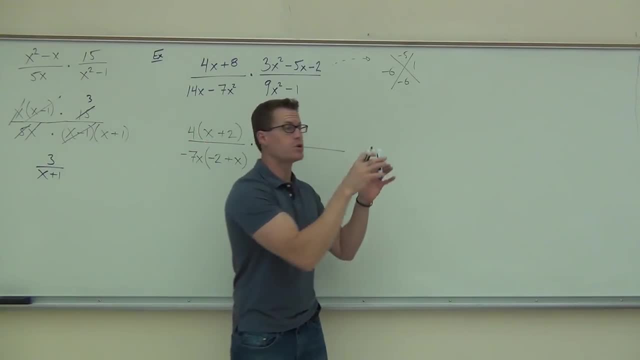 Did you find negative 6, positive 1? Good, all right. Now we can't just put x minus 6 and x plus 1.. We can do that if there's no number out front, like that. That'd be great. but there is a number out front. 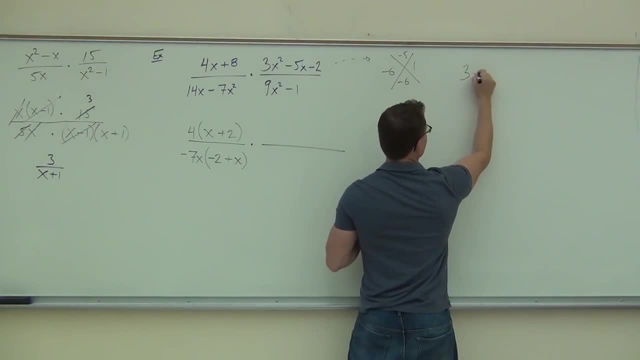 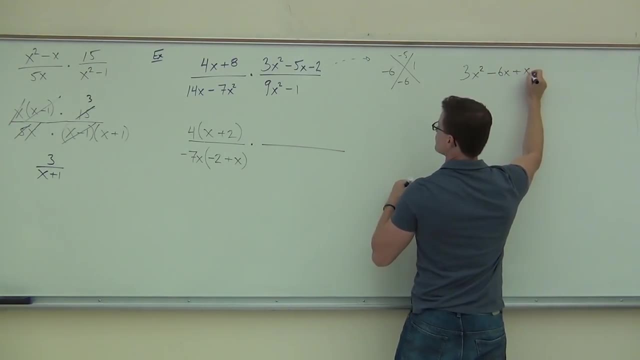 That means our extra step says we're going to do Factor by grouping, Yeah, factor by grouping. In order to do that, we make four terms out of it. We look at the first two. What factors out of the first two is a 3x. 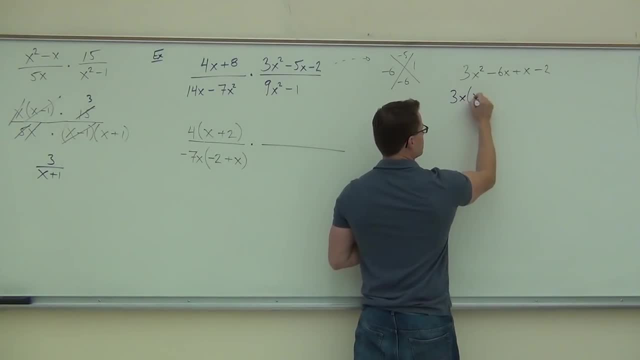 So we factor 3x, we get x minus 2.. We look at the second part, There's really nothing that factors out of those two terms. So we factor out a 1.. So we're going to do plus because it says plus. 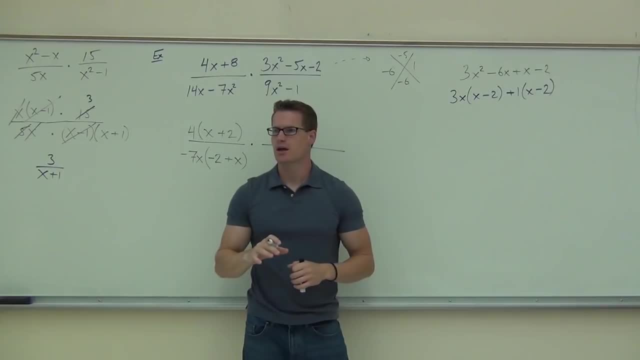 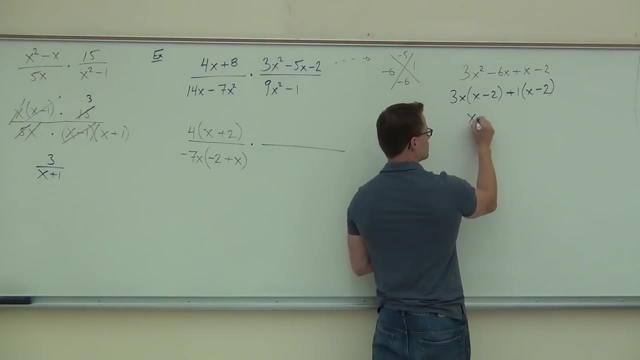 We still add the x minus 2, because factoring out 1 doesn't change anything. Have we done the problem right? Yeah, it looks right, because we have the same thing in both spots. So we continue on And that's our new numerator. 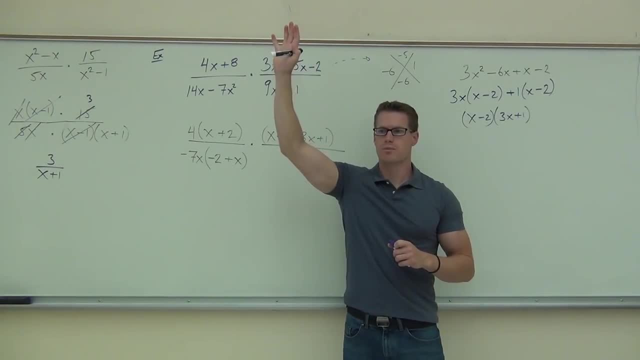 How many of you are with us so far? Feel like this, Good, Hey, there's one more part. Let's look at 9x squared minus 1. Factor it. Okay, So you can put that together. We're going to use the denominator. And you can add that. So you can add that to the denominator. So you can add that to the denominator. I don't know, I'm just having a little bit of fun. I don't know if I can add that Here. 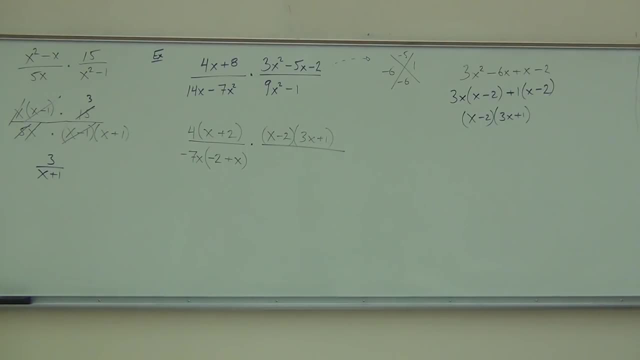 I'm sorry, I can't say it. I'll say it Here One more time. So we put that together. So that's what you were able to do. I put it up So you can add that to the numerator. 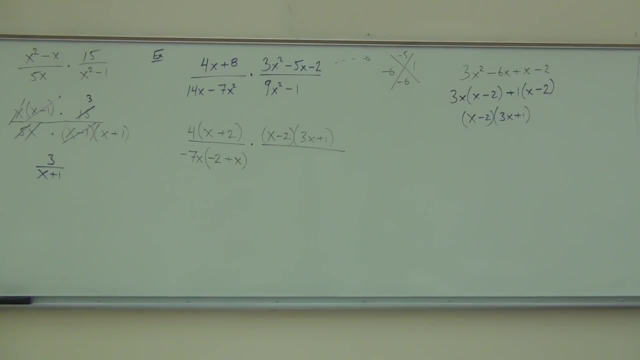 So now we add that That's good. So we get four terms out of it. So we add that down, So we add that to the denominator. So then that gives us an alternative. So we add that to 9x. If we factor 9x squared minus 1, we look into this and we see we have how many terms here. 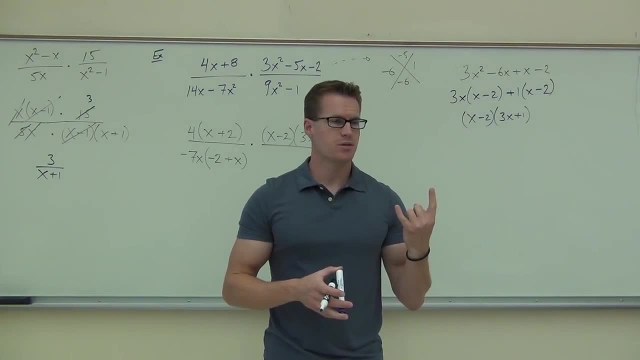 How many terms here? Two terms, Two terms. So that means we look for greater than one factor. of course there's not one, because we have a 1 up there, but this isn't a diamond problem. this can only be really one thing. 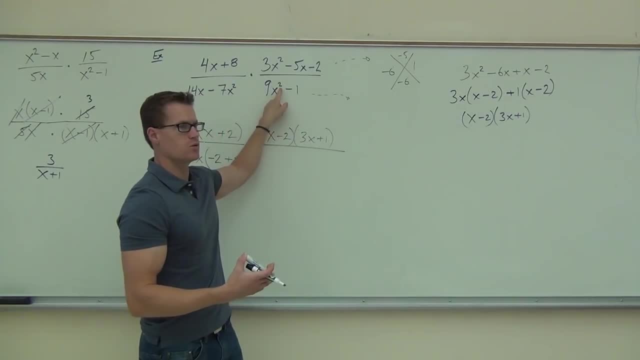 for us, This could be a difference of squares, because we don't have a cube or nothing. In this case, this is a difference of squares. did you see the difference of squares? Now, how in the world is there a difference of squares? 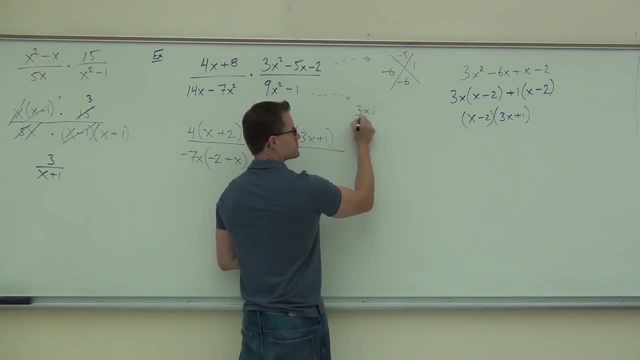 Well, we can write 9x squared as 3x squared. did you buy that? That's 9x squared and then minus instead of 1? you really could. you could write 9x squared. You could write 1 squared. 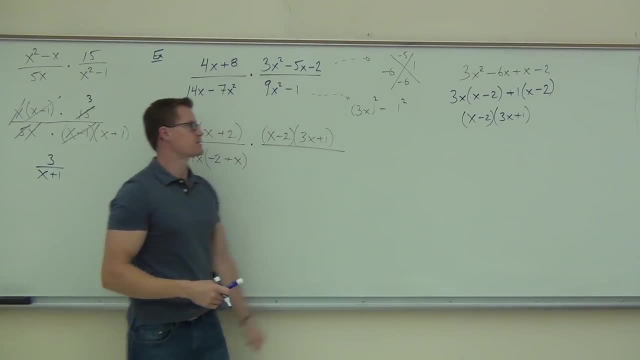 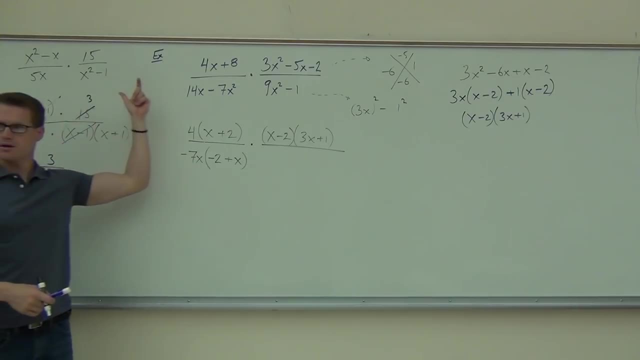 And so what this is is exactly the same as this. This is the same as this. basically, It's just instead of x squared, you have 3x squared. Are you with me on that Difference of Squares? We've done that several times now. you're going to be pretty good at this at the end. 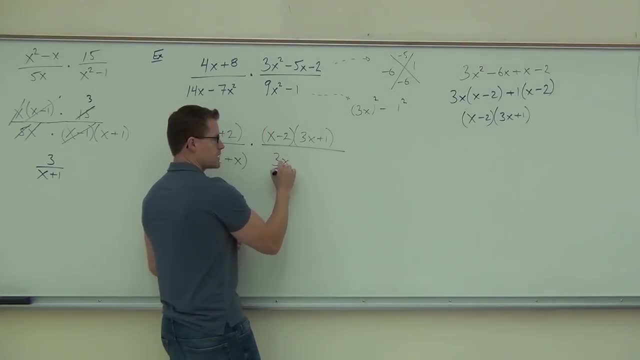 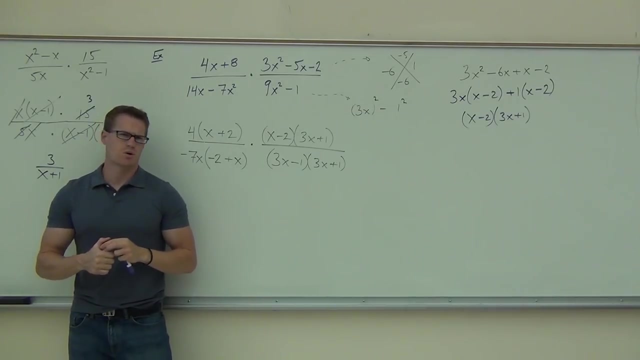 of the semester. So we get to factor this as 3x minus 1,, 3x plus 1, just like we did this. Ladies and gentlemen, are we okay on the problem or no? Imagine, if you're okay, You can follow it down. 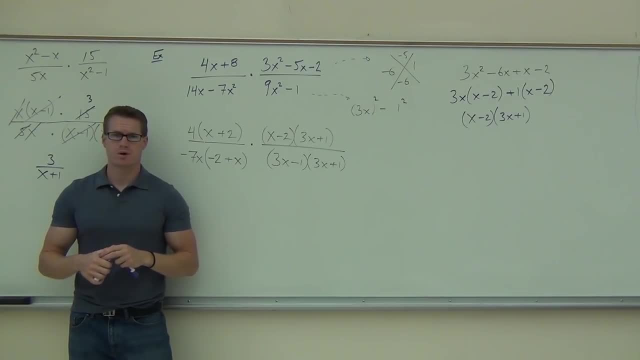 You might have to go back and try this problem on your own. Trust me, you don't want to just sit here and follow it one time, because of course I know how to do this stuff right. It's going to make sense when I'm doing it, but it might not make sense when you're doing it. 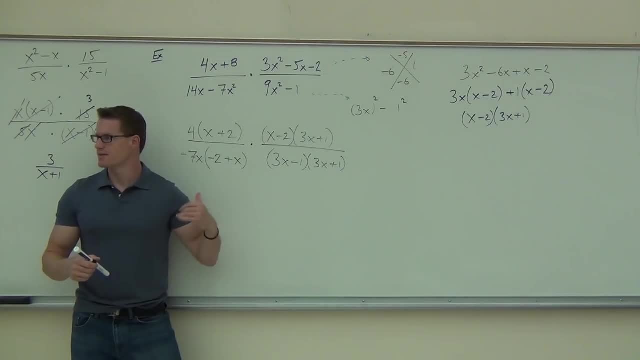 So go home and try this one again. Make sure you can get this again, okay, If you're not doing it? I had a snafu with the lecturers. I couldn't get them on this weekend. The hard drive just didn't matter. 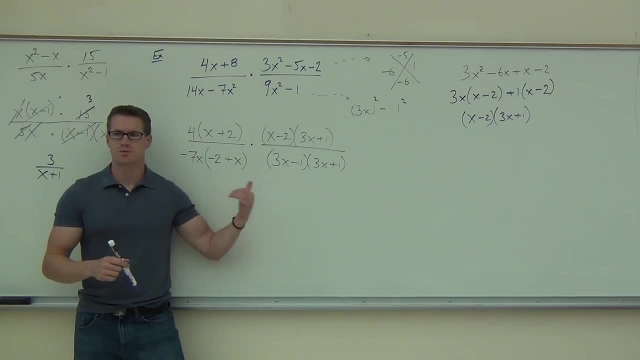 I was not so happy last night, But these will be on probably tomorrow afternoon: the lectures. Can you make the negative 7x times the negative, 2 plus x as x minus 2? That's exactly the next step I'm going to do. 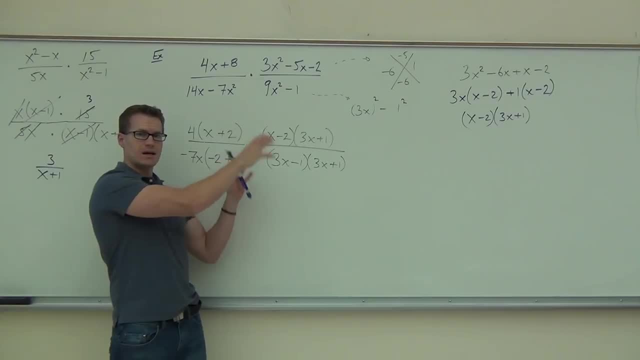 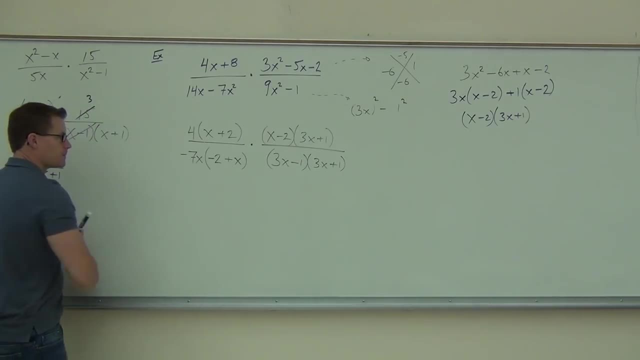 Yeah, that's a great point. So are you okay? getting down to this far, so far, Okay. So the next thing we are going to do is: is that what you said? Are we okay? That's hard for you, right. 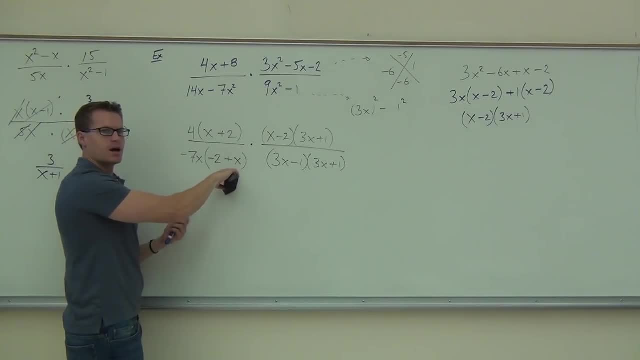 Okay, Well, hard for you to say is: can't we write this a little bit different? And yeah, we're going to. Instead of negative 2 plus x, I'm going to keep these, the signs with the terms. 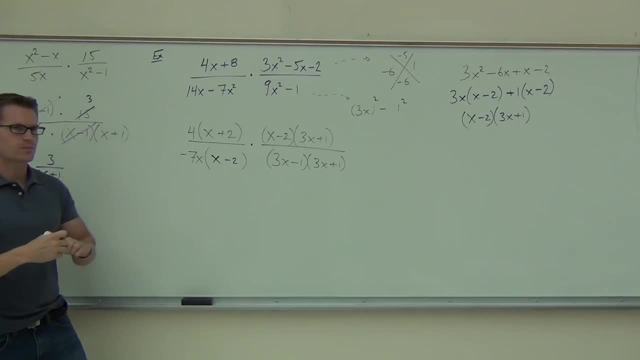 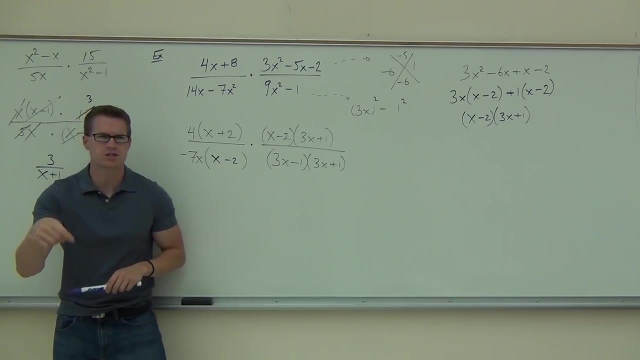 and just do x minus 2.. So I'm going to give you the next step I'm going to do. Before that, before I start simplifying some things, I'm going to do one more thing. Yeah, I need to see one fraction out of this. 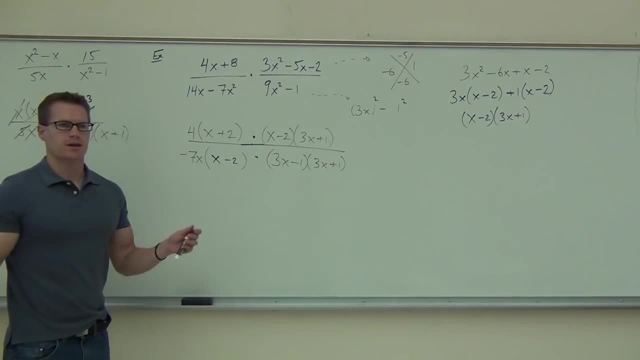 So I'm going to extend this: Put the dot dot. That's the only thing. I just want one fraction right there, That's it, And then we can start simplifying. Shout out some things that we can simplify up here. 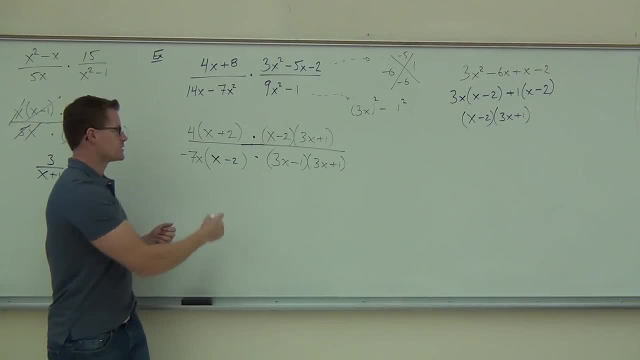 X minus 2.. Okay, Someone else, give me something else. we can simplify up here. Three x plus 1.. Great, Wait a second. Even though they're on the same fraction, I can still simplify those. Sure, Why not? 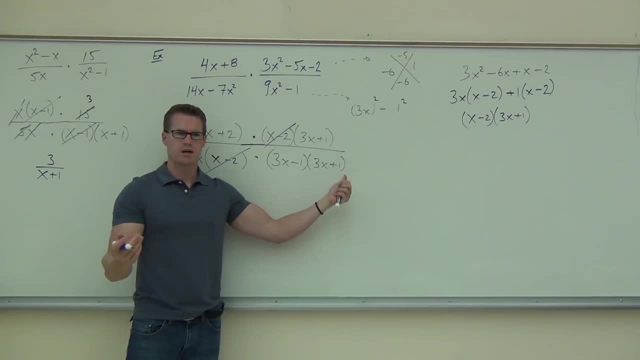 Yeah, You're just looking for common factors. It doesn't really matter, And it doesn't have to be a cross from each other. Is there anything else we can simplify up here? I got a. how about the four Seven? This one? 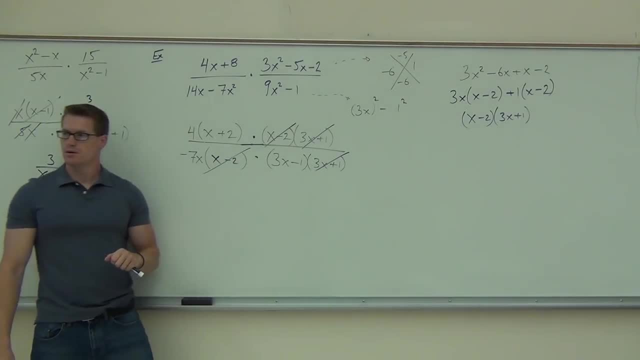 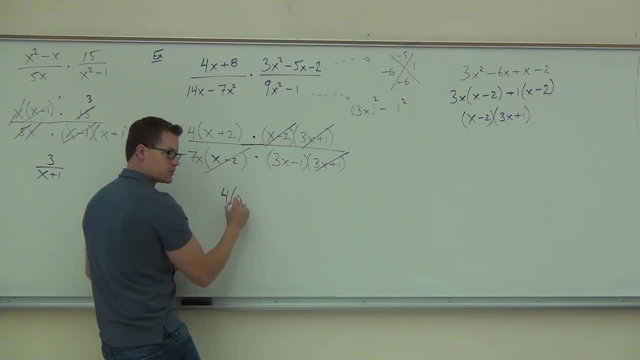 Three x minus 1.. There's nothing left, Nothing like that, So we're just going to write what's left over. We've got a 4 and an x plus 2.. We've got a negative 7 x Three x minus 1.. 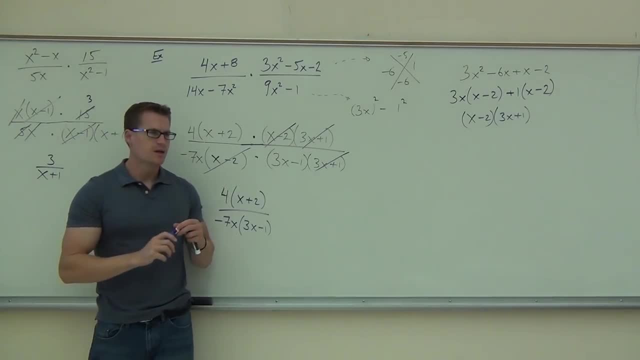 Don't distribute it, You just leave it Just like that. Now again, the reason why we've factored out the negative 7 up here is so that these, these two expressions would simplify out. Otherwise you'd have to factor a negative at this point. 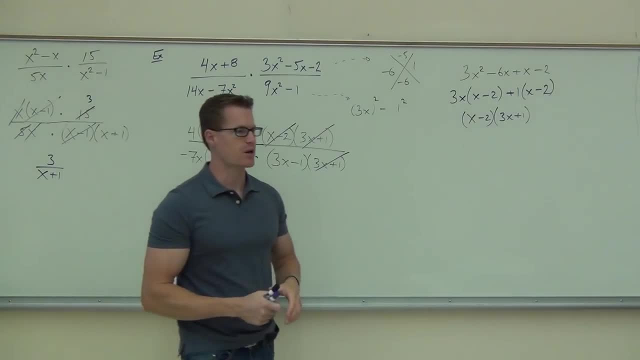 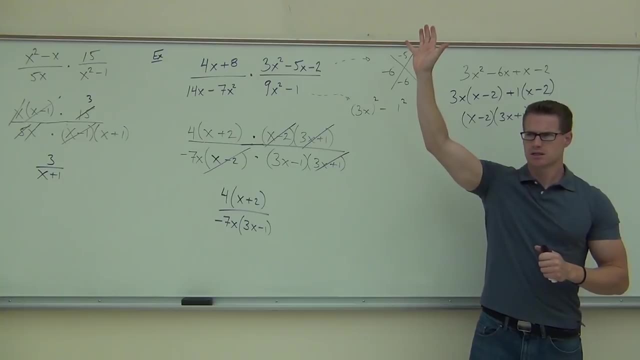 Are you with me on that? You'd have to do it somewhere. You may as well do it again. it's easier that way. Do you feel okay about multiplication today? Raise your hand if you're okay about multiplication today. Good, So we learned that multiplication. 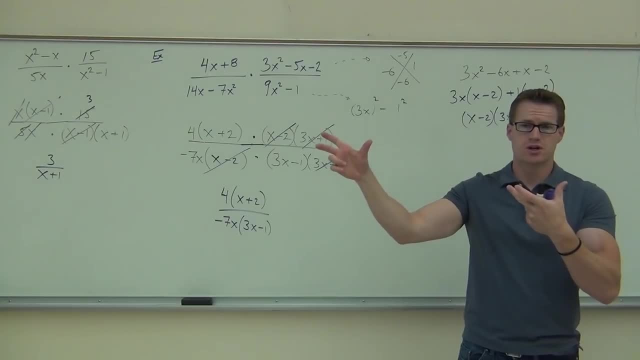 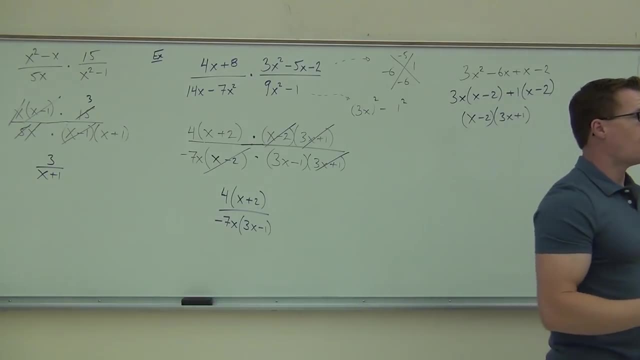 is basically simplification. It just happens in two different fractions, So we're simplifying two different problems at once. basically, if we get to put them together as one fraction and then we go. Let's see what happens now with some division. 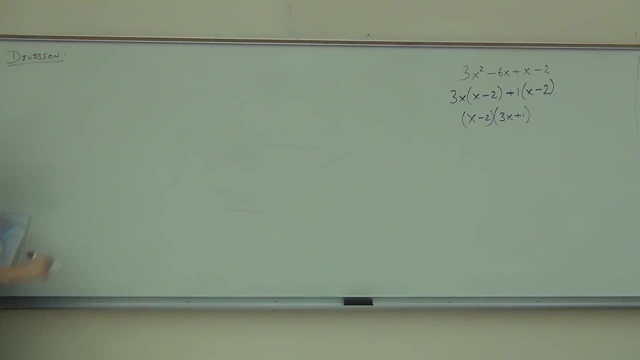 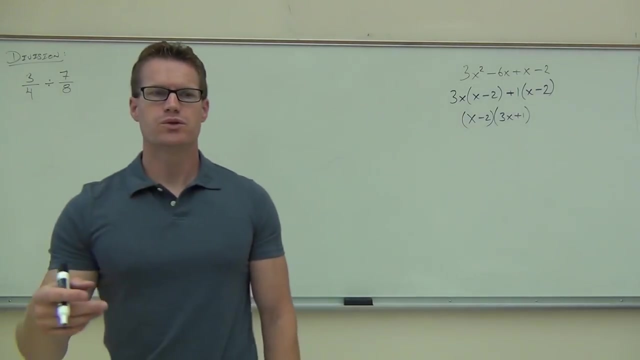 Just like before, we're gonna start off kind of nice and easy with some basic, basic fractions here, And the question is- I know you know this because you're in this class- but how in the world do you divide fractions? Is there a way to actually directly divide fractions? 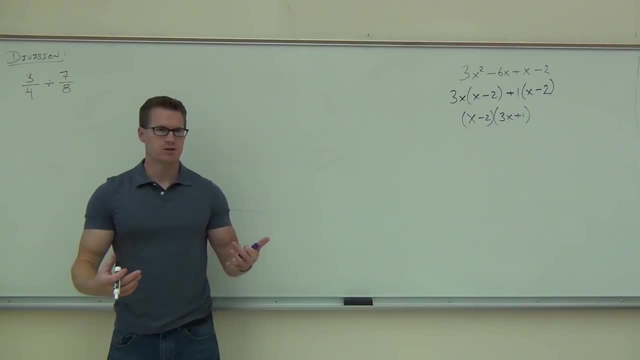 or do we have to manipulate this somehow? Manipulate them? Yeah, you really can't just directly divide them, right? It's really hard to think about that If you really think about what's three-fourths divided into seven-eighths parts. 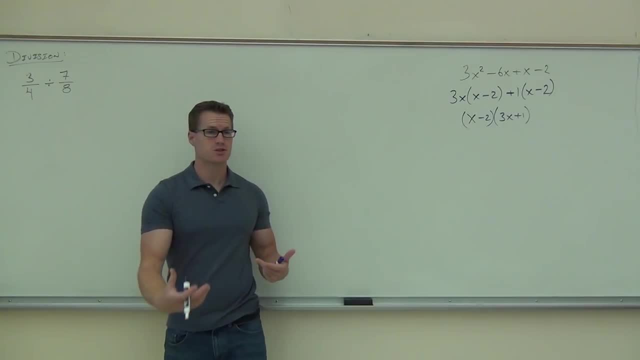 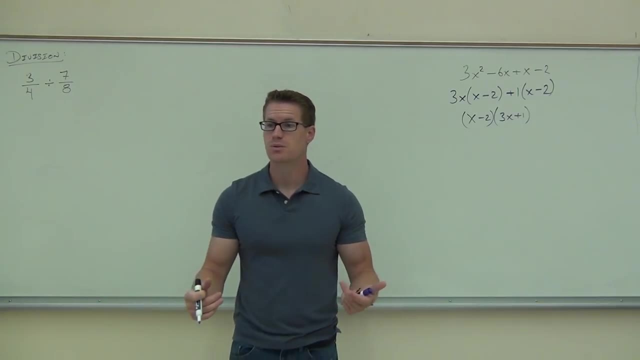 I don't even know That's kind of weird to even contemplate that. But we have a method of doing this thing. What's the method of actually dividing our fractions here? Flip one and multiply. Do what now? Flip that half one. 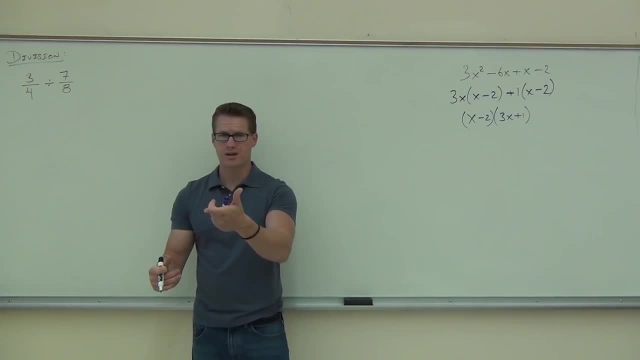 Flip one. okay, yeah, that's great, We flipped one. What's the flip one? what's that called Supernova? If we're gonna find the reciprocal, we're gonna reciprocate it right, Reciprocate that fraction. 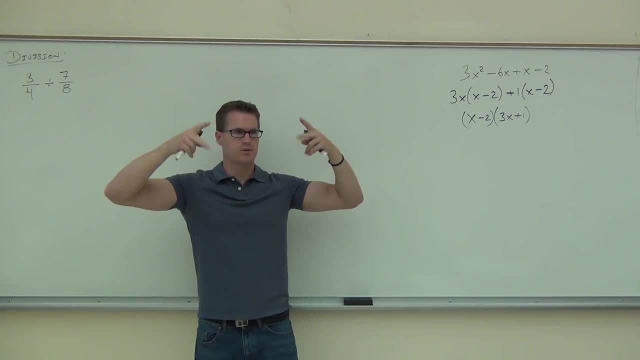 Now do we reciprocate the first one, the second one or both of them, Which? The first one we leave alone. Second one: we reciprocate that one. So we reciprocate the second fraction, and after we reciprocate the second fraction. 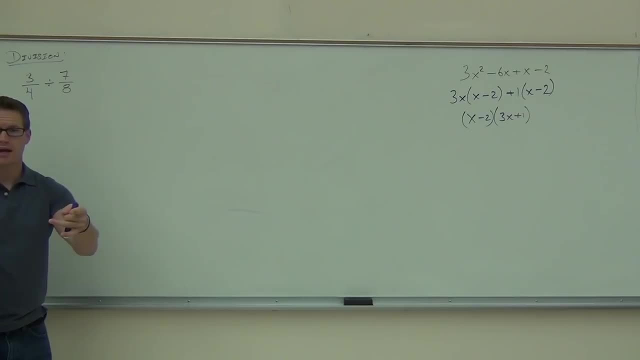 we do what to it? Yeah, multiply it and then we'll write as one fraction. So we're learning that division literally has one more step than multiplication. That's really it, and it's not even a hard step. You just have to remember to reciprocate. 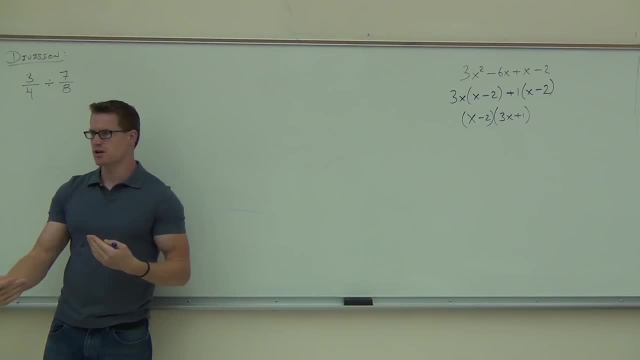 the second fraction, then you're back to multiplication, which we just finished covering, which essentially is just simplification, which is basically just factoring. So if you know how to put fraction in factors, you know, that's it. So we're going to reciprocate the second fraction. 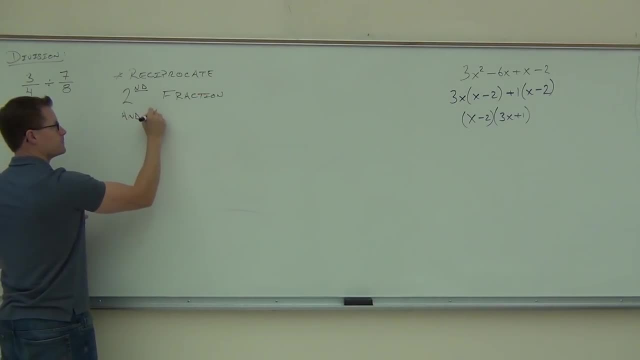 We're going to put in the second fraction And then we're going to multiply it, And then we're going to get the fourth fraction, and then we multiply it, The fourth fraction, we multiply it, And that's going to be the second part. 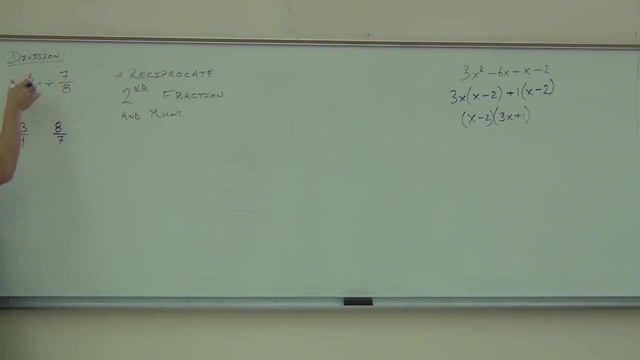 the last part of the big picture, And then we're going to multiply it. So in our case up here, what we do, like you've seen many times, before we leave the 3-4ths Instead of 7-8ths, we make that 8-7ths. 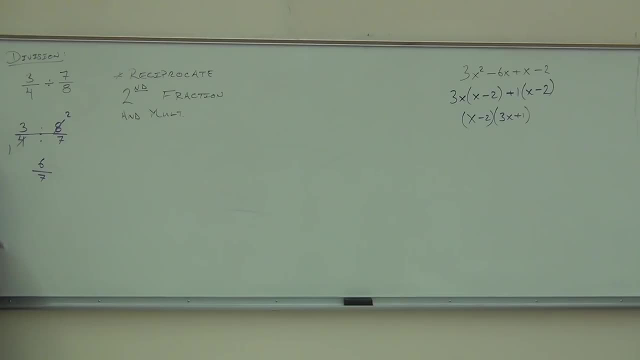 That's the reciprocal, And then that changes the division into: We get six seconds if I've done that right. I think I have and we're good to go. Are you okay with the division of simple fractions like that? Good, Let's try to extend this concept to our rational expressions. 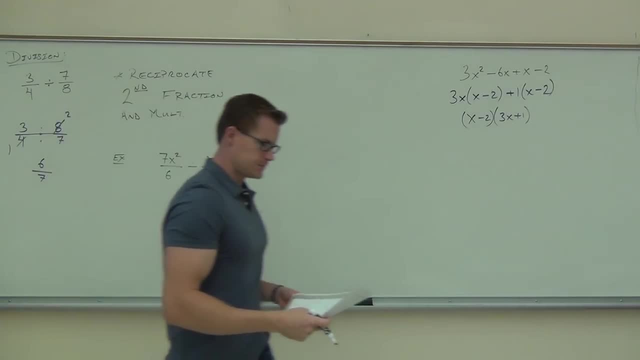 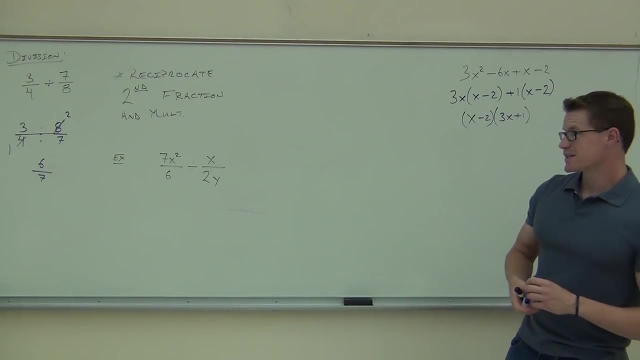 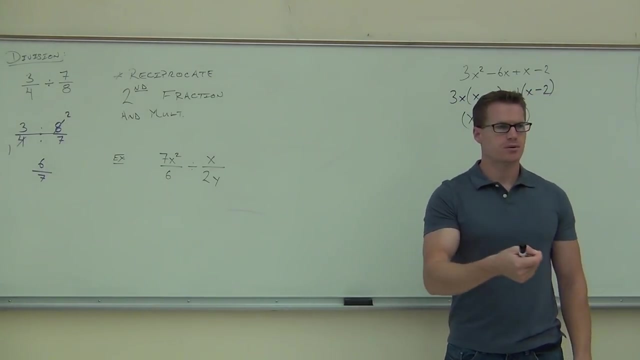 So 7x squared divided by 6, divided by x over 2y, and our first step again is what's our first step? Reciprocal, Reciprocal. okay, So we're going to find the reciprocal of. again, we're talking about which fraction here? 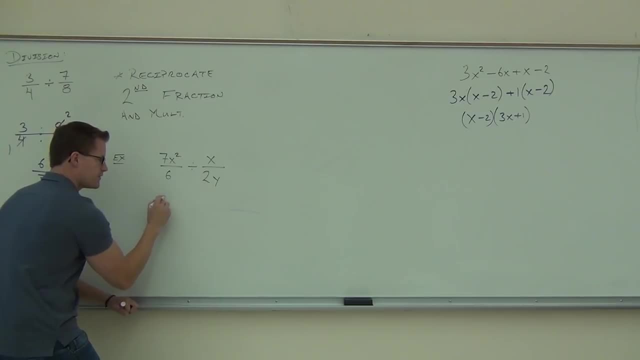 Let's do that. So the reciprocal just means we're going to leave the 7.- Okay, x, squared alone over 6. Instead of dividing, we'll be multiplying, and we're going to flip over or reciprocate this second fraction. 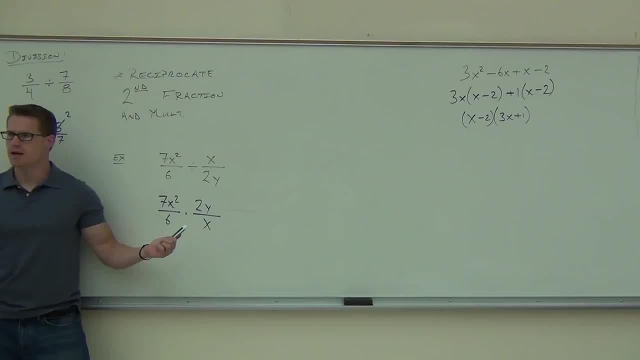 And this is something we just finished doing. That's great. We know how to do that. What's the first step in doing this one? What was that again? Good, Okay, We want one fraction out of it before we start simplifying. 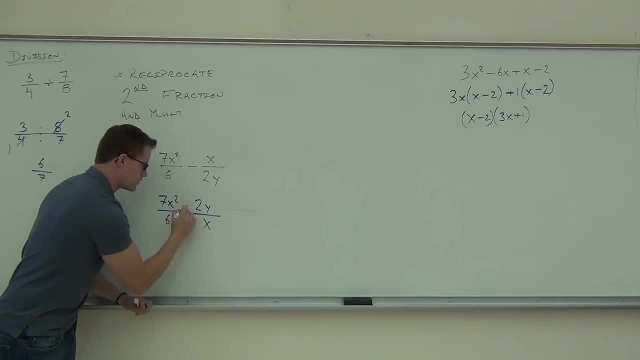 So we're just going to continue that concept. We make one fraction And, as someone who hasn't spoken yet today, what's the first thing? What's the first thing I can simplify here? Say that again, 7x squared. 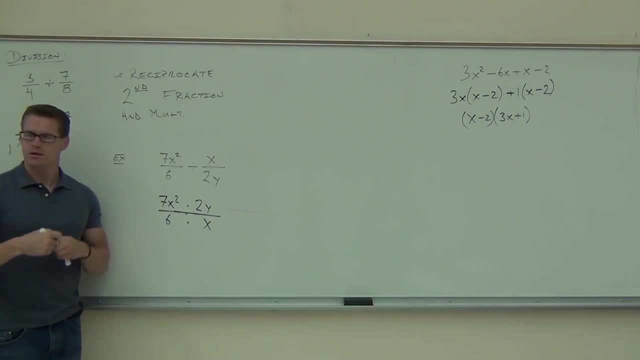 7x squared, Okay. What part of that? X squared, Okay. X squared becomes what? And what else happens? The x from the two ones on the bottom, Good, Okay. Anything else that you see The 6 and 2.. 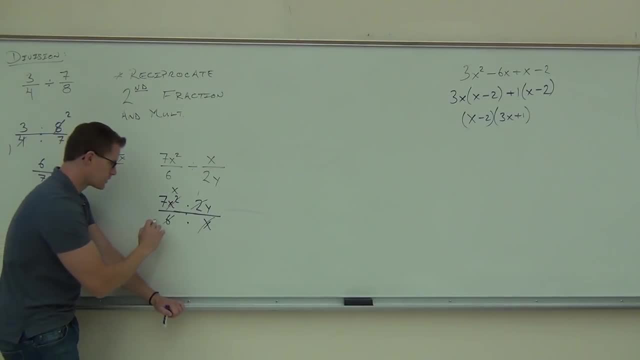 2 becomes 4.. 6 becomes Perfect. Anything else that you see? Anything else? No, I think we're done there. We're going to write the numerator as the multiplication of those remaining factors. Denominator is the same thing. 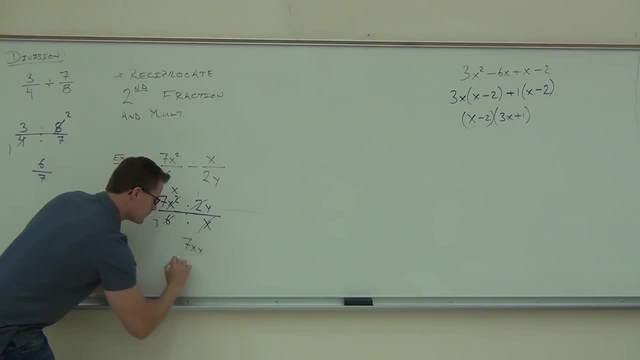 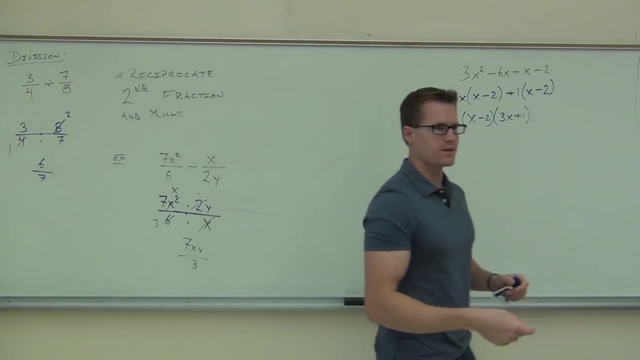 So we have a 7. We have an x, We have a y, All of the 3.. That's it As far as we can go. Let's try one before we make this any more complicated, Just to make sure you have this down. 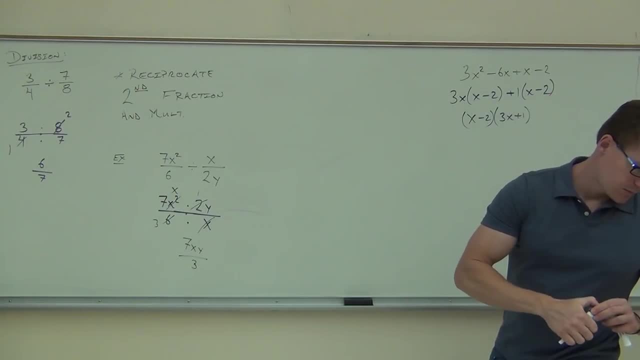 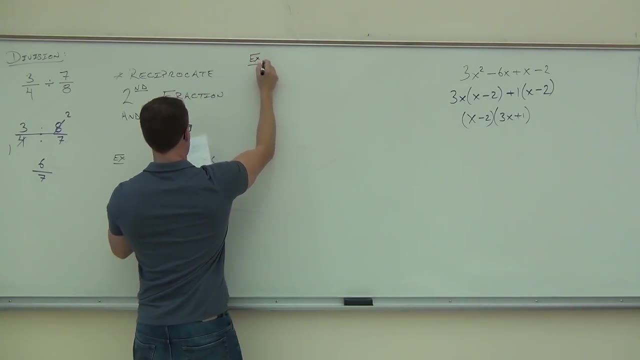 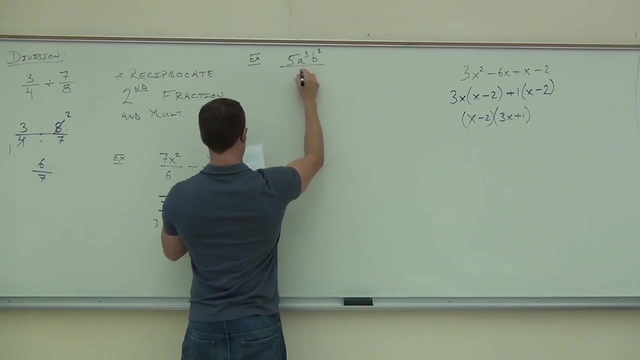 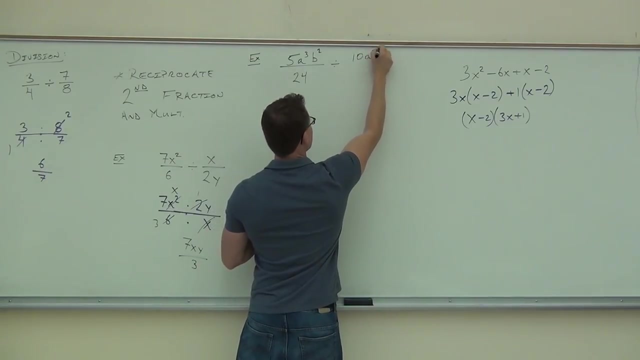 Then we'll keep going. Okay, I'll be tight. So let's see, We have 45 for any agency And then we'll get 1.. Let me get this back up. I'm going to get the children down. 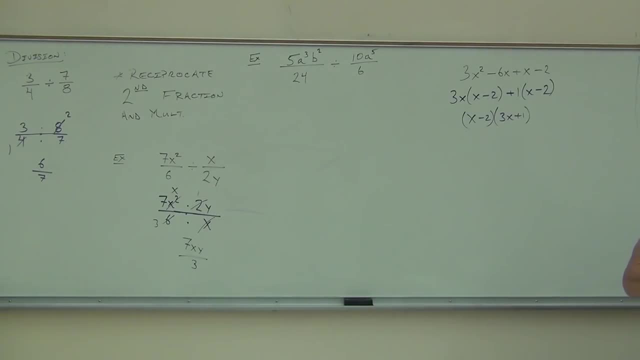 Okay, 1. Here we go. 2., 1., 4., 5., 8., 9., 10., 11. 5., 1. 3., 12., 5., 4.. 2., 5., 6., 4., 6., 5., 6., 7., 6., 17., 8., 8., 9., 9., 10., 20., 22.. 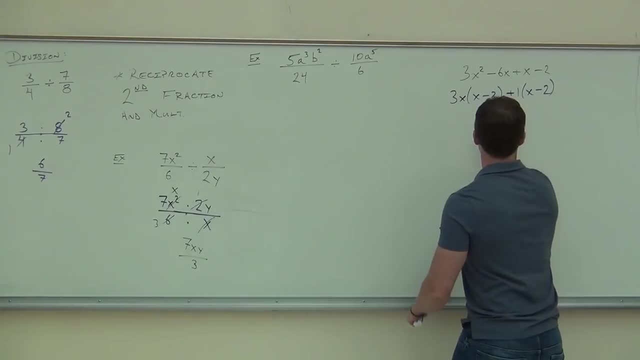 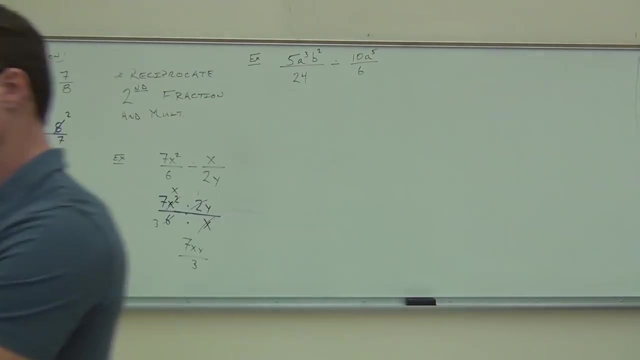 22. 22. 23. 8., 23. 24. 24.. Is that homework still going around? Have you guys gotten the first assignment yet? No, Okay, hurry, What's the first thing you did? 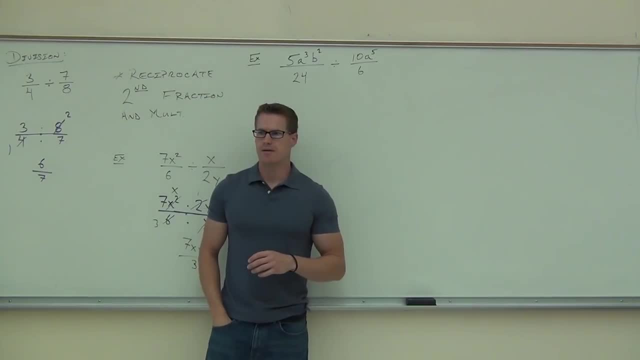 Flip this thing, Okay. Do you know, by the way, why I have you wait until you have one line before you simplify? Here's a good reason why: Because if I don't have, you do that. a lot of times people look at this fraction and go. 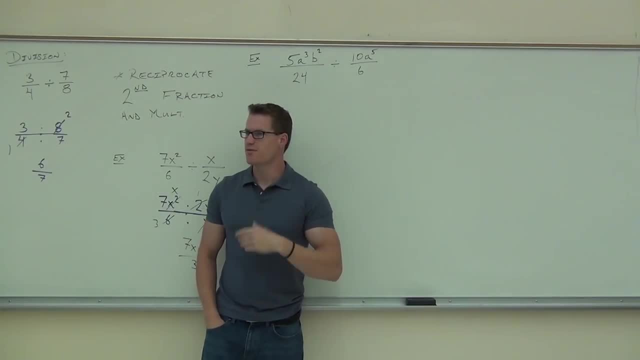 oh, you know what I see? I see the 10 and the 24.. I can simplify that. Do you see how? if I don't have you write one line, then some people are going to do that. See what I'm talking about. 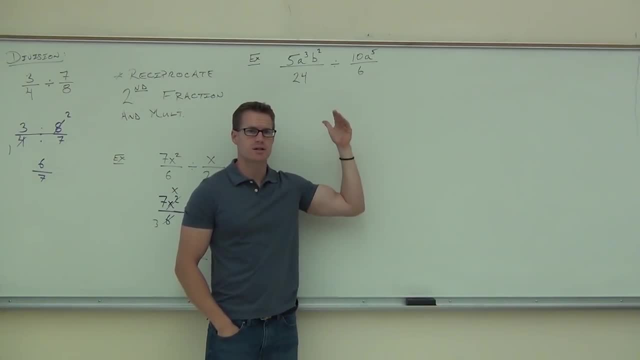 Oh, 10 and 24.. Two goes in the boat, We get five and we get 12.. Yay, We can't do that here. We have to wait until we can write it as one fraction. that only happens on multiplication. 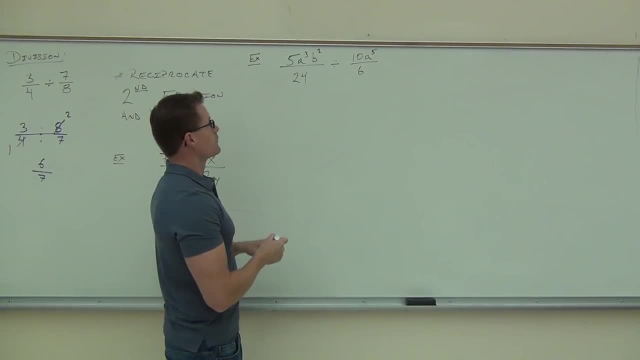 That's why I have you do that step. So here we go. all right, First thing we're going to do is reciprocate the second fraction. Of course we're going to be multiplying, but now we're going to be multiplying by 6 over 10,, 8 to the 5th. 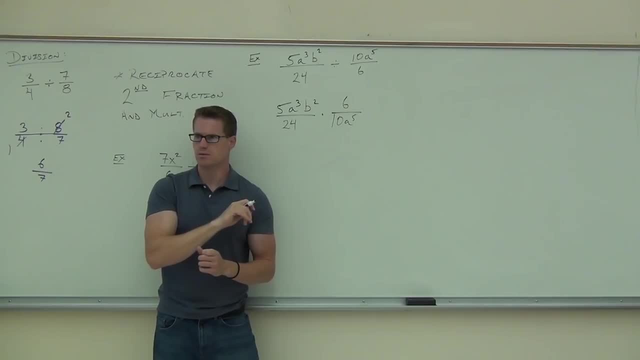 Nod your head if you did that step correctly, Sweet Good deal. Next thing we do is what? Before we simplify- Yeah, before we do that, I want to see that This allows you to simplify things. It says: oh, I have one fraction. 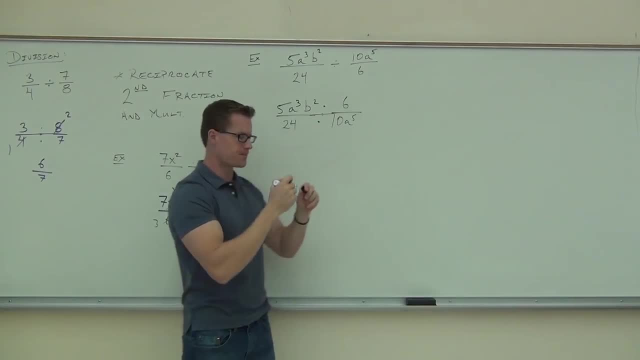 One fraction is how we simplify Common factors, Both the top and bottom. We do that part And now we get to go. okay, the things I see here are 6 to 24.. 1, 4.. Did you get that one? 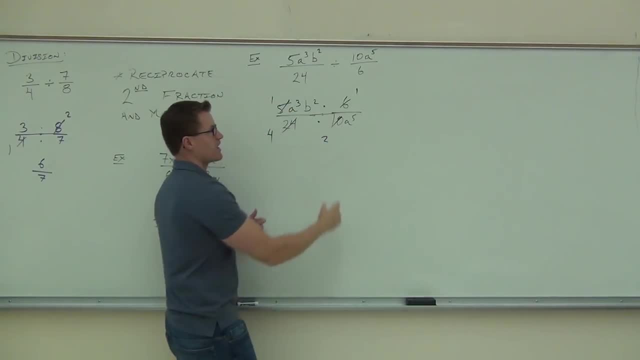 We get the 5 and the 10.. 1, 2.. I get the 8 to the 5th and the 8 cubed. 8 cubed is gone. 8 to the 5th becomes a squared. 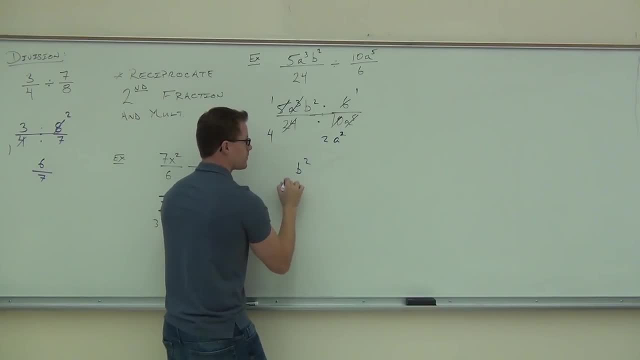 And what I'm hoping is that you've got a b squared over 8 a squared. Did you get that as well? And we're done As far as you can go. We're done on that problem. okay. Now let's see what happens. 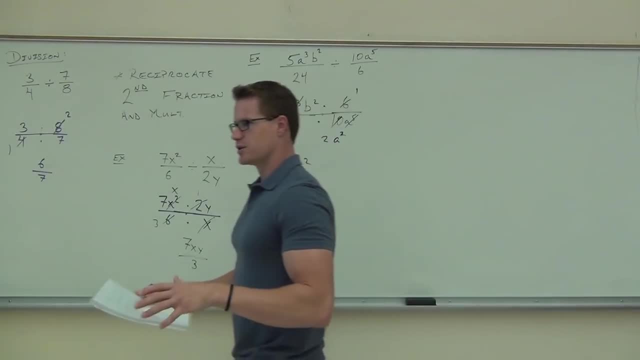 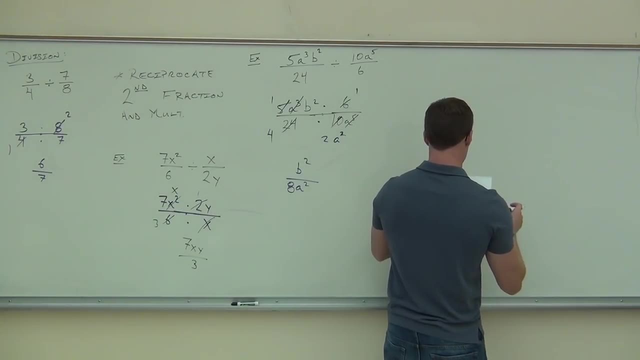 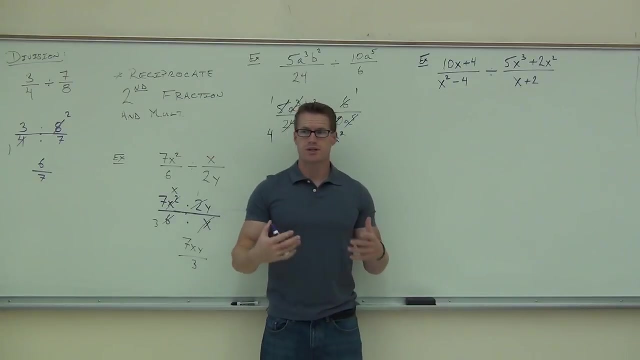 See if we even do anything different when we start getting actual, honest to goodness rational expressions. So this has some pretty serious factoring in it. We're going to have to do that, But here's what I'd like from you, all right. 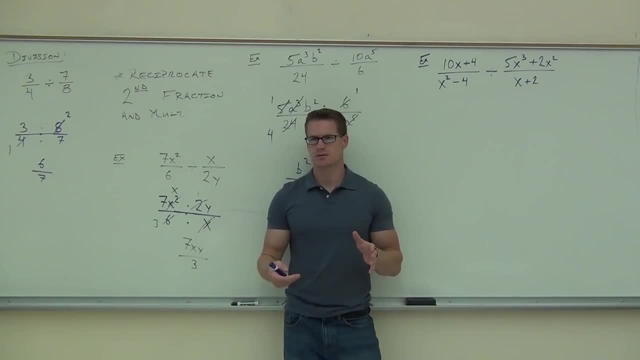 You all know that we're going to factor here, right, Right, You're going to factor eventually. That's what this whole thing is. That's what this whole thing is about. Just make sure that you flip it first before you factor it. 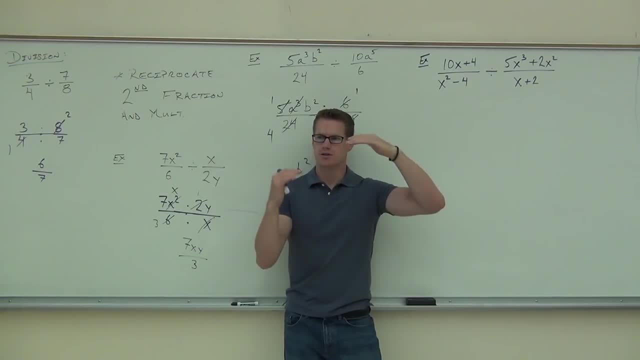 Because what I would hate for you to do is factor and then notice some common factors that maybe are coincidental and simplify those before you flip it. That would be the wrong thing. So make sure that we're flipping this first, And then you can start factoring. 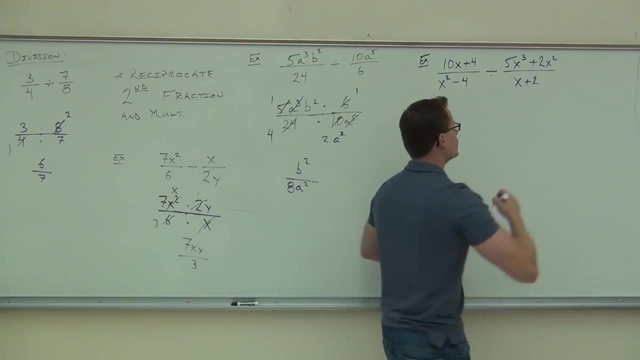 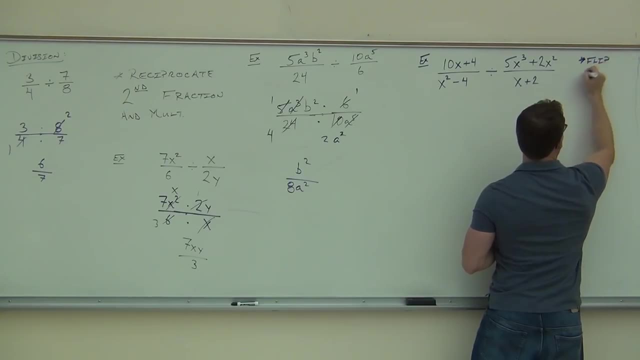 Are you with me on this? Just do that first when we have that down. So I'll say: flip first, then factor. So the first thing we're going to do, we'll leave the first fraction alone. We all know that by this point. 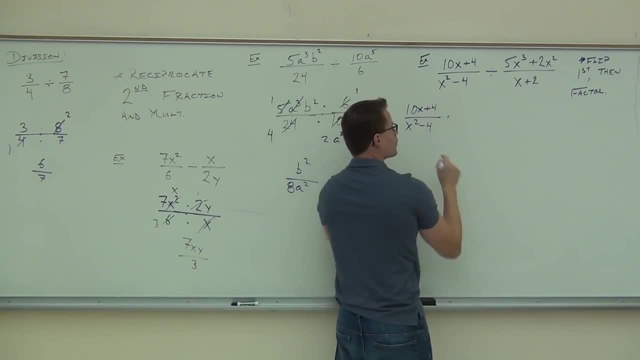 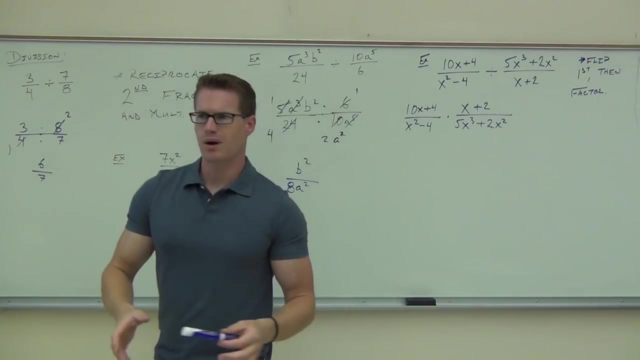 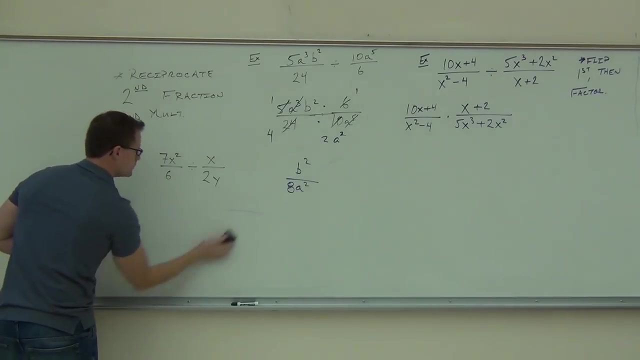 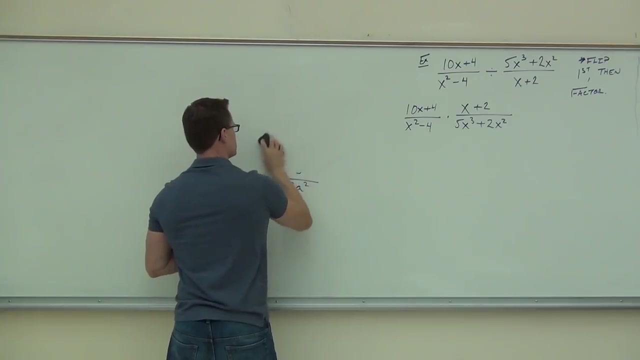 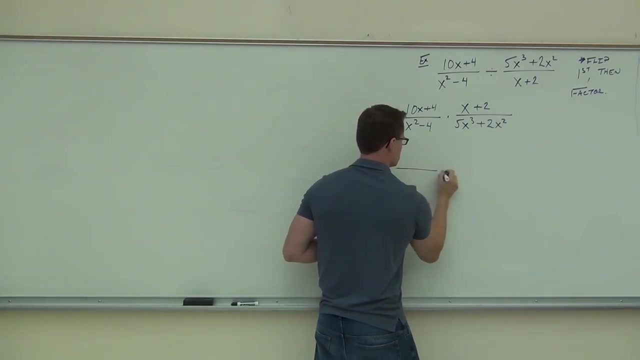 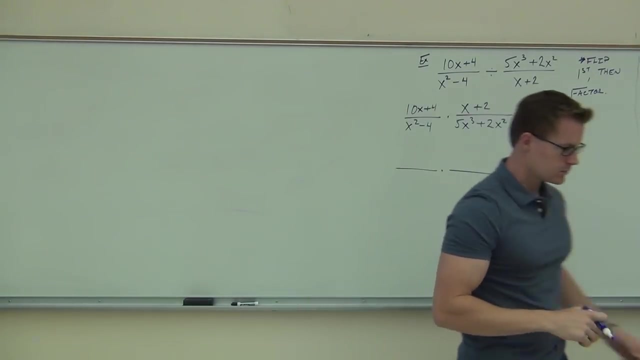 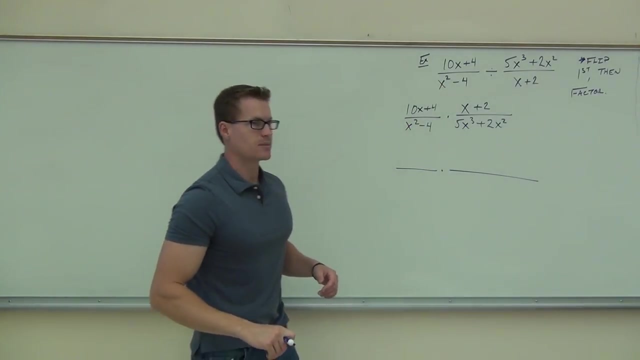 We're going to change our division to multiplication by reciprocating the second fraction And then we get to factor it. Why don't you give yourself some time, Give yourself a few seconds to try to factor that thing, okay? Okay, let's start doing it together. 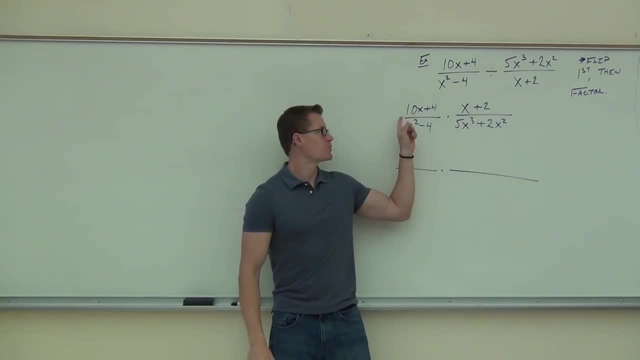 If you're still working on it, that's fine. Top fraction or top numerator here. What's this? one? Two, Two, Two goes out of that. okay, Two goes out of that. we get what? Five x plus two. 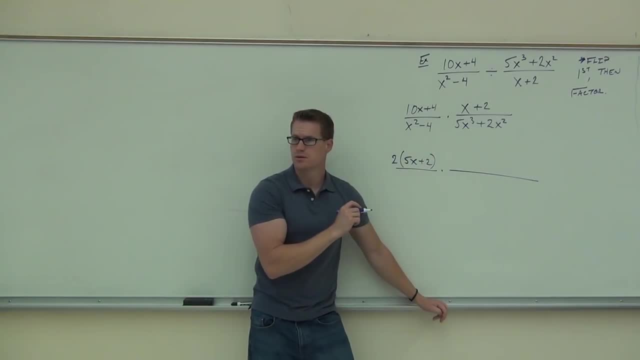 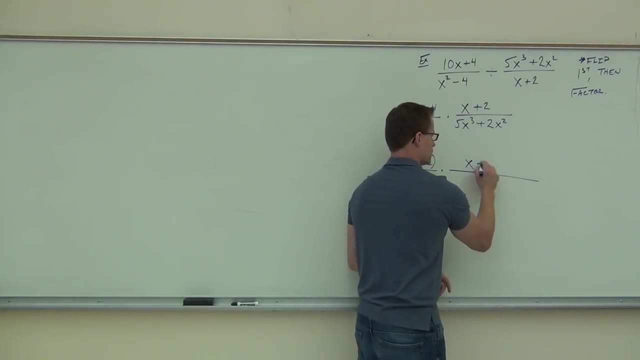 Good, Did you all get five x plus two? Okay, How about this numerator? What factors out of these two? The same? Okay, great, Sometimes that happens. How about this one? Does anything factor out of those two? Good, 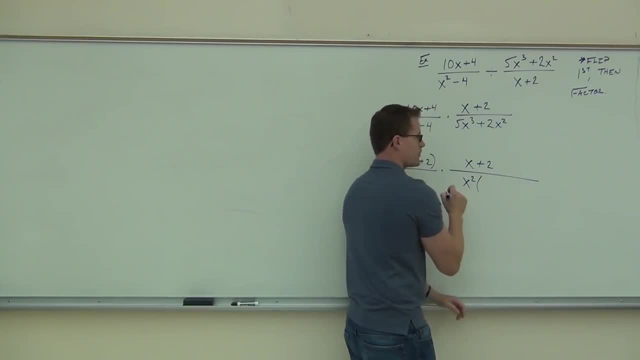 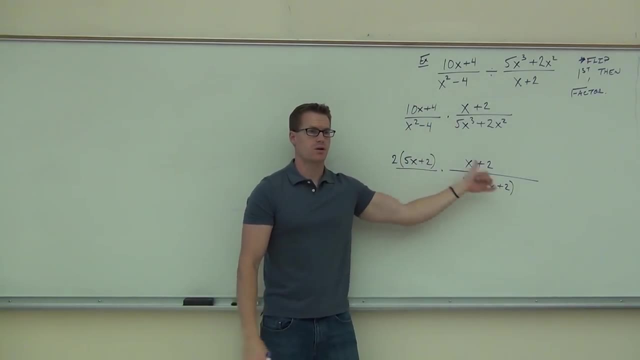 Good, And I'm left with Five x plus two. Okay, We already might be seeing some things here, right? That's great. Now, last one we have is x squared minus two. Okay, So x squared minus four. some of the right-hand side of the room. 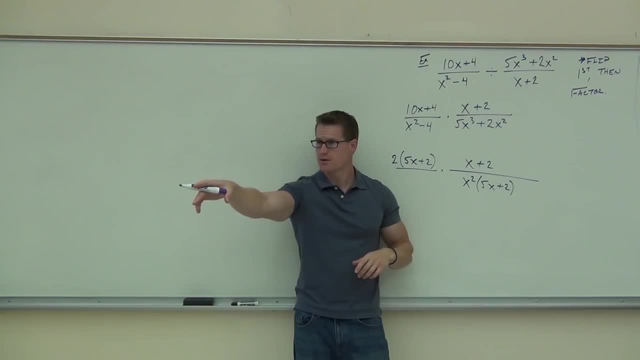 What is that known as X squared minus four? Difference of squares. Say it louder: Difference of squares, Good, Difference of squares. And some over here. how does difference of squares factor in this particular case? Good, Two right. 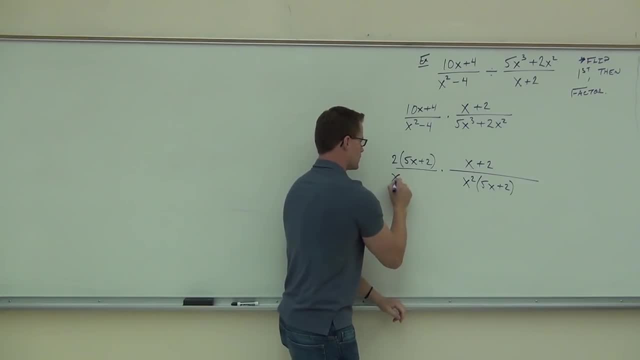 Not four, two Good. Are you starting to see the difference of squares a little bit easier? All right, I'm throwing them at you now. I'm just making sure you get this down. We've had like three or four today. 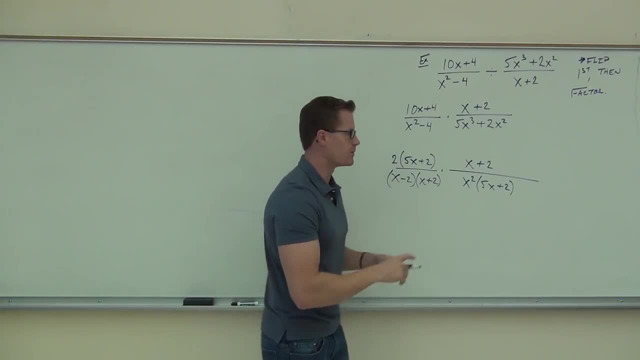 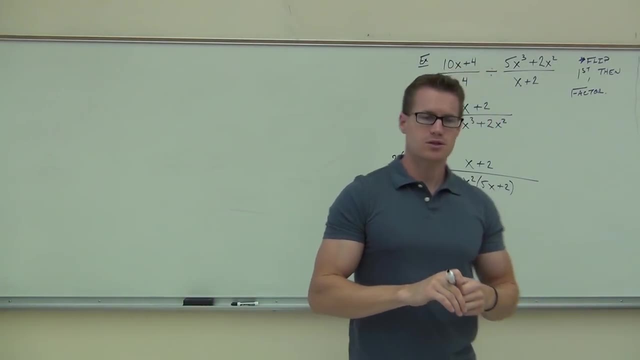 So we really need to get those, so we're not really stuck on them. That's why- Okay, great, We have this thing completely factored. The next step is to do what Good? Okay, let's try that. So one big fraction out of this. 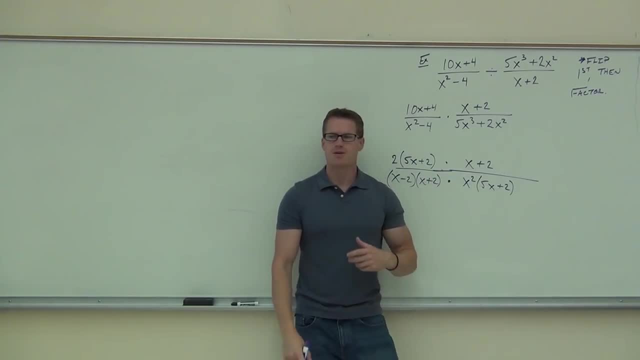 That's what I want to see. There's one thing here I need you to notice: If you make this one big fraction here, notice you're multiplying right. And this top thing, it didn't have any parentheses We could factor. 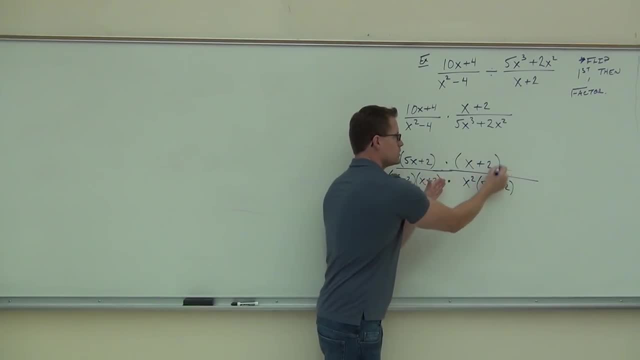 We didn't create any parentheses. But if you're going to multiply this, you do need to throw some parentheses around that. Do you see why? Multiplying that out, Multiplying that entire thing, This fraction implies parentheses here and here already. 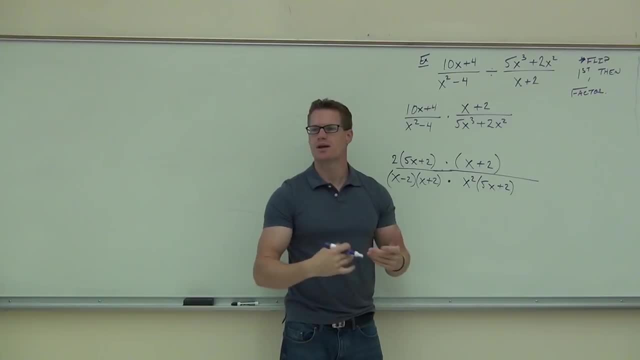 So we need to show that on the next step when we extend that fraction. So make sure you have those parentheses. That's going to allow you to simplify some things a little bit easier, because you're going to see it. Now that we see it, what are you guys seeing here? 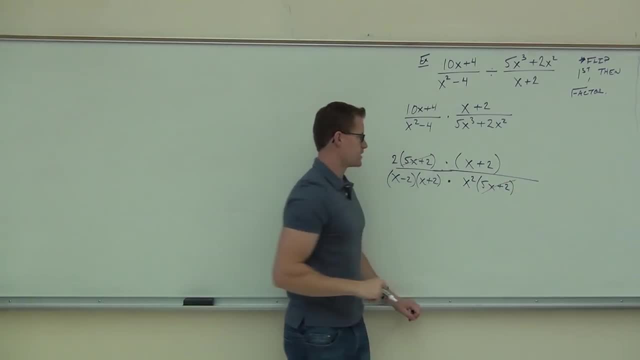 5x plus 2.. Okay, Somebody else give me another one besides: 5x plus 2. 2. 2. Okay, Someone else give me another one, if we have any. Do we have anything else? Okay, Let's write what's remaining. 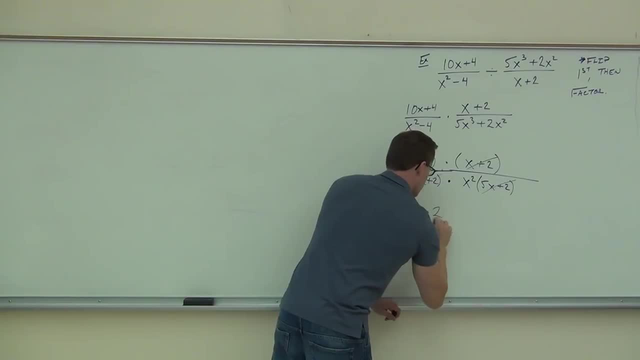 Only thing we have in the numerator is what 2.. 2. On the denominator, I see the x minus 2.. We didn't cross that out. I see the x squared. Be careful not to lose that thing. We typically will do it this way though. 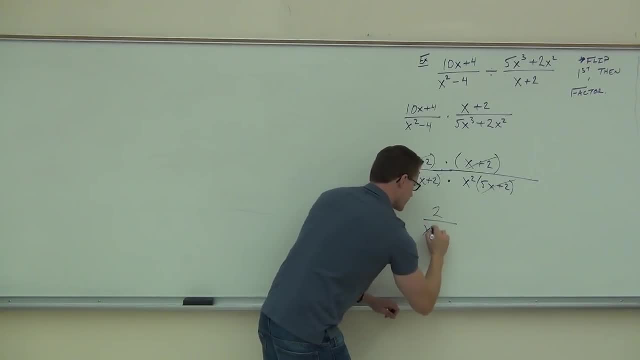 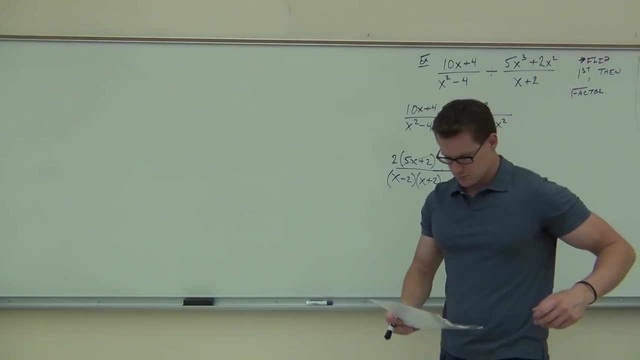 We'll write the x squared before the parentheses. Don't distribute it. You're done. That's as far as you can go. Do you feel okay about this example? No, Right, I'm going to have you do one on your own before we do another one together. 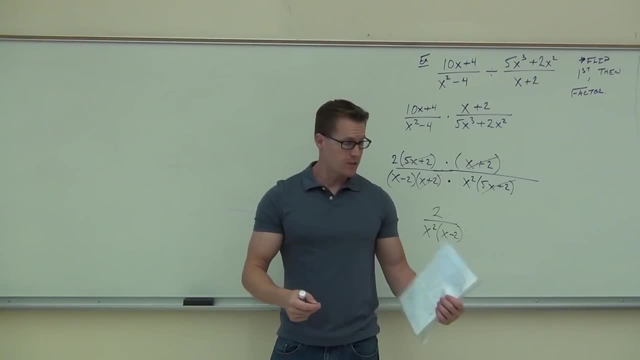 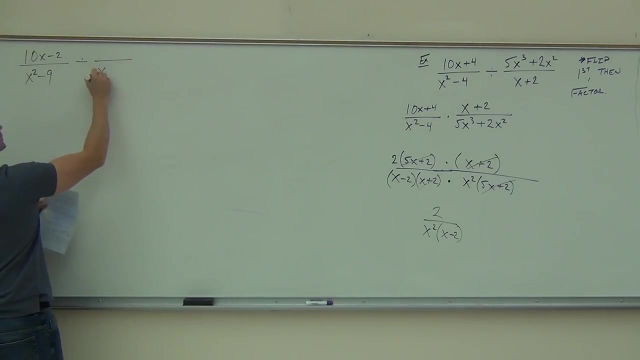 Then we'll practice one more, and then we should have some time, And then, when we're done with our section, we'll go on to adding and subtracting. So try this one completely on your own. Okay, It is similar. Here's the last one, which is good. 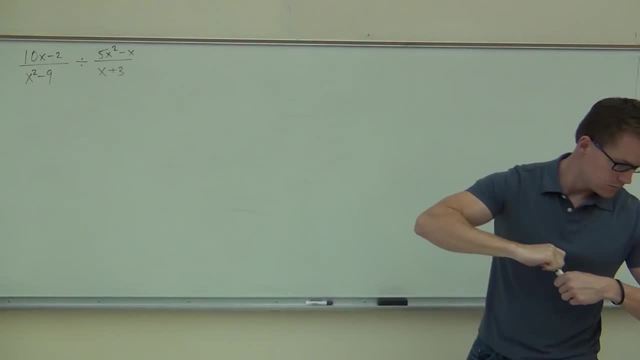 3 Degrees, twice greater than half. That's correct. I got this, See, And then it goes. Sometimes you have to mix all the missing str感謝 at the end. So how many operations does 1 pass 8.? 8,, 9,, 10,, 11., 12., 7., 5., 16., 8., 12., 14., 16., 17., 18., 19., 19. 20.. 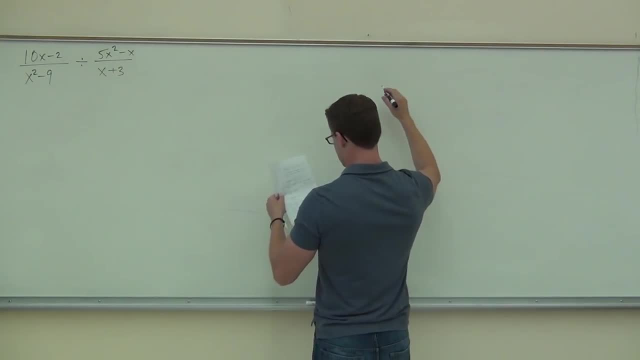 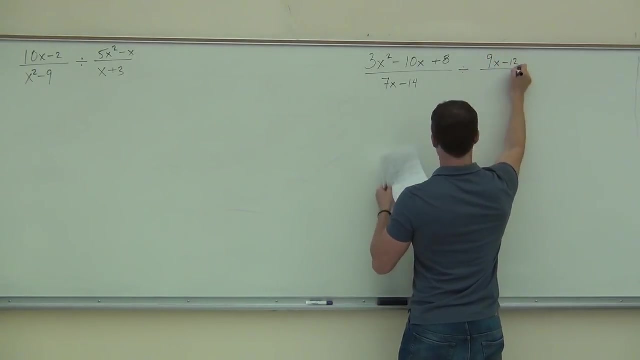 21., 22., 23., 24., 25., 24., 25., 26., 27., 28., 29., 30., 31., 31., 32., 34.. Do this one on your own. 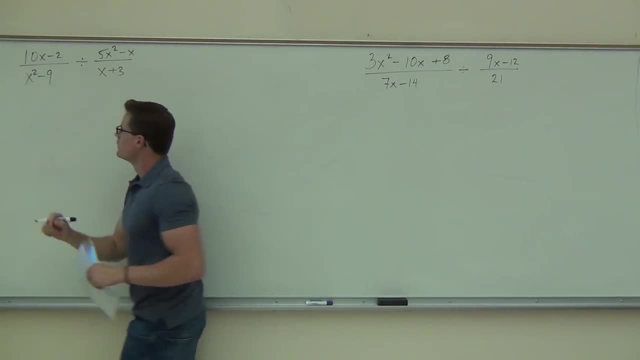 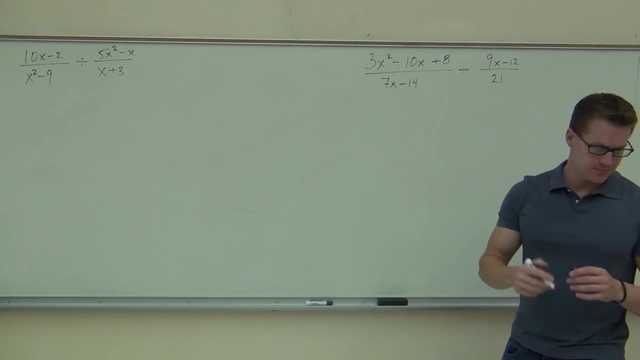 If you get done with that, that's a 10. by the way You get done with that one, you feel like a superstar. today you're like a rock star, you know. go ahead and try that one. By the way, is there any other homework to turn in that you've had to give in class? 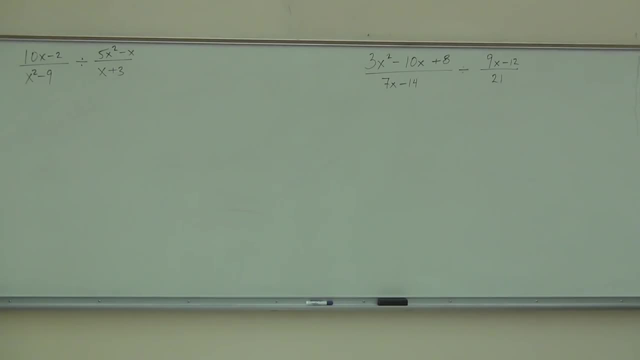 Is that the first assignment you're going to write? Are there two assignments in there? Did you get jumbled? I mean there should be four steps going on. Okay, make sure the steps are separate when you go in, because people are going to forget. 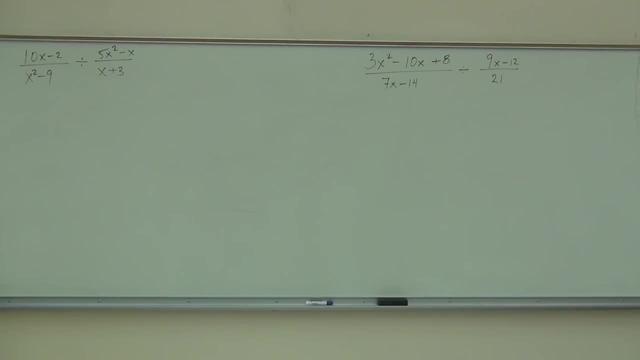 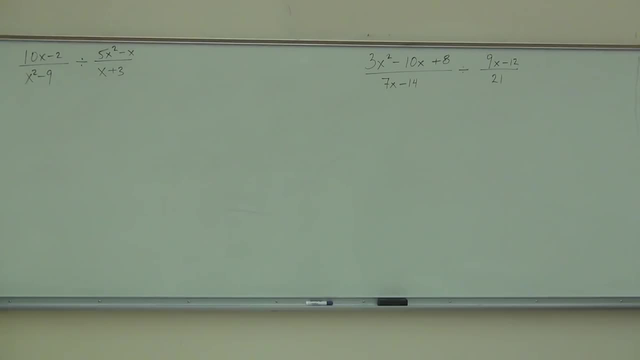 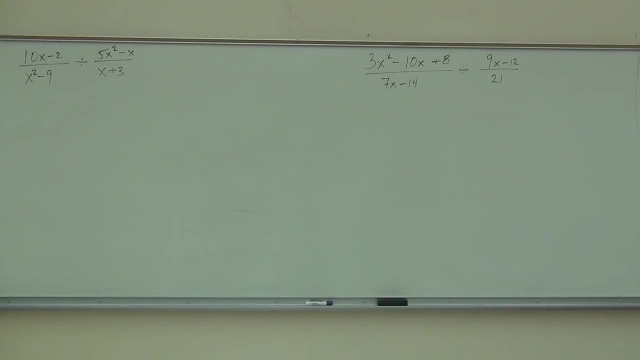 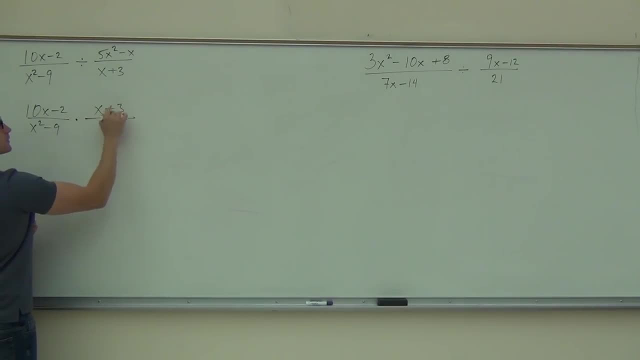 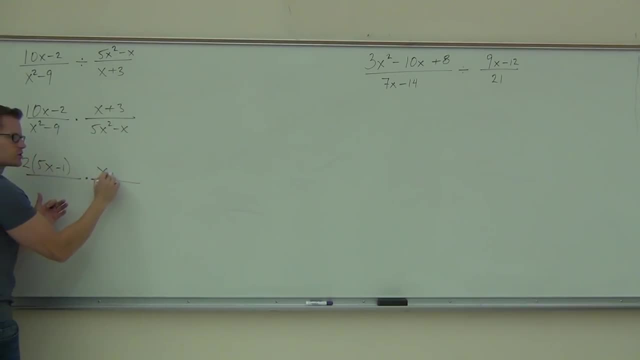 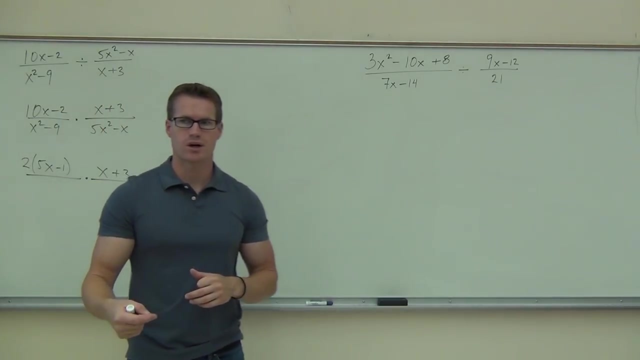 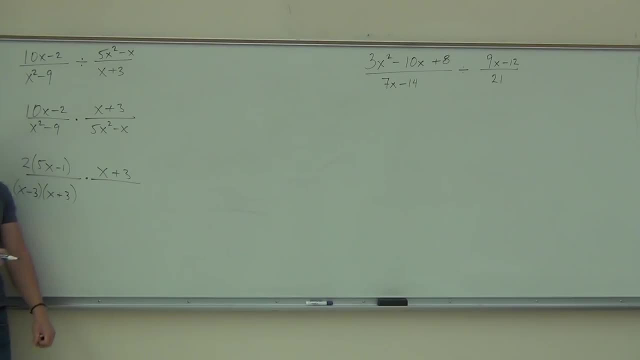 Okay, Okay, Okay. Okay. we factor out is just an x and we're going to get 5x minus 1.. Before we go any further, before you start simplifying anything, crossing stuff out, even though I know we want to do- 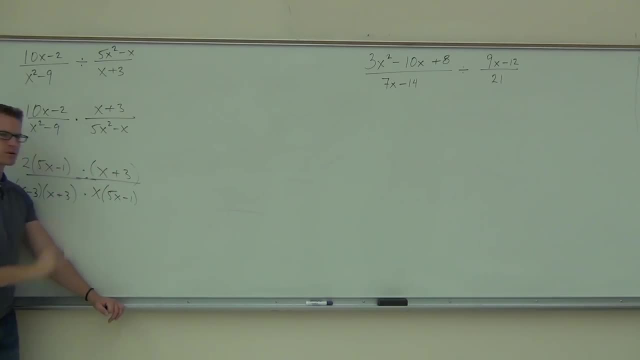 it right here. just extend this line, put the dot and the dot. We need some parentheses around that thing, and now we're going to start simplifying. What I see up here is an x plus 3 and an x plus 3.. I also see a 5x minus 1 and a 5x minus 1.. I just don't want. 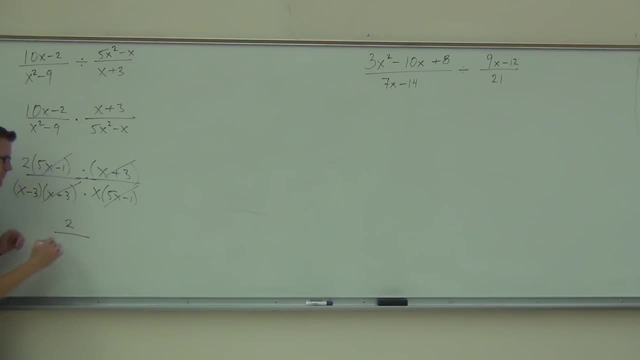 to forget the things that I haven't crossed out, such as the 2, that x particularly. A lot of people forget that x. We don't want to do that. The x we're going to write first and then we'll have x minus 3.. Would you raise your hand if you made it down that far? That's. 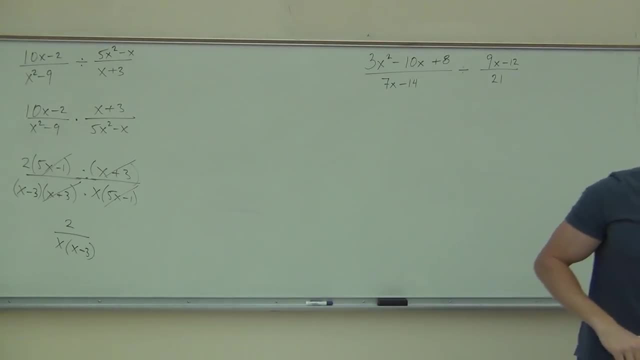 good, Good for you. Now the next thing we're going to do this one very similar idea. It just has a little bit more complicated factoring in it, but if you know how to factor these things, you're going to be able to do it. 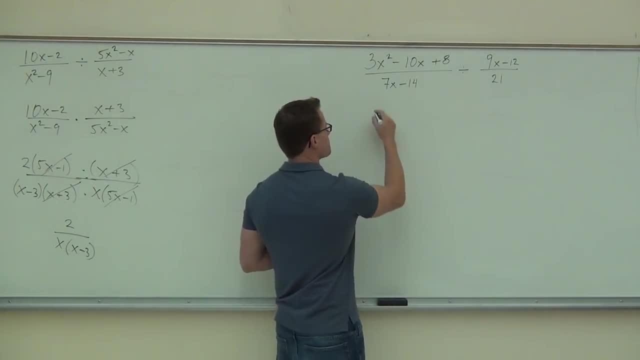 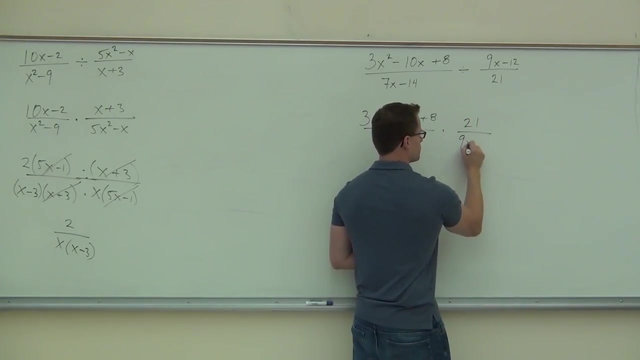 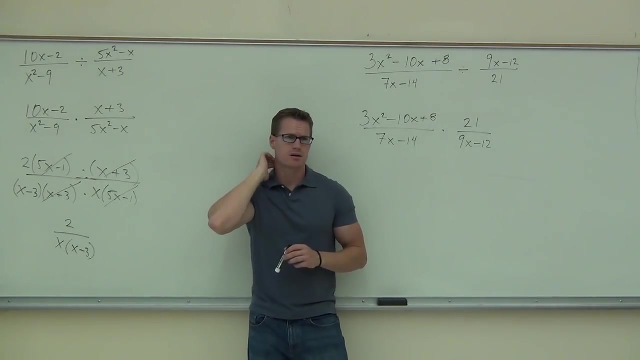 It's not a problem. So we're going to leave the first fraction alone. We are going to reciprocate the second. Tell me something up here that you need to factor. Would you tell me that? Yeah, We are going to factor. 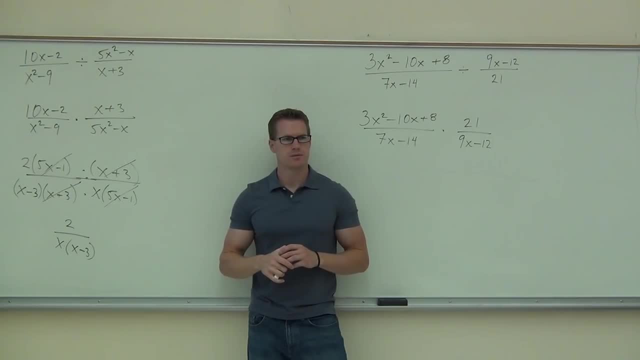 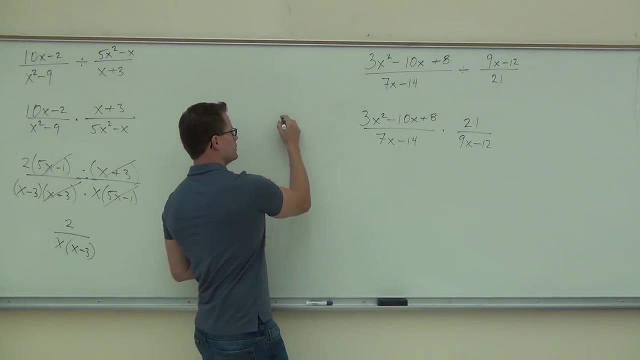 We're going to factor that. How do you factor that problem? Okay, Does this have the extra step or not? do you think Absolutely? So we're going to factor that. This is probably the hardest thing to factor in this problem. 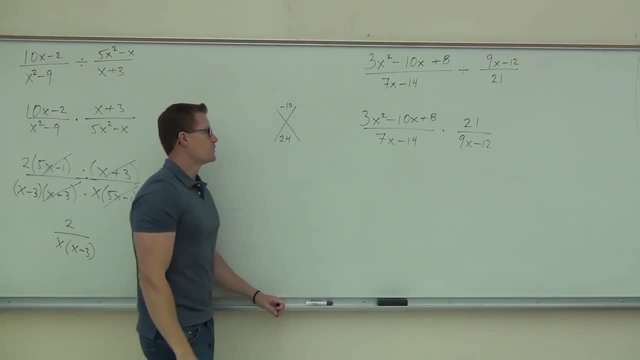 You've got negative 10, we've got 24.. One of the things I'm thinking is: negative 10 and 24 are like 12 and 2.. Or am I wrong? Okay, You could do 12 and 2, right, but it's not going to work out. to add to that, You can't. 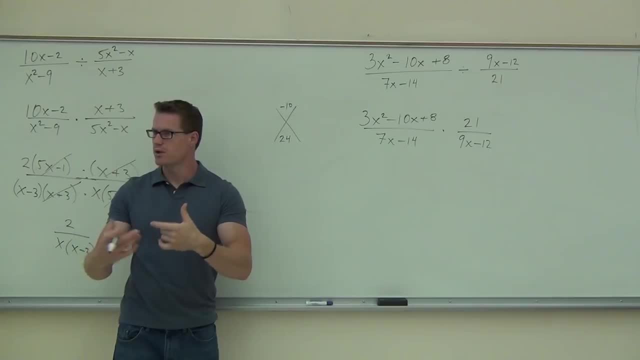 do it, So we're going to factor that. So you're going to have to have two negatives here that multiply the positive 24 and add a negative 10.. So don't trick yourself up on doing stuff like 12 and 2.. Even though 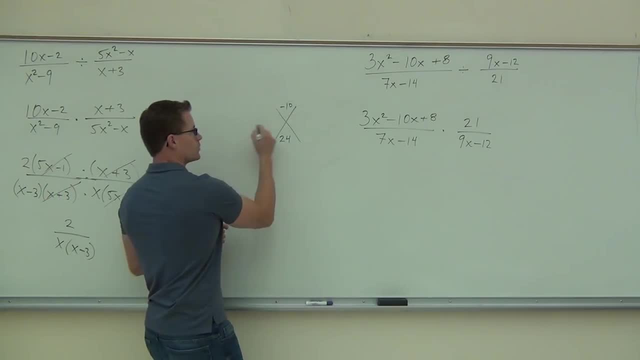 those are the first numbers that popped in my head. you really do have to check. So negative 6, negative 4.. We're going to write 3x squared minus 6x minus 4x plus 8. So we're getting. 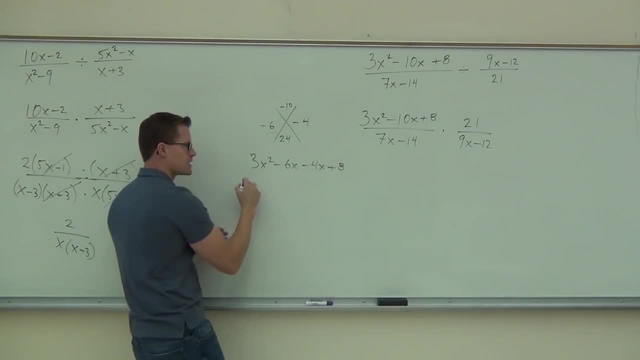 that from over there, just like we've done several times before, Factoring by grouping says we're going to factor out 3x. We're going to factor out a negative 4, which is going to change the signs inside of our parentheses. on the second part of this thing, We have 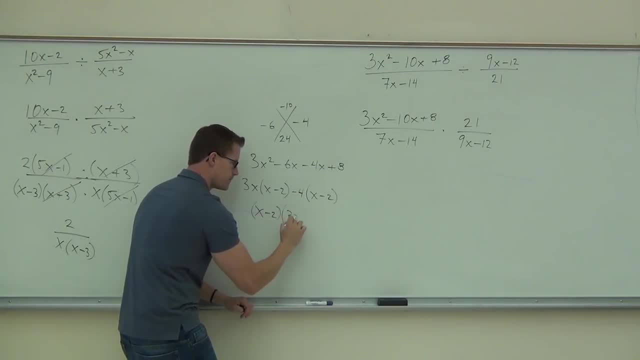 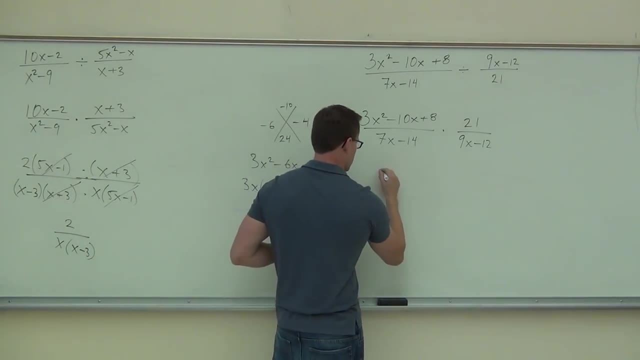 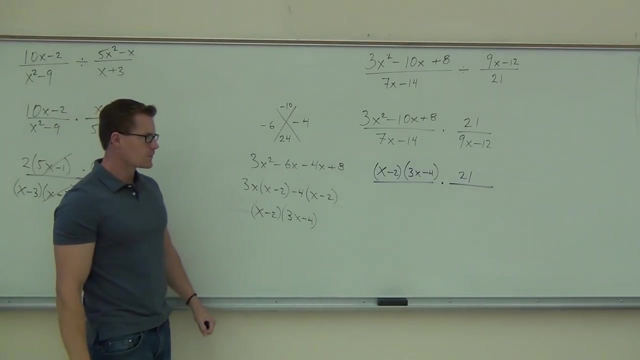 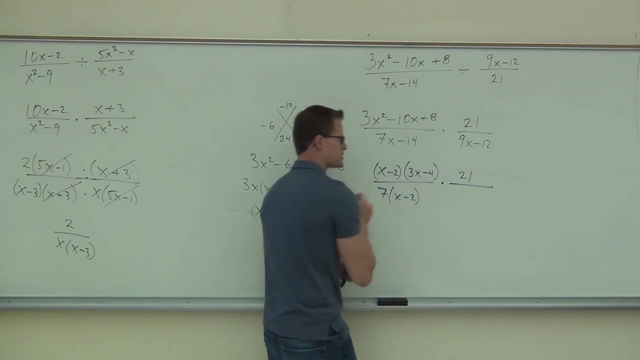 done it right. We'll continue to factor that And that. right. there is our new numerator. I know 21 doesn't factor, but the other two should factor. What factors out of my 7x minus 14?? So we're going to get x minus 2.. The other thing we're 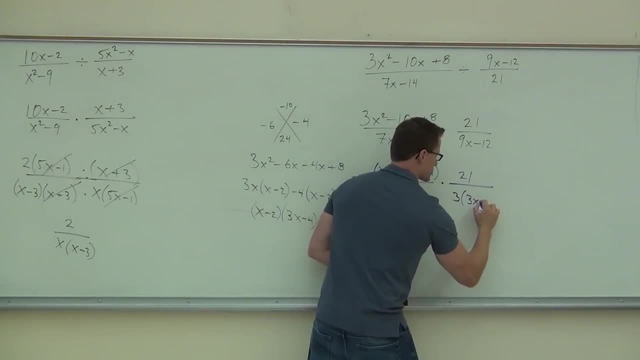 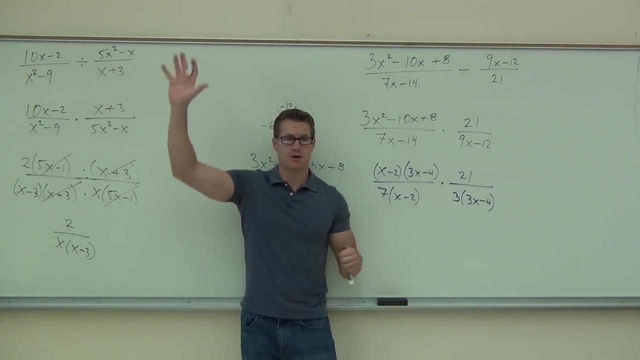 going to factor out is a 3.. We'll get 3x minus 4.. And now we're going to start the good part of simplifying some common factors. By the way, how many people were able to make it down that far? I know we gave some time on that. Oh, that's fantastic. Very good, We'll. 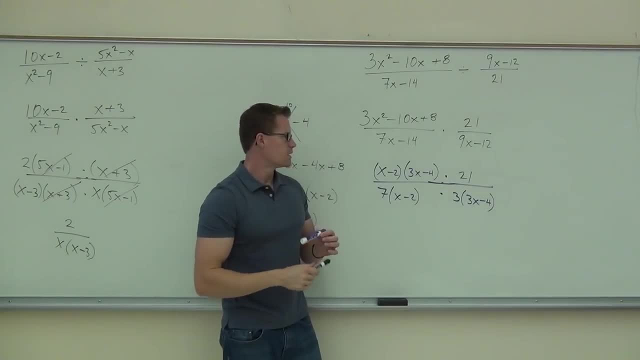 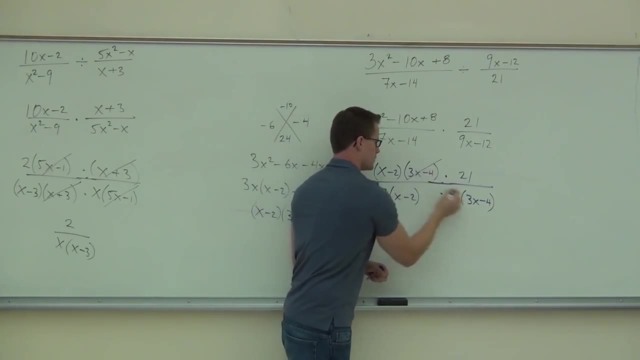 extend our line. put the dot dot. Can you tell me something up here that simplifies Good. Do you remember any other things? That was broken, Yeah, that was broken. What else do we have here? 9. 9 times 7.. 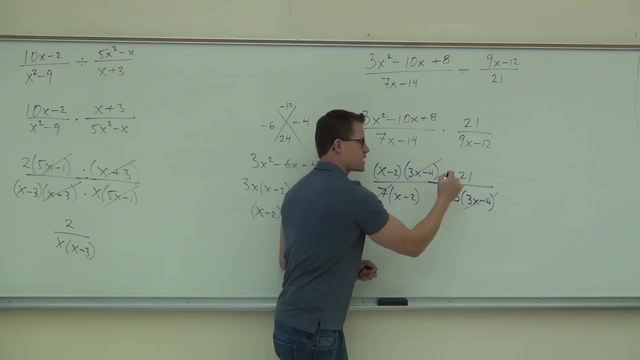 9 times 7.. 9 times 7.. When does 7 become a 3?? 7 becomes a 3.. 7 becomes a 3? You can go over that. Yeah, 7 becomes a 3.. 7 becomes a 1.. 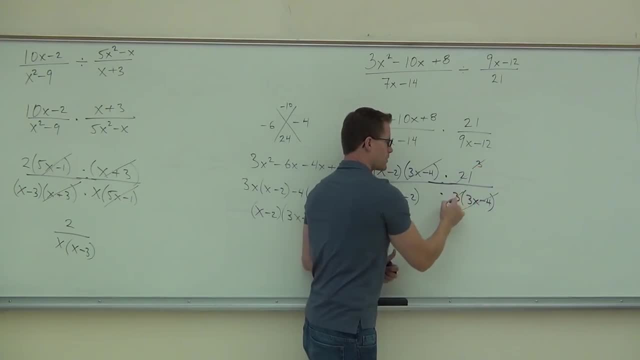 7 becomes a 1.. 7 becomes a 1.. What else? 3 plus 3.. Yeah, The 3 is there. You can keep going on that We have a common factor of 3. still, 3 plus 3.. Anything else? 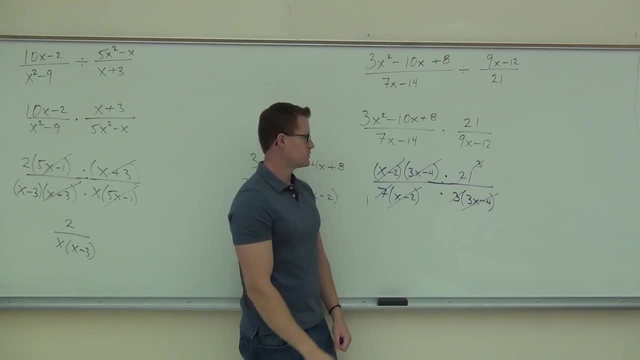 That's minus 2.. Wait a second. We just crossed out everything. You got 1 and 1.. We don't have 0.. We don't have 0.. What you have here here is the first two. That's 1 plus 2.. 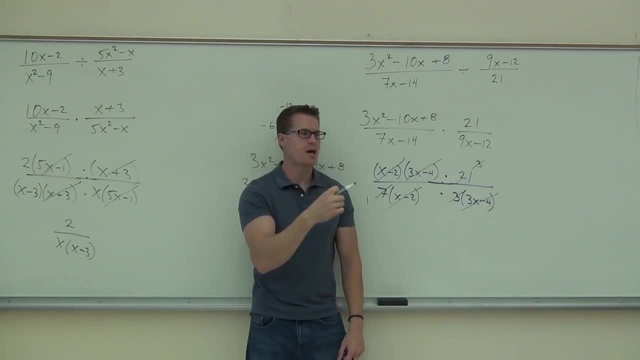 What you have here are you made lots of factors of 1, right. So basically you have 1 times 1 times 1.. That's just going to make 1 for us. You have 1s on the top, You have 1s on the denominator. 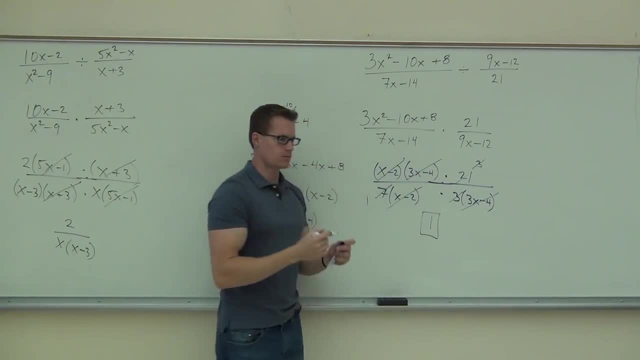 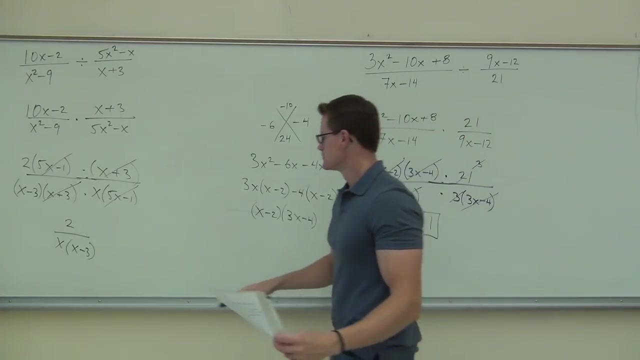 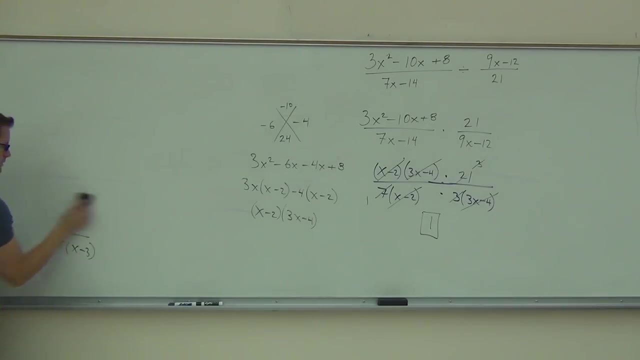 You're going to get 1.. Okay, I want you to do 1 all the way down by yourself, and then we'll call it a day today. Well, maybe not. You might have something. Oh, but there are some homework problems. I do want to go over with you, so we'll do that. 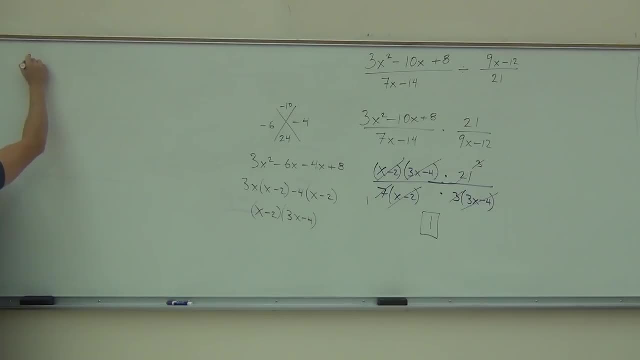 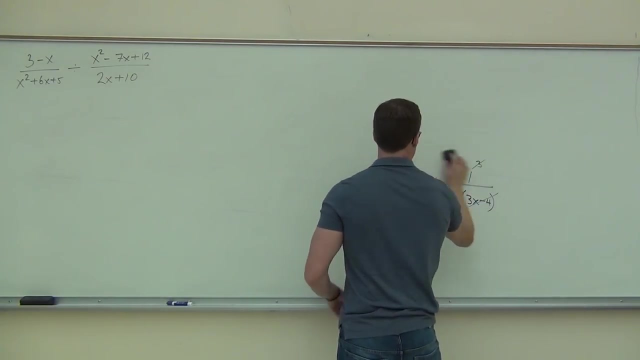 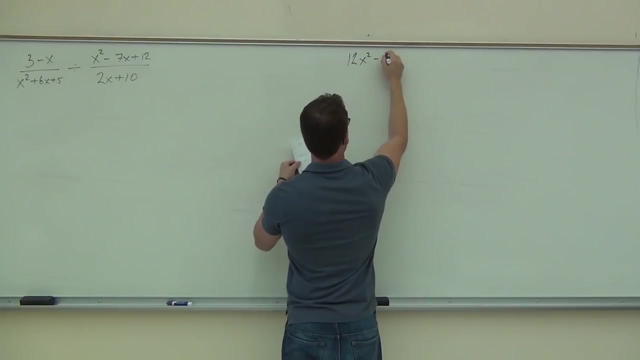 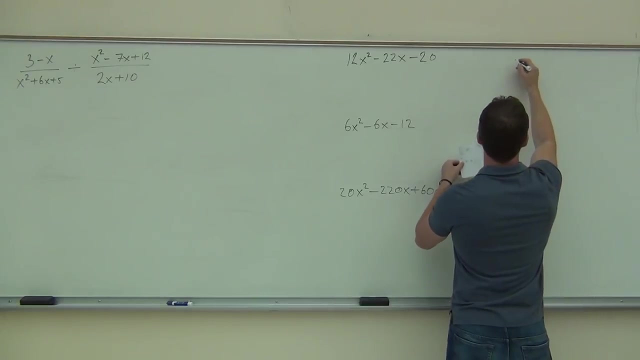 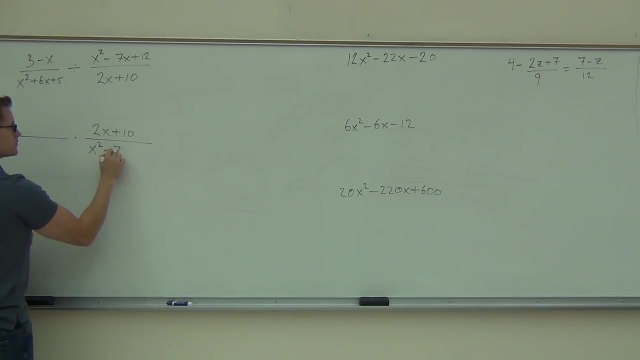 Hello, There you go. This is all you. You guys got to do this one. Oh, All right, Thank you, Thank you, Thank you. So I hope you reciprocated the second fraction. That's the first thing that you do. 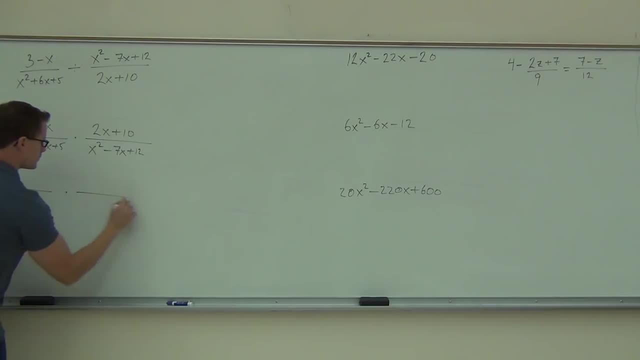 Next thing you do is a whole bunch of factoring. One thing real quick. I want to make sure you saw this. Look at the board here for a second. I'm going to pause you On this right here. even though it looks like well, there's no common factors. 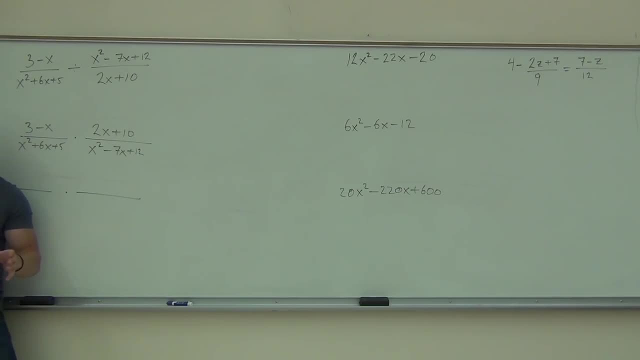 what I need you to do with this thing is make the x term positive. Remember doing that, So make that positive. That means you're going to factor out a negative 1 here and you're going to get instead of 3 minus x. 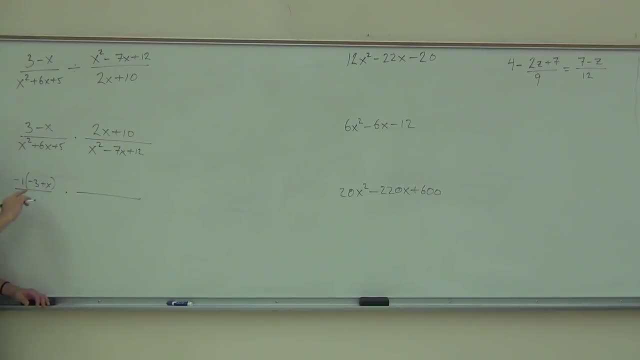 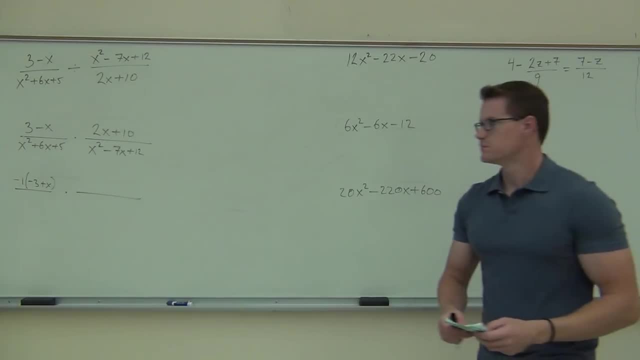 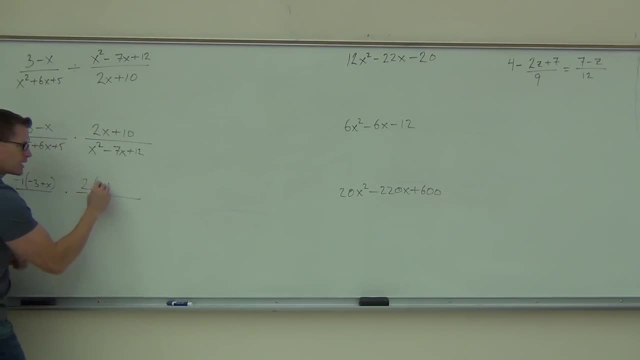 We have 2x minus 10.. Hopefully you factor out 2 from that And you've got x plus 5, and you've got that one. Hey, these last two, they're clearly diamond problems. We got three terms. 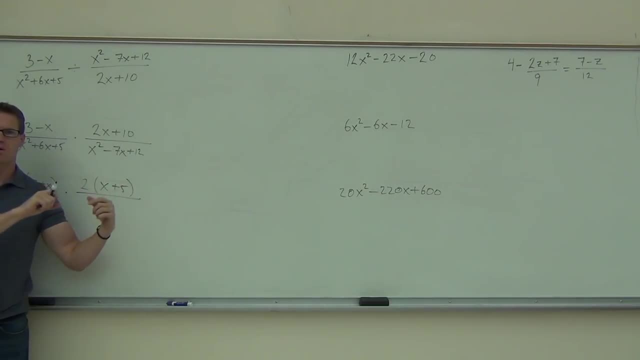 Am I going to have to use the factor by grouping that extra step, or can I go directly to the factors? Great, Okay, So these are easier ones, right? These are the ones that you don't want to waste your time on. 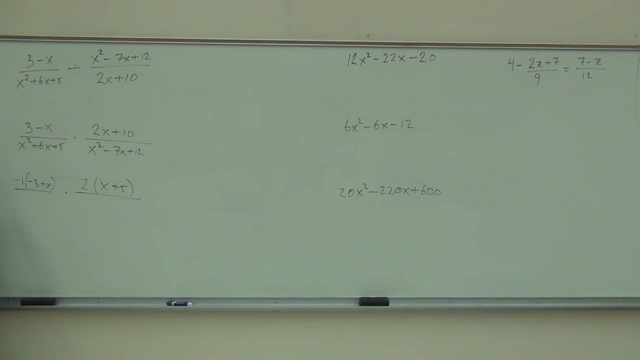 I don't know if you're going to be able to see this that well, but I'm going to do a mini diamond problem. Six and five right there. I'm going to do negative seven and twelve right there With the six and the five. that's going to be five and one. 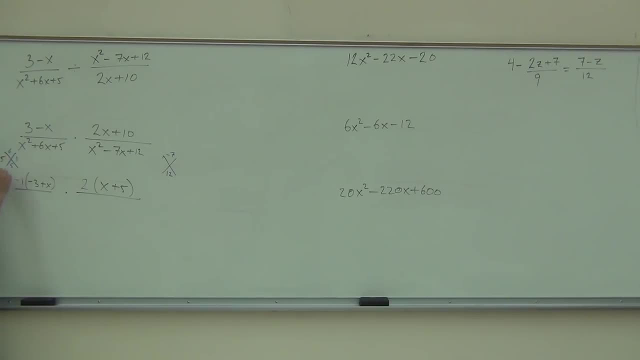 Did you get five and one, With the negative seven and twelve. that tells me I have two negative numbers here. That's going to be negative four and negative three. Did you get negative four and three? Yeah, Good, Okay, So here we have our x minus four, x minus three, no factor by grouping. 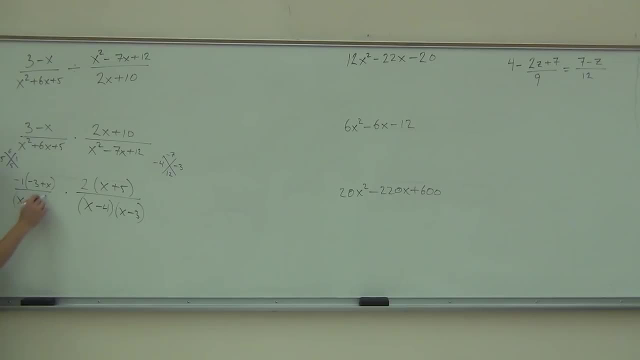 That's great. Here we've got our x plus five, x plus one Again, no factor by grouping, but you really shouldn't have to make it down that far. That's very good. Okay, So we extend our line here. 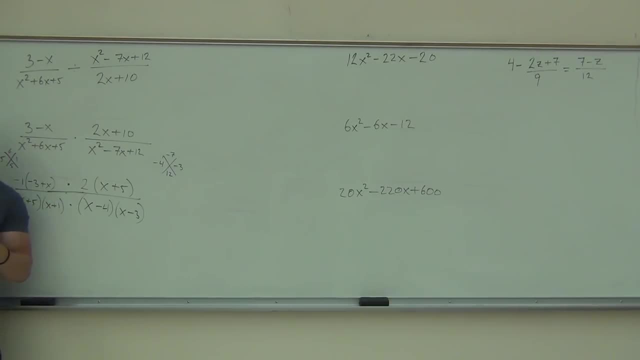 We put our dot and our dot. Now we can start simplifying some things. There's one thing I'm going to do before I do this, and you'll probably know what I'm talking about here. I'm just going to reorder these things because right now it doesn't look exactly the same. 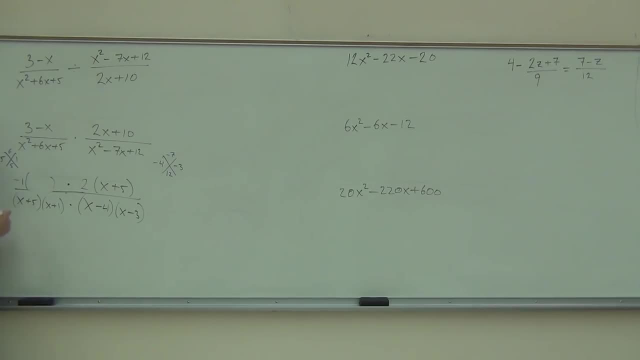 to me. So I'm going to erase this. I'm going to put my x minus three, and now I can simplify: We've got our x minus threes gone. We've got our x plus fives gone. Is there anything else that we can do? 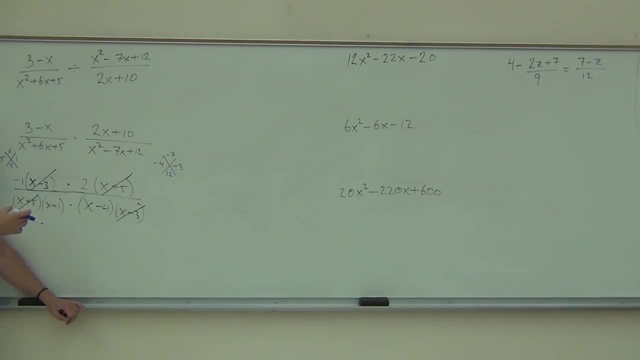 No, In fact there's not much left on the numerator. actually, What is left on the numerator for us? Negative one times two, So that'll give us negative two. And then on the denominator we have two factors left. We just have to write both of them. 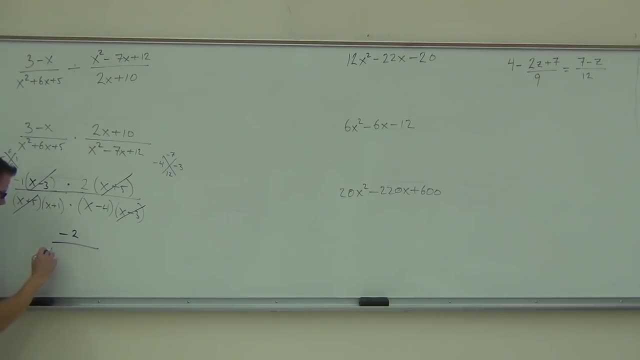 Don't distribute it, Don't coil it. That's it. That's as far as we can go. Ladies and gentlemen, we're done with division. How many of you feel okay about multiplication and division? Are you starting to see how important factoring is to us? 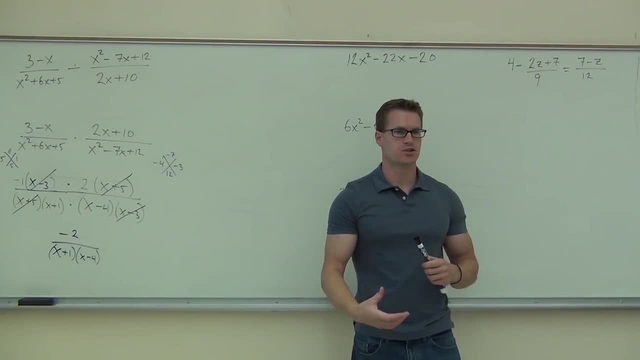 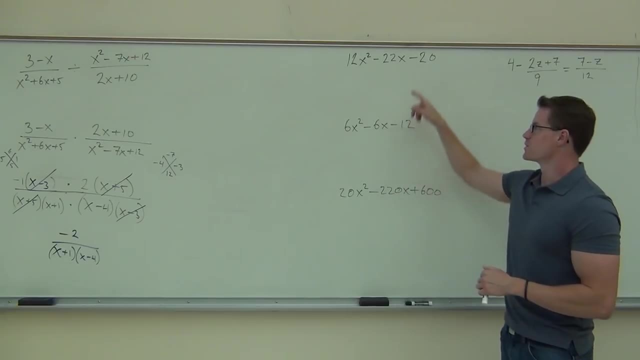 That's basically all we've done for like five sections in a row, just different applications of factoring to do in the last two minutes. I do want to go over these homework problems. These are from your C point, the first C, point four, I believe you did. 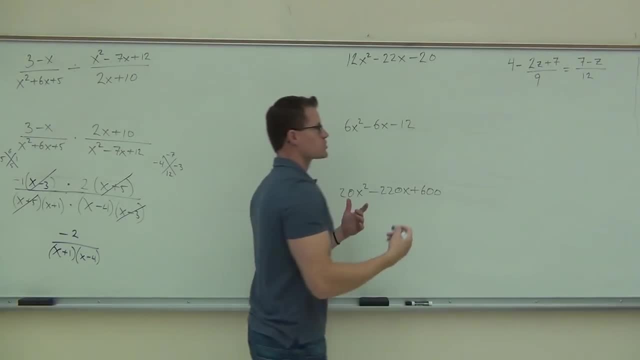 This one is from the solving, I think, C point one. I just want to make sure that you're seeing the greatest common factor. Look up how this is going to change what we do, especially on these two problems, if you factor your greatest common factor first. 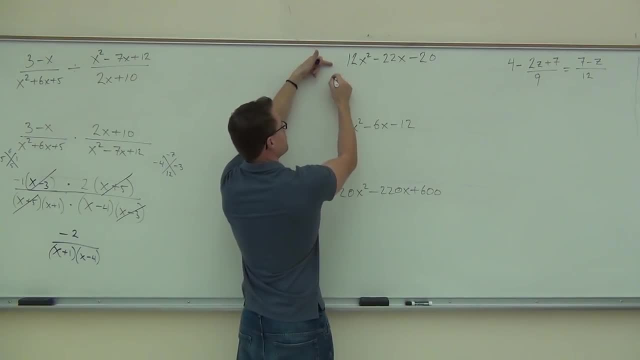 So, on this problem, we're looking at this. I know a two factors out of that, What this does for you. when you do this, it's going to factor it completely, because if you don't do this and you factor this with the diamond problem, the extra step which is 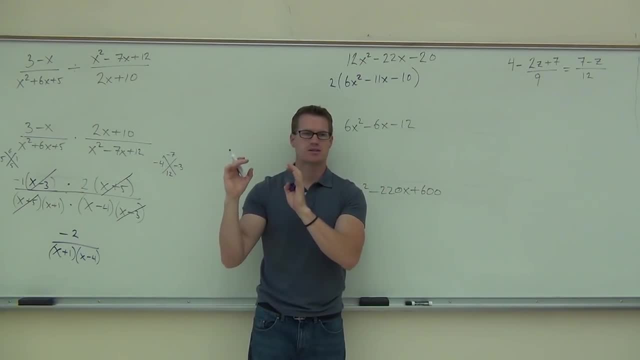 what you have to do. you're going to have one factor that still has something that can be factored. That's why, if I gave you the, if you said, oh, I did that right, I circled it, I crossed something out, that means you got it wrong, because it's not factored completely. 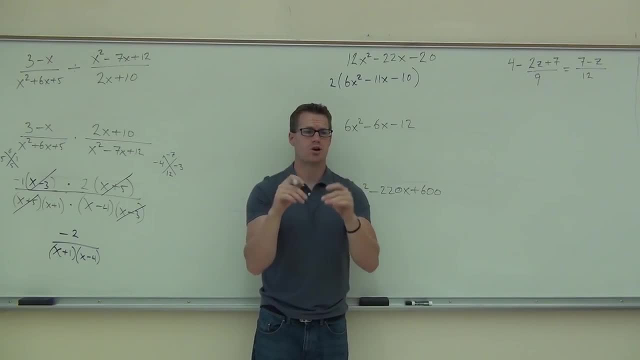 You have something in there that can still be factored. By the way, what I do on your homework, I circle one problem. I put a check mark. if it's right, I'll cross it out, if it's wrong, I'll subtract it. 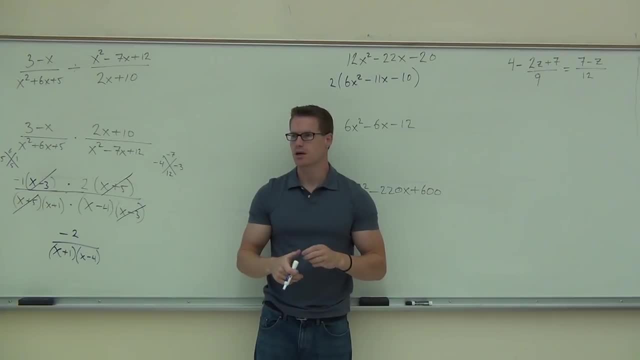 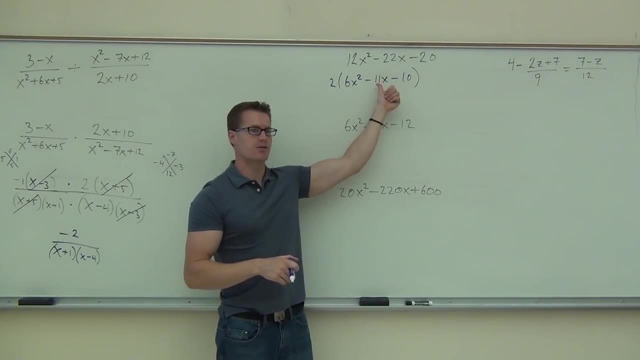 I'll probably circle the part that you need to work on if I have some time. So that's what you have on that thing. This would be the diamond problem, but you have to do this step first. You got it, Otherwise you're not going to have it completely factored. 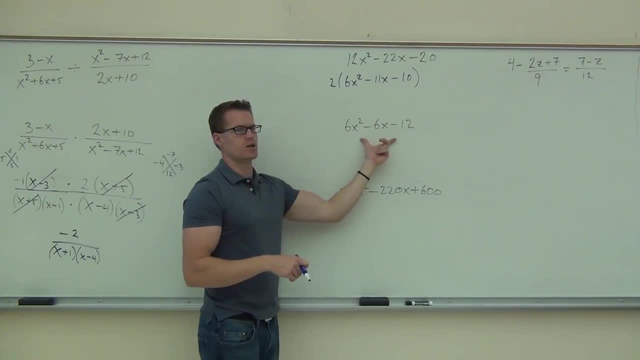 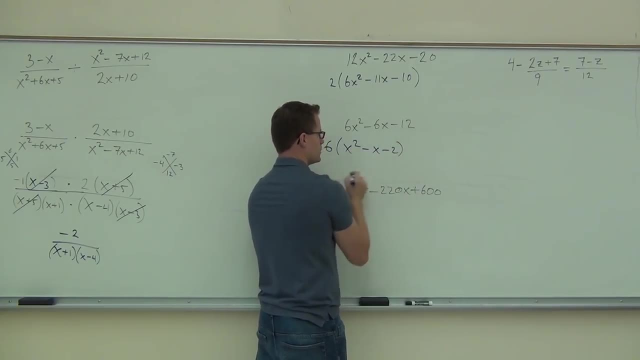 You're not going to be okay with that one. The next one: these ones are nice, Man. if you do GCF, you don't have to waste your time. You factor out a six. it becomes x squared minus x minus two. 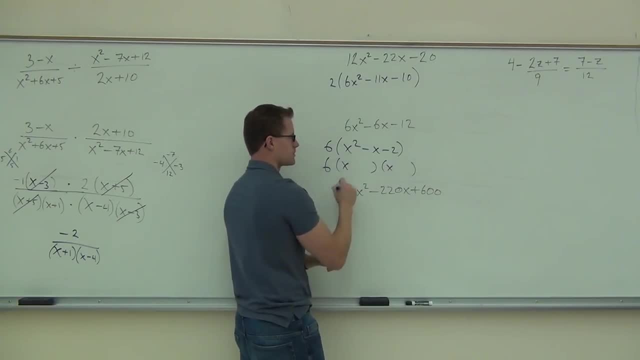 That thing factors very easily. That's x and x minus two plus one, You're done. You don't even have to do an extra step. That's just a simple diamond problem. off to the side. You with me on that. That saves you a lot of time. 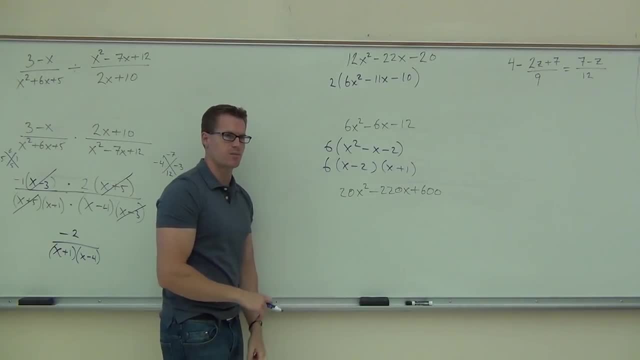 This one. this one saves you a ton of time. OMG, I mean crazy tight. If you factor out the 20 here, What is that 30?? This is one of the ones you might have spent a whole long time doing if you tried to do. 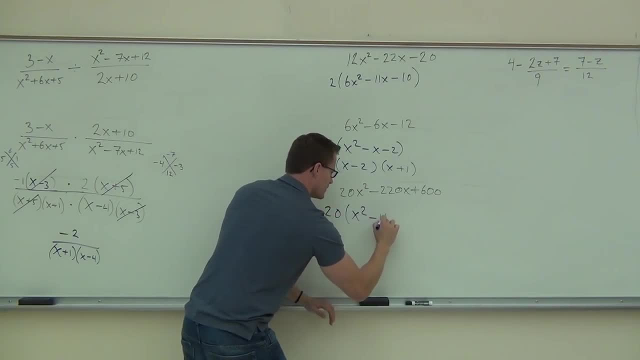 this with the diamond problem and the extra step. That's crazy. You get huge numbers. It's ridiculous. You get like 12 hundred, You get like 12 thousand. I mean, come on, Really, There's got to be a better way to do that. 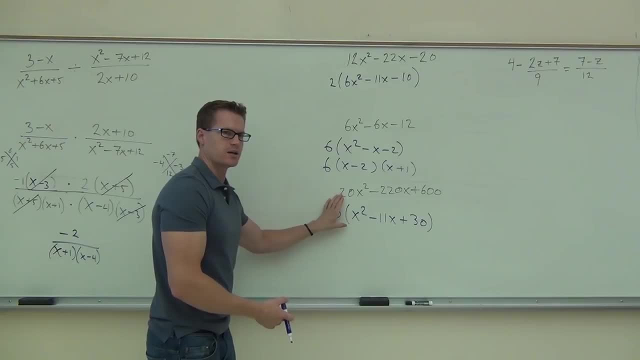 You factor the 20 out. Ignore the 20 for a second. Do you see that? this is very easy to factor? You just go 20.. That's a diamond problem. off to the side, Negative 11 and 30. You're going to get negative six and negative five. 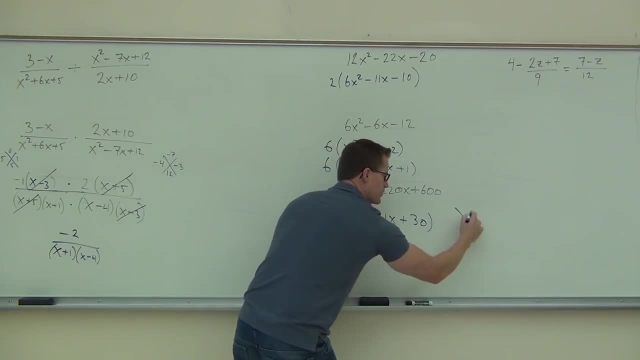 X minus six, X minus five. You're done. That's all you got to do This one. I just got to make sure you do one thing on this: When you multiply it by the LCD, which is on our left side, you're going to get negative. 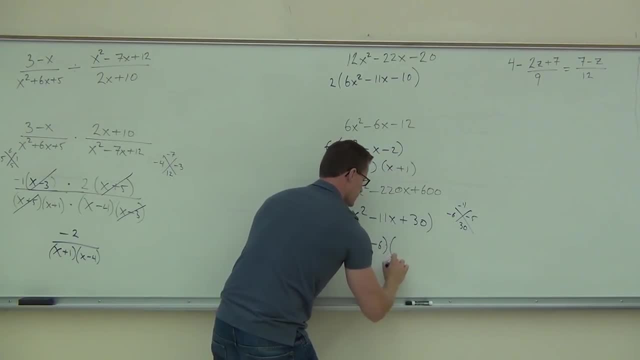 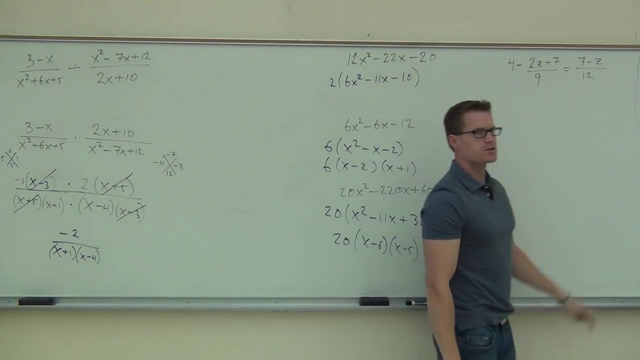 six and negative five. That's all you got to do This one. I just got to make sure you do one thing on this: When you multiply it by the LCD, which in our case is 36. Make sure you first multiply it by the four.